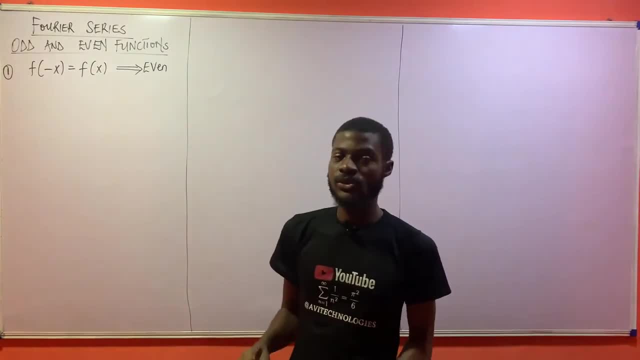 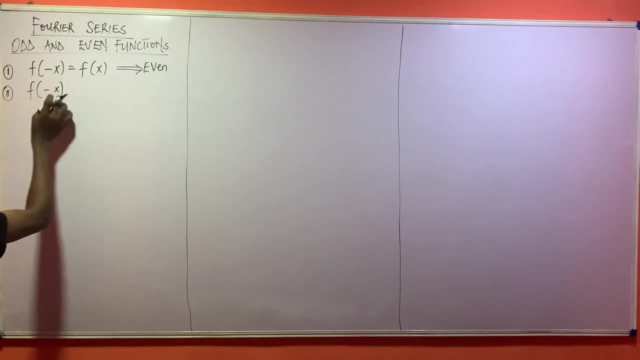 the same function as its own self. So this, if this happens, it's an even function. Okay, what if f of negative x? you still compute f of negative, but this time you get minus f of x. now what does this minus f of x mean? It means everything inside the function has changed its. sign. That's the meaning, because you know minus kind of changes signs. So if this happens, this can be called an odd function. So you can call the function an odd function simply because you now have the negative of the function. So let us get started here. Let us test something. 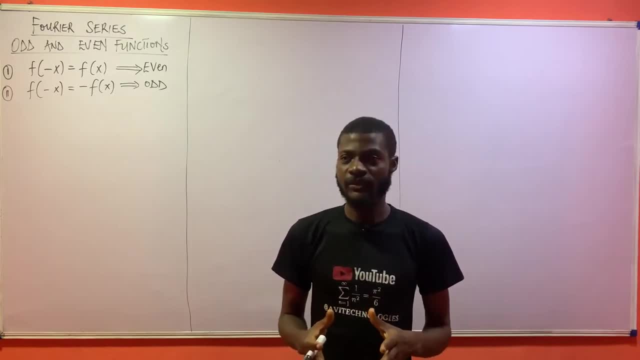 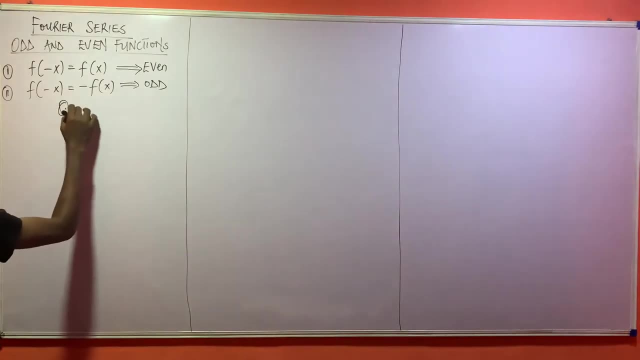 Let us test something First of all. you know Christmas around the corner. people are already disturbing me, Okay. so first question, First question. let us do this algebraically. So for a start, let us assume we have a function f of 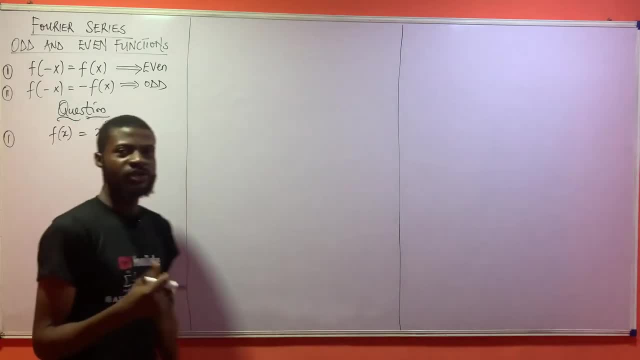 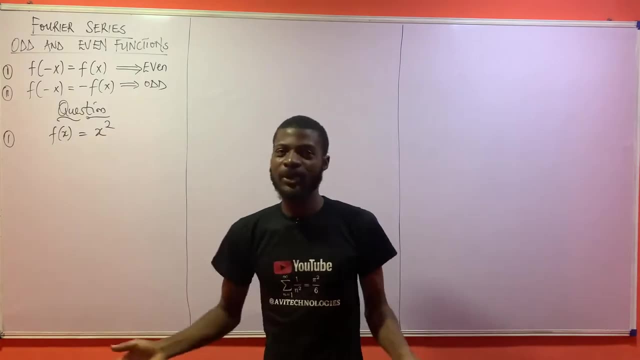 x equal to s squared. Now, is this function even or is it odd? Clearly it's going to be even. The power here is an even power. It is going to be even, but we don't just conclude like that. Let us just test it Now. what would be the value of f of minus x? 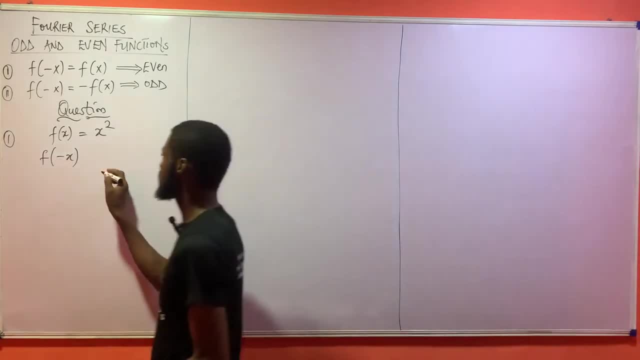 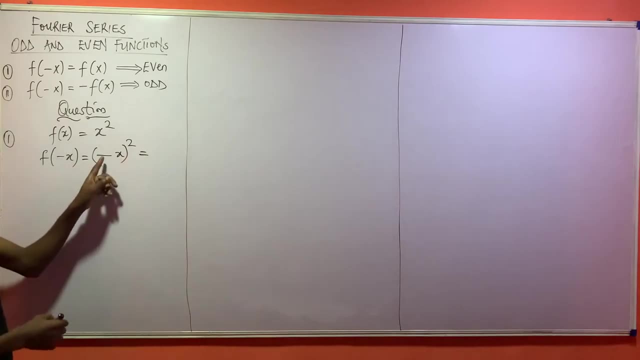 We're going to ask ourselves what would be the value of f of minus x? So this would then give us minus x all to the power of 2, right, Okay. so this would then give us minus s. squared means minus x times another minus x, right? So minus times minus is plus s, times s is what s squared. 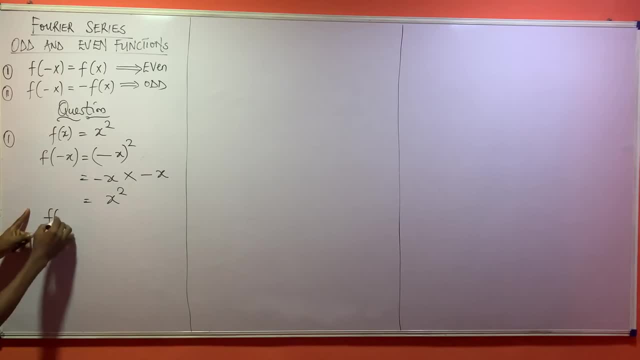 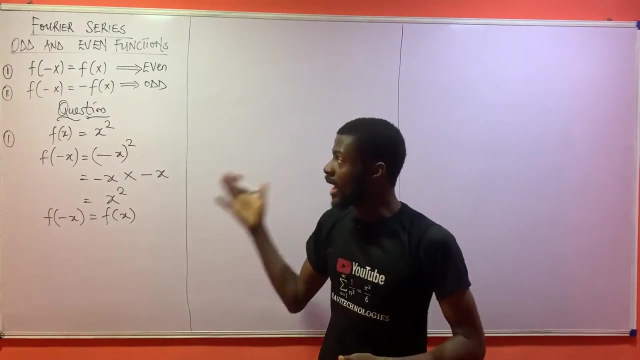 Now, what do you notice? The answer for f of negative s is the same thing as your f of s. So what does what condition does this satisfy? Even? Because if it's, even when you take the negative of the independent variable, your answer is still the function itself. Okay, so imagine if 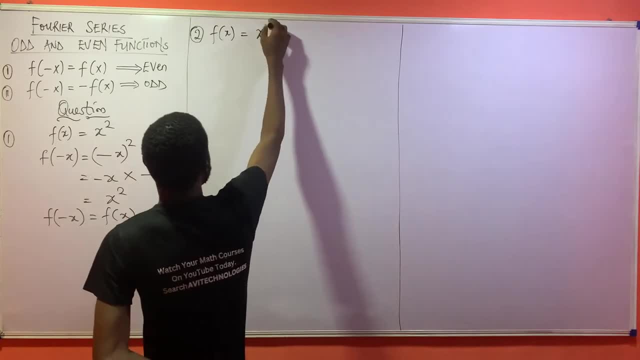 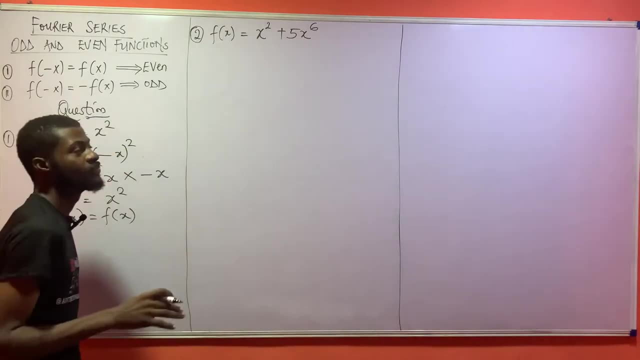 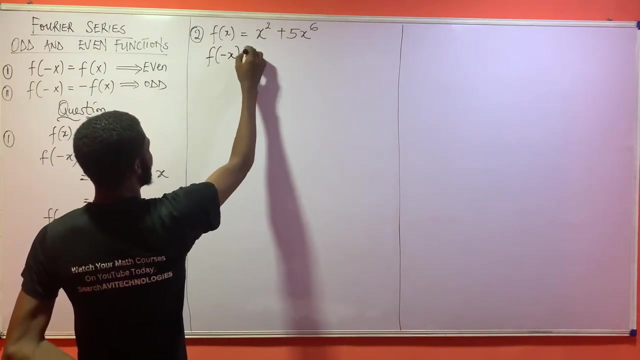 we have f of s equal s squared plus 5x to the power of 6.. For example, something like this. For example, something like this: Okay, now, what do we do? first of all, We try to see if f of minus x is going to give us a very beautiful answer. So I'm going to put minus s Any way you. 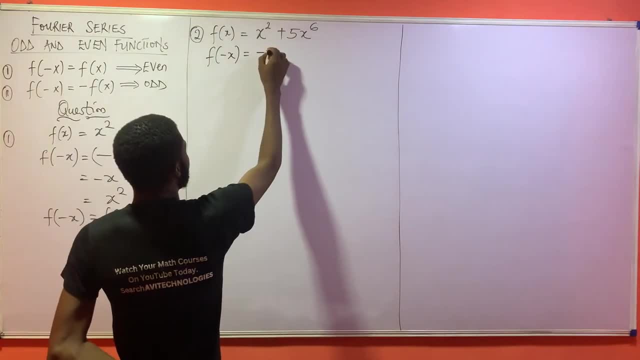 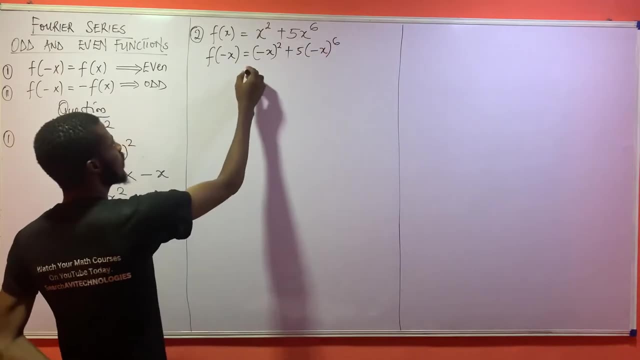 see, s you commutate the hand, Then you put minus x. So this is minus s all squared plus 5 bracket minus x. Then you put to the power of 6.. Now please, provided you are taking an even power. 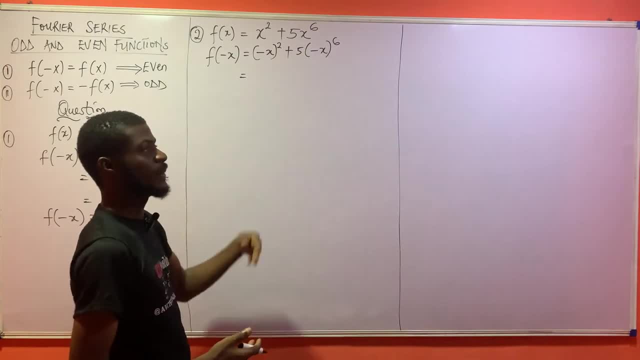 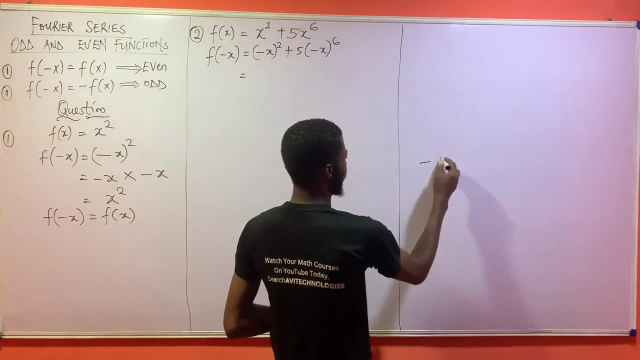 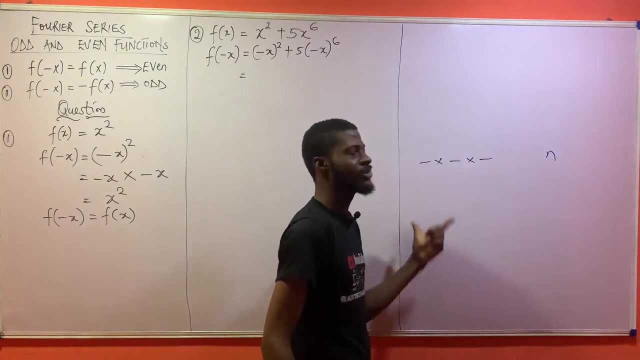 the sign is always positive, Because if you multiply the minus sign an even number of times, okay, let me say that again- If you multiply minus times, minus times, minus n number of times, such that n is an even number, your answer is always plus. If it is an odd number, your answer is a minus sign. 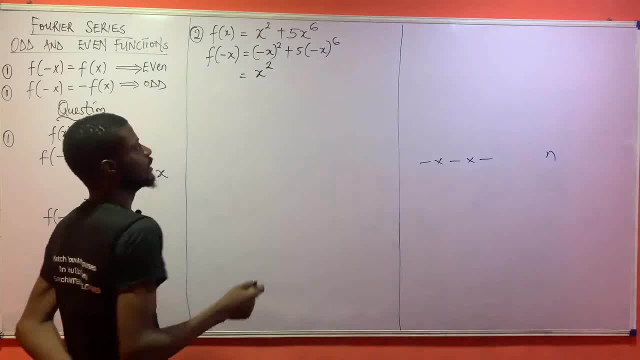 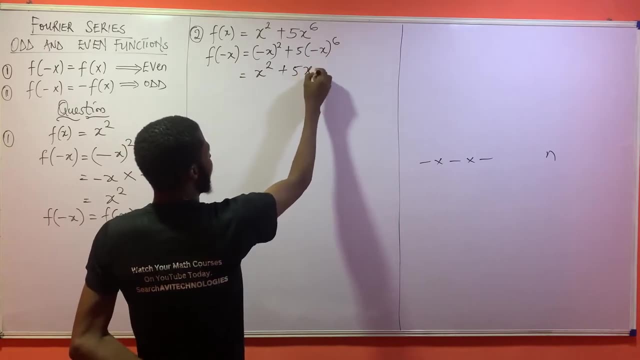 So this guy is going to just give me s squared, ideally, Now, plus 5.. What about this? minus The power here is also even right, So this is going to be positive. I will say: this is x to the power of 6.. Now, what do you notice? This function is the same thing as what this very 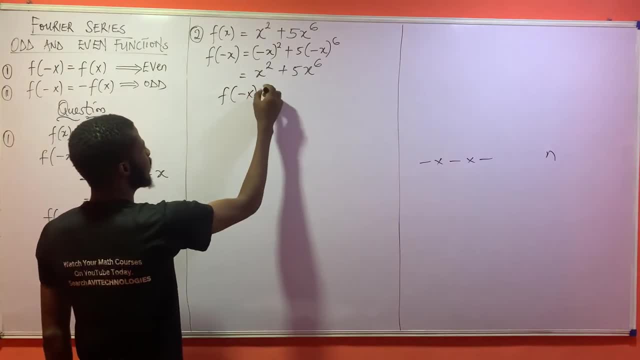 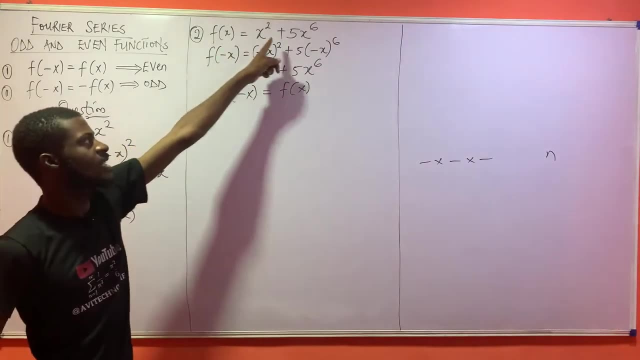 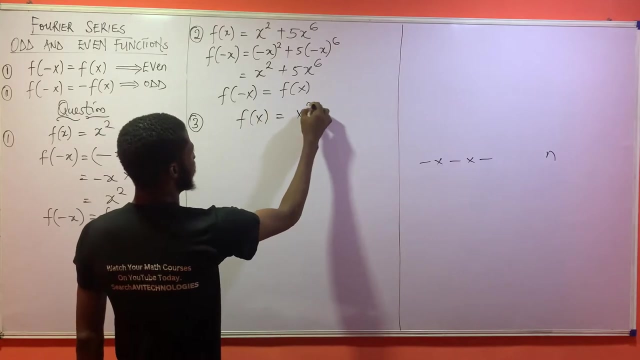 this very guy. So it means the result for f of minus s is same thing as f of what x. Hence, this guy is what Even This very guy is an even function, Okay, 3.. f of s equal to x to the power of 3. f of s equal x to the power of 3.. Now let us see and let us. 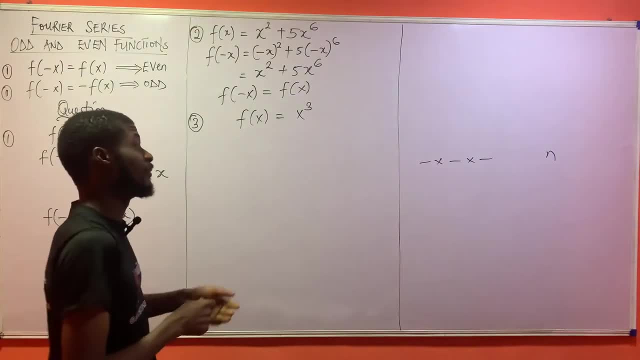 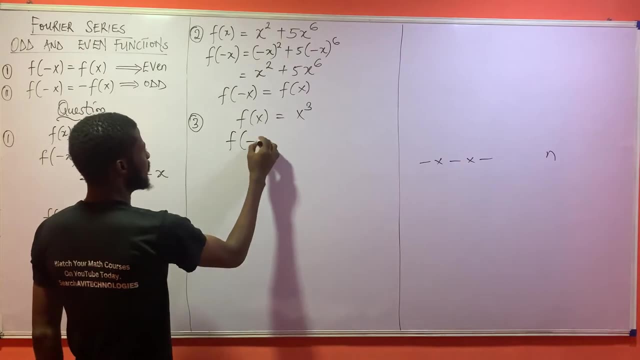 look at this. Is this even or odd? Clearly, from the power it's going to be odd. It's kind of ideal for it to be odd. So let us just see f of minus x. it is the value of f of minus. so that data. 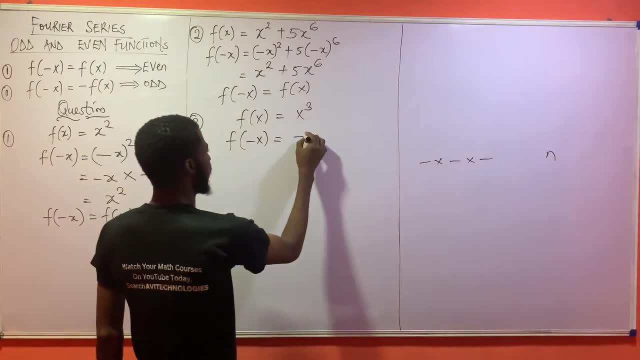 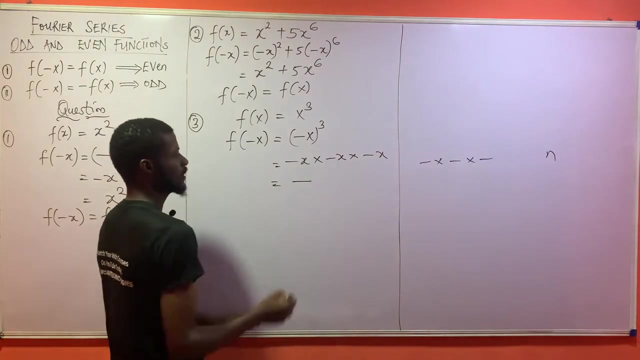 means, if it's even or odd, This is minus x everything to the power of 3.. Now, what does this mean? Minus x times minus x times minus x. Now, minus times minus is plus, Plus times minus minus s times s s squared times another s s cubed. Now what do you notice? This is an even. 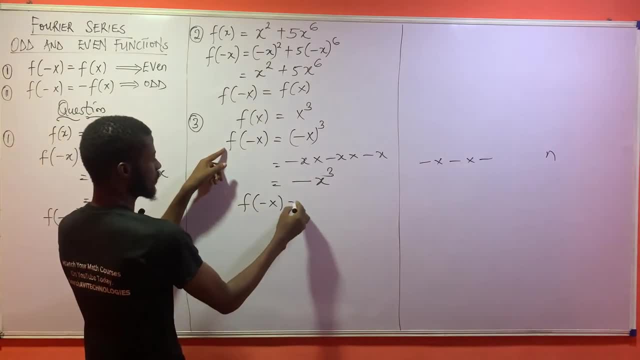 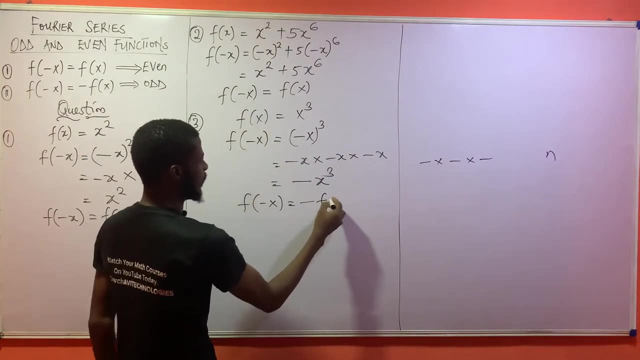 here The f of minus x is equal to minus. this is s cubed. Now what is your s cubed? You said f of s is equal to s cubed. So this is minus or odd f of s. So this guy you see here is an odd. 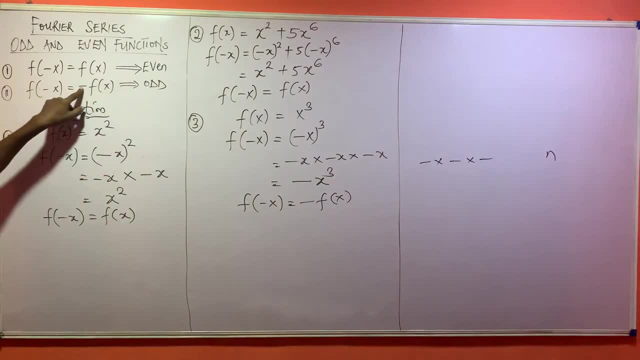 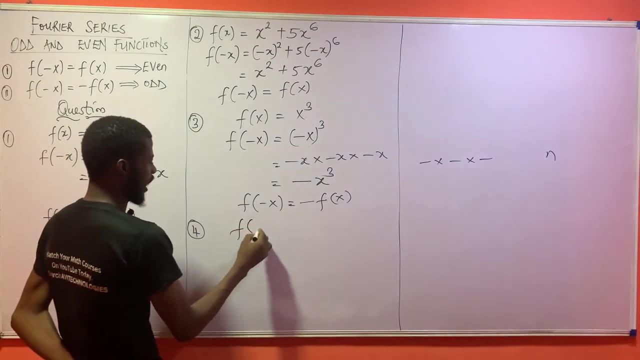 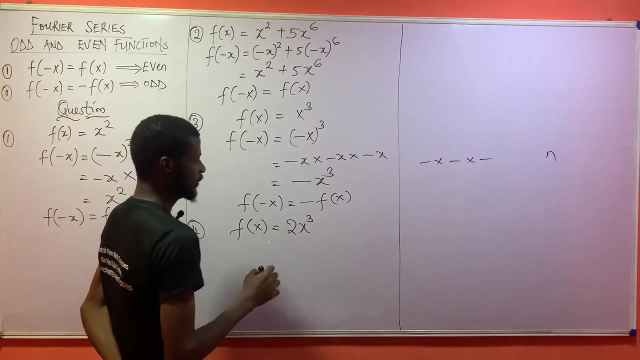 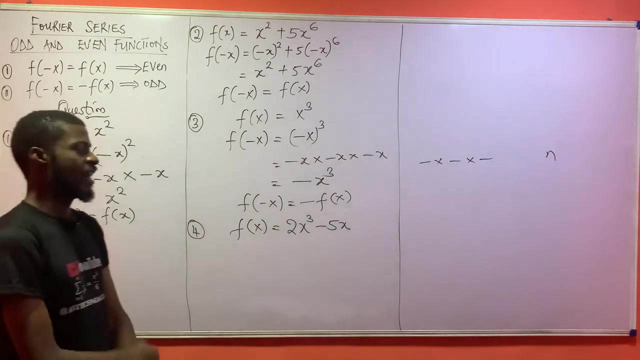 function, Odd function. So let us test the number 4.. I'm going to give 5 examples on this. f of x, equal. let us say we have 2x to the power of 3, minus 5x. Okay, just minus 5x, Let me leave it like that: Minus 5x. 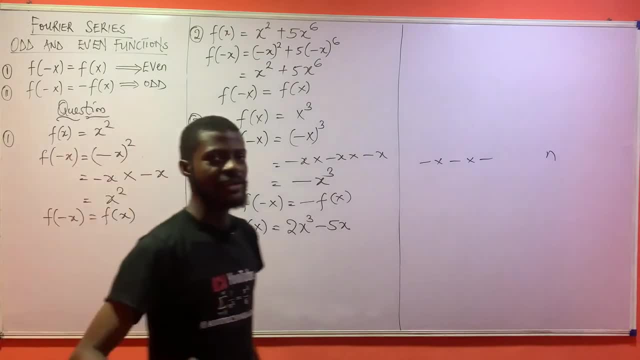 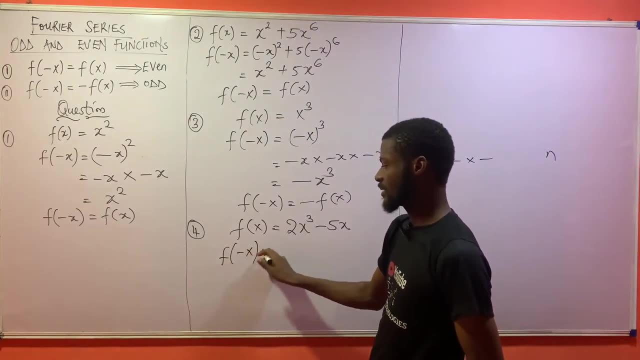 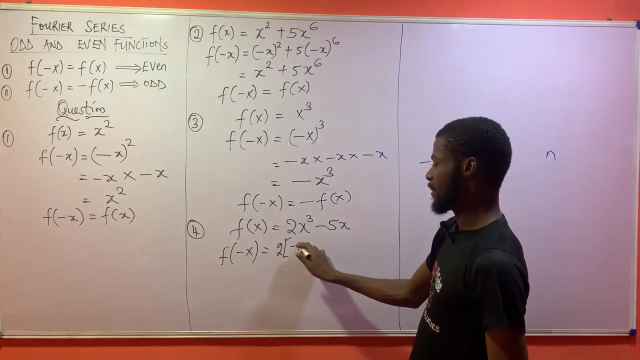 just this very one. Now let us see if this guy is going to be even or odd. Now see, obviously the first thing I have to find is f of what Minus x. So this is the first thing we're going to find. So anyway, see, as I'm going to put minus x, so this is 2 bracket minus x. 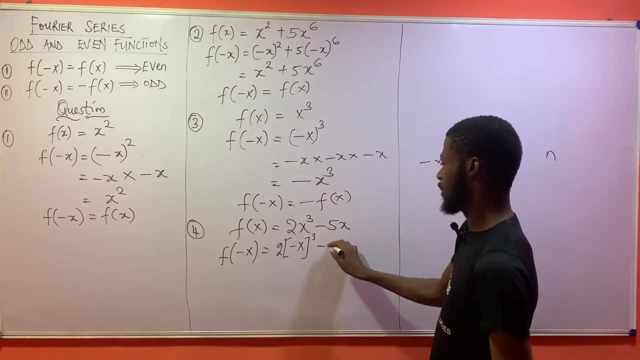 sorry, Minus x to the power of 3, minus 5 bracket. what Minus x? Now, this is 2.. What is minus s cubed? This would give me what Minus s to the power of what Theory? I believe you agree with that. 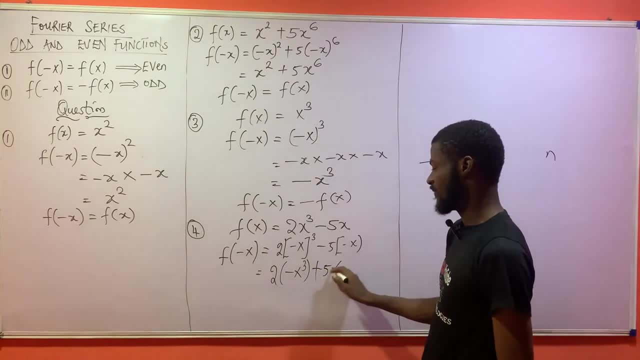 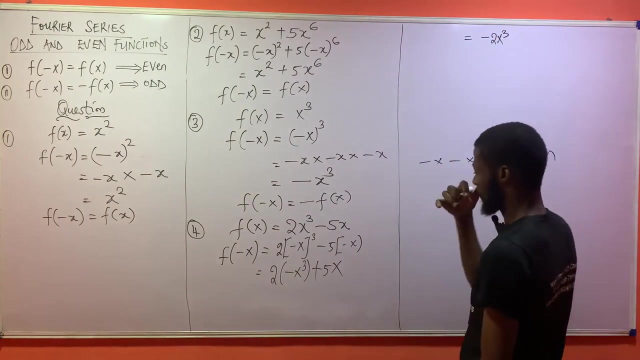 Minus times. minus is plus 5 times s is what 5x? Okay, now let me calm down a little. Okay, sorry, Calm down or come up a little bit. Okay, so let us come up. Minus s cubed is minus 2s cubed. Then plus what 5x? So what answer is this f of what Minus x? 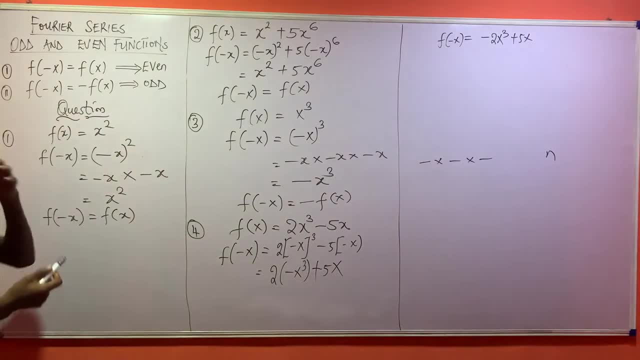 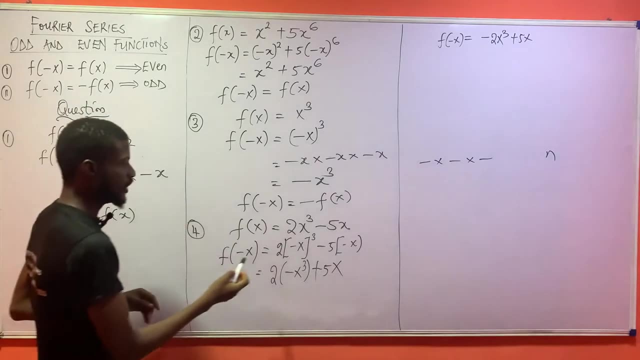 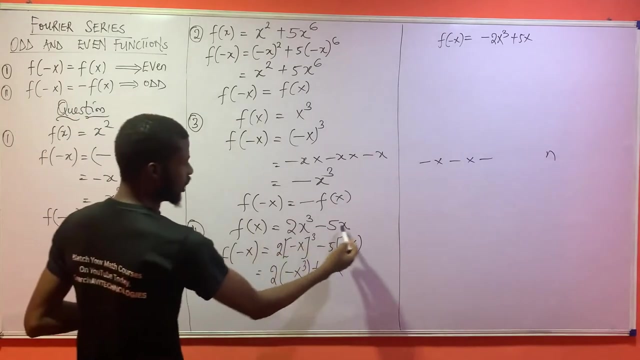 Now, what do you guys have about odd function? If you have an odd function, if you have an odd function, everything is going to change its sign. See, this is 2s cubed plus 5s. Everything is going to change its sign. That's why this minus is outside. Everything is going to change its sign. 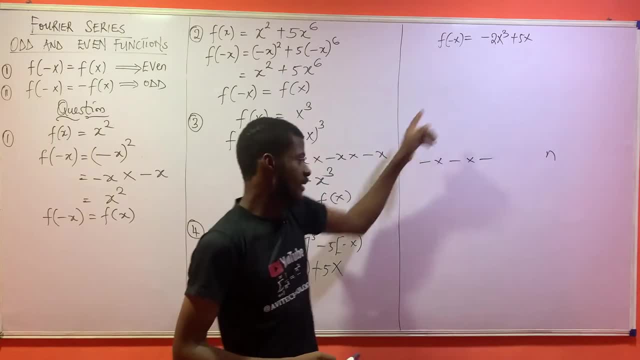 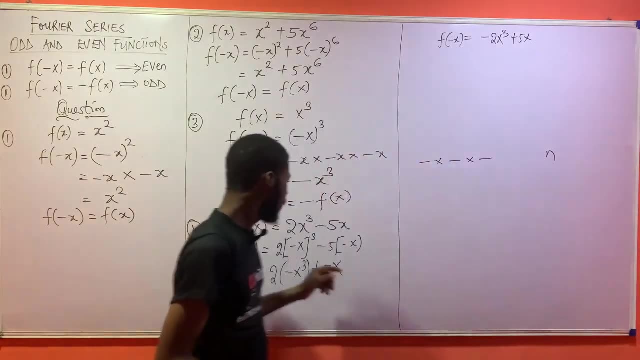 This guy and this guy did the sign change. Yes, This is 2s, cubed with a plus in front, even though it's invisible. Then at this part it became a minus. This is minus 5x At this part. 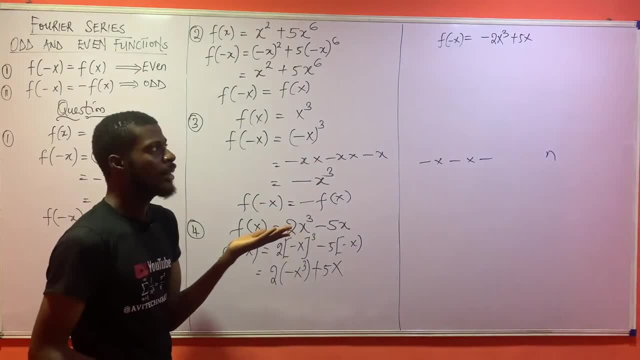 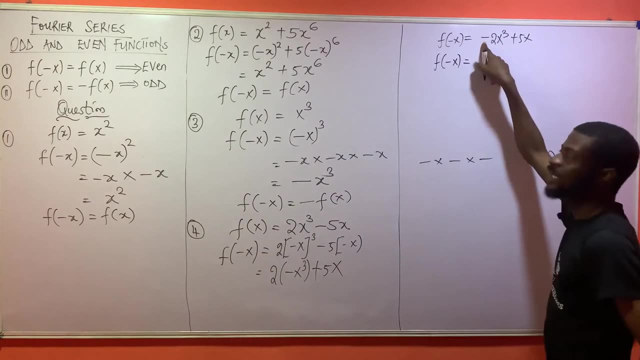 it became plus 5x, So I can say that this function is odd. But let me assume I want to proceed further. That's what I'm going to do. I will say f of minus s is equal. Let me factorize. 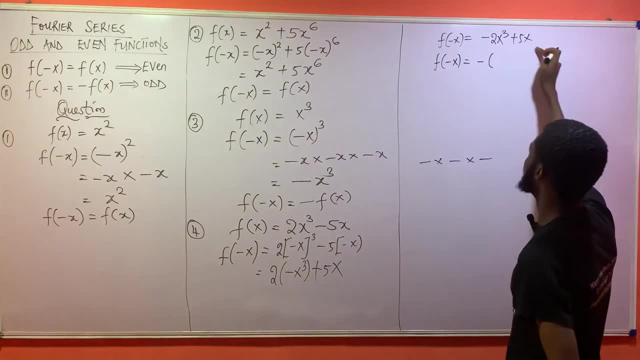 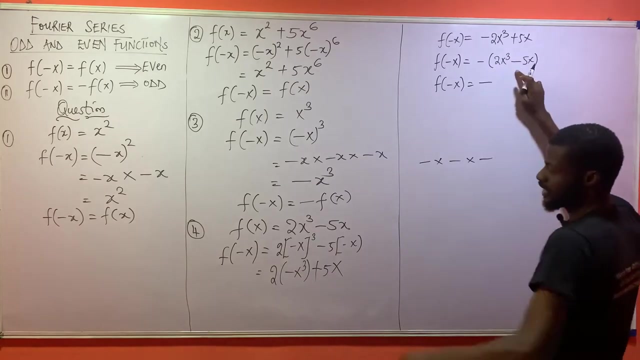 the minus sign. So this is minus Everything here, since minus can't so be remaining. So s cubed plus minus is minus. Then you have your 5s right, And this will become f of minus x equal minus everything here, Is it not the function? Look at it: Everything. 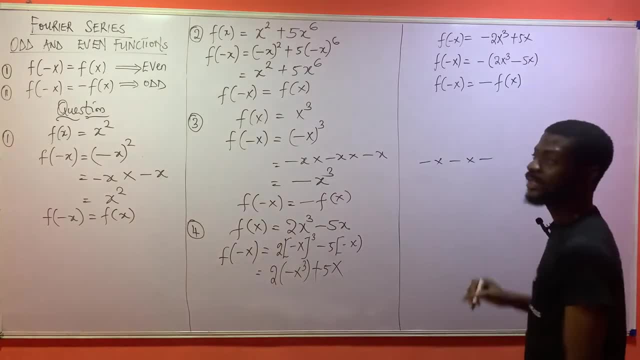 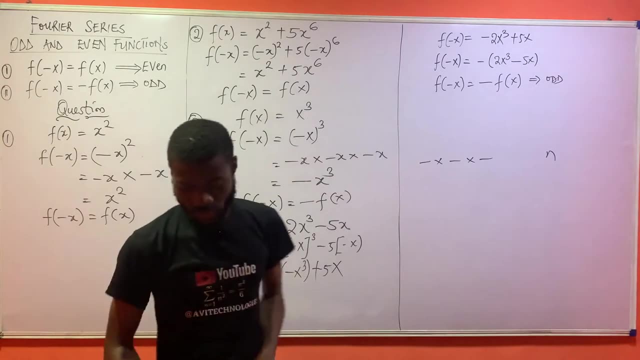 here is the function right. So this is minus f of what x. Now, what has just happened? This guy is an odd function, So that very function is going to be an odd function. That's what we're going to be having: Odd function. 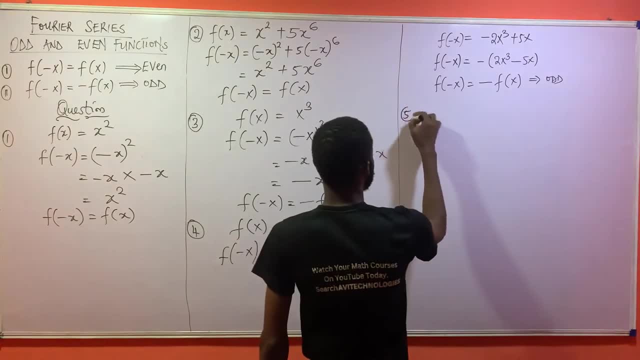 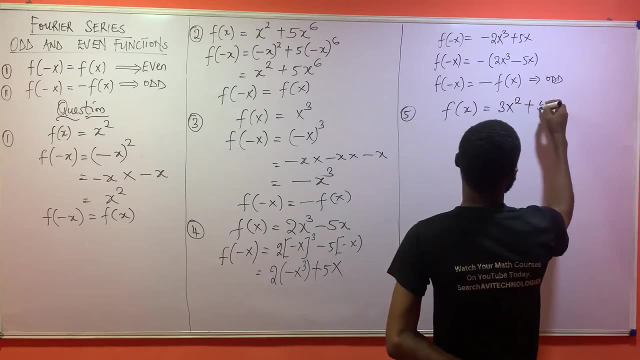 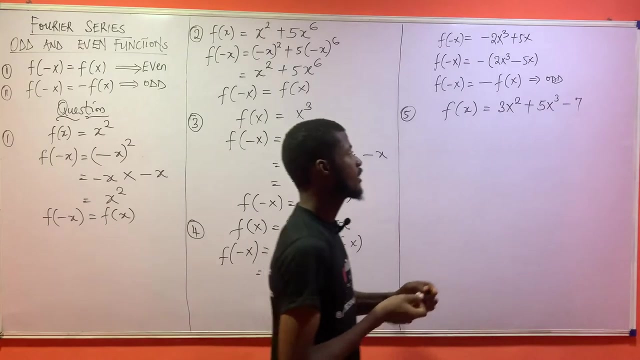 Okay, The five. Question five. Let us say we have f of s equal 3s squared plus 5s cubed, minus 7.. Something like this: Minus 7.. Okay, Well, as always, ideally, minus 7 is an even. 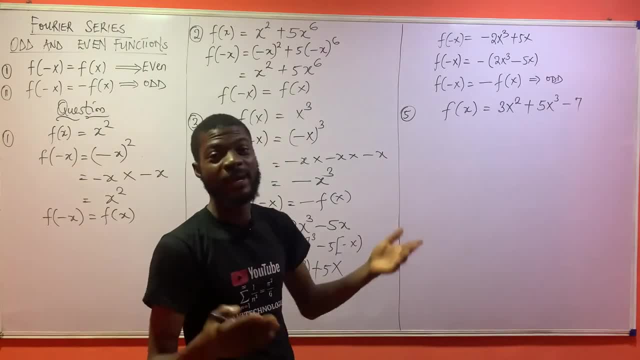 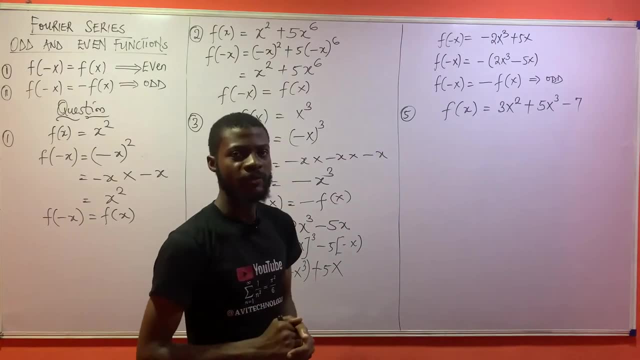 function, Even though, like, our answer is still going to remain minus 7.. It's not going to change, So, but let us look at that carefully Now. will this be an odd function? Yes, it is an even or an odd function. Look at it carefully. Would that be an even or an odd? 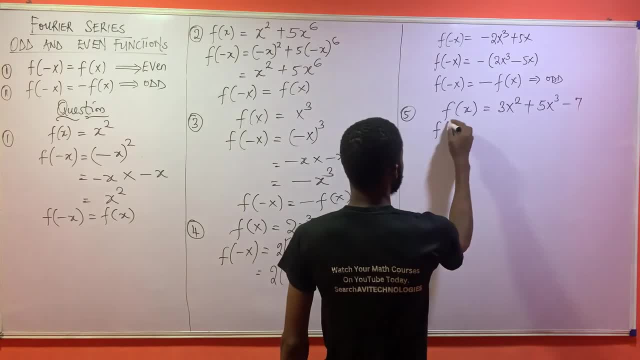 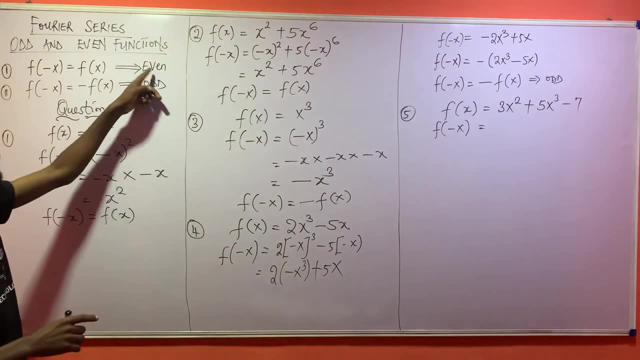 function. So how do we know? We're going to first of all test it with f of minus what x? Let us see what this will give to us. Remember: if the function is even the result of this remains the same as the original function, But if it is odd, every single thing. 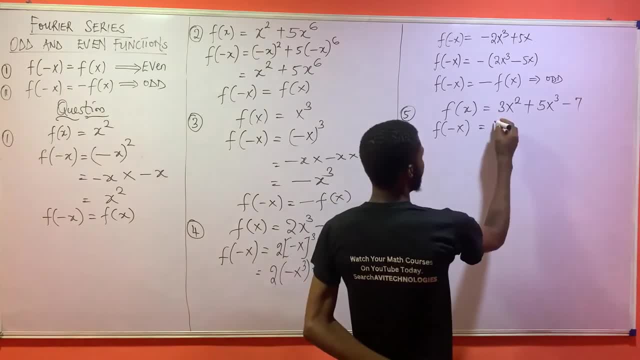 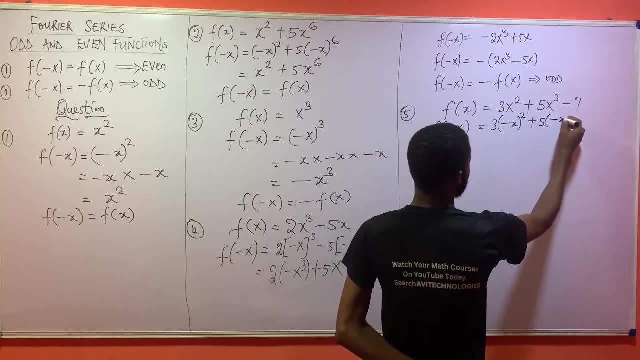 is going to change its sign. So let us start. This is theory. Bracket s is now minus x all squared, Plus 5. bracket s again is minus x, all cubed. then minus what? 7.. If you want to, you can. 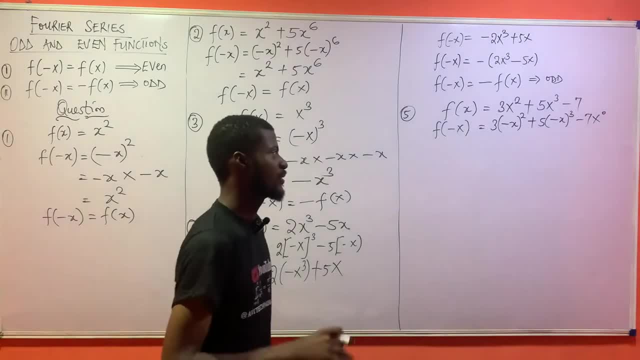 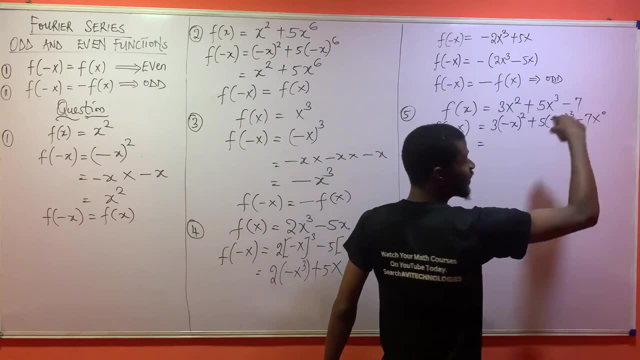 put s to the power of 0. But it's still useless, So no need for that, And this will then become sorry. if you want to put minus, it's still the same thing, So no need Now this will. 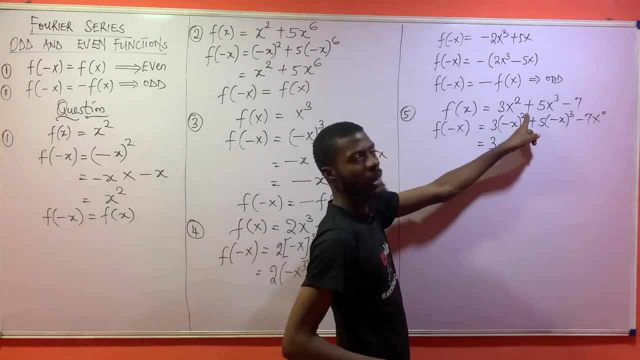 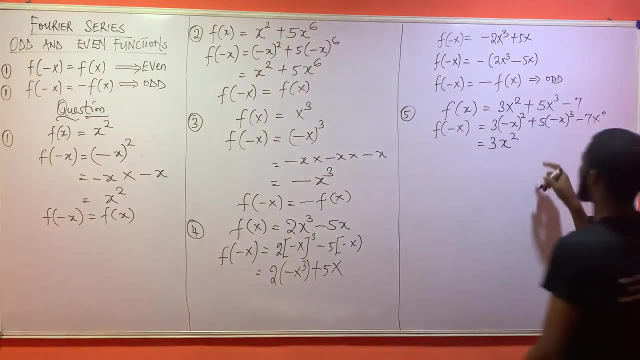 become 3 minus s all squared. What would that give to you? Minus s all squared. What would that give to you? That would just give you s squared, Just give you s squared. Now I am saying plus times minus. Now, plus times minus, is what Minus? Why am I saying plus? 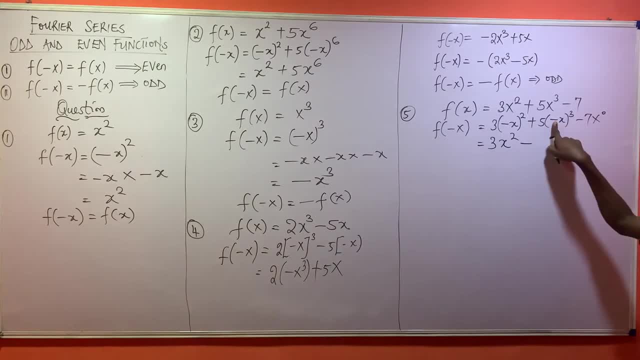 times minus. This guy is odd. So if you say minus times, minus times, minus 3 times, because this is a cube, right? So minus times, minus times, 3 times is going to give you another minus. You put your 5,, then you have your s to the power of 3.. Then minus what? 7.. Now 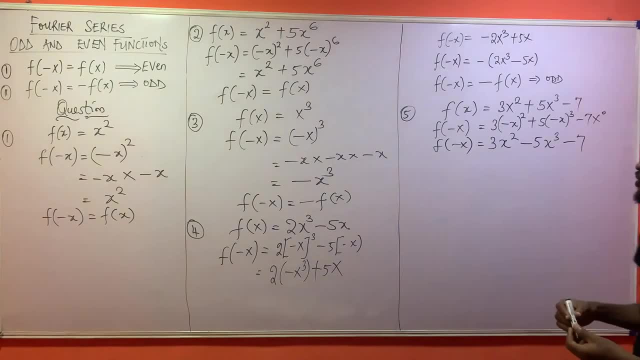 this is your f of minus x. Now look carefully This result. is it the same thing with this very guy? No, It's not the same. So the function is the same. It's the same. It's the same. 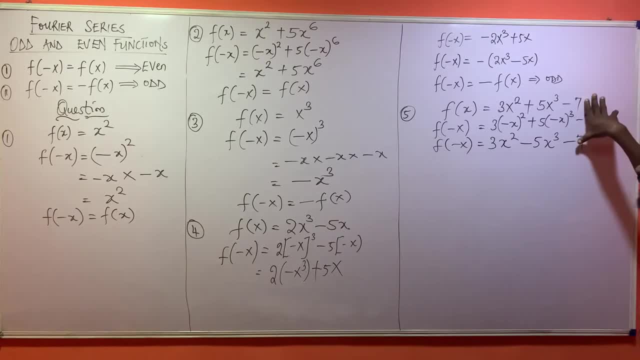 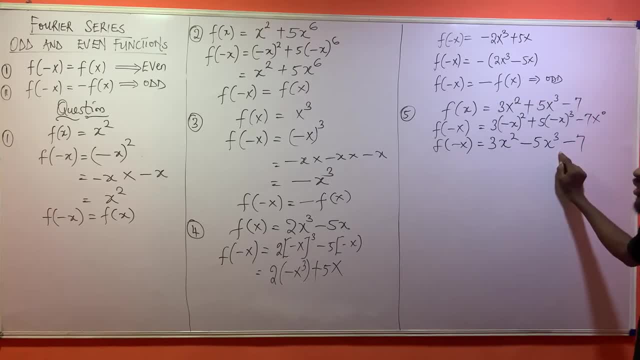 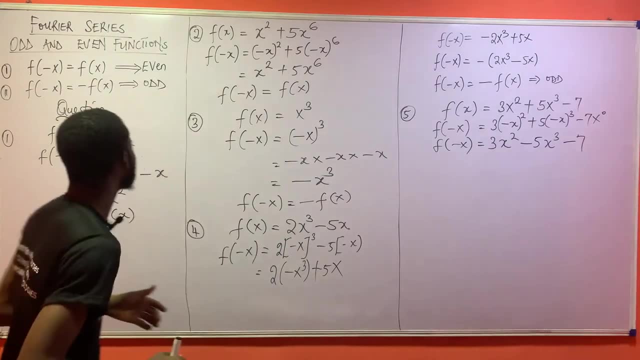 change here for this very guy. No, So it's not odd, because look at it, Let me go over this again. I know you already understand, but I love saying things again. This very guy you see here, this very guy you see here. if the result of this is the same thing with 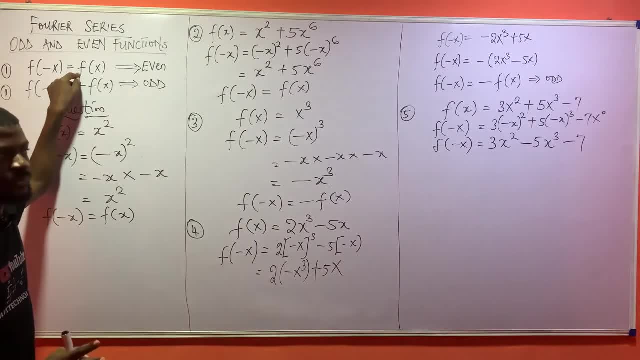 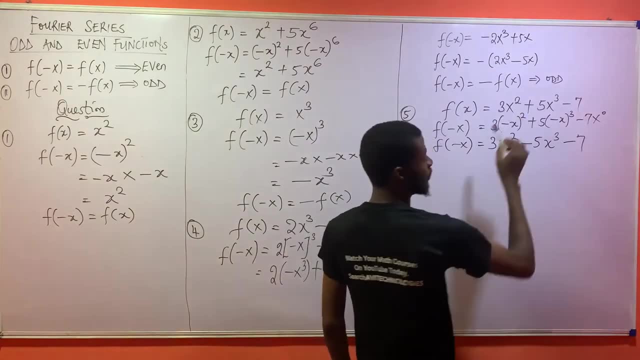 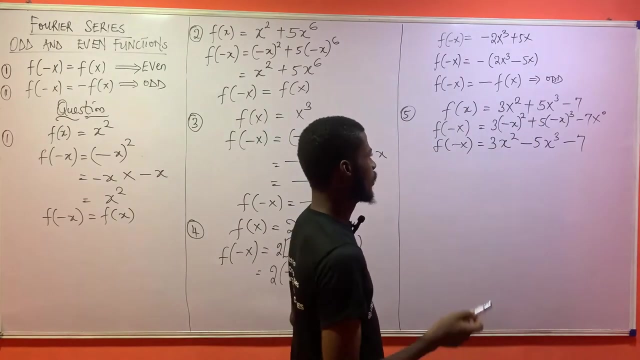 the function exactly the same. that guy is an even function. But if each sign inside changes, it's an odd function. Right now, this and this are not the same, So it's not even This guy and this guy. these signs, some of them, did not change. Look at it. 3s. 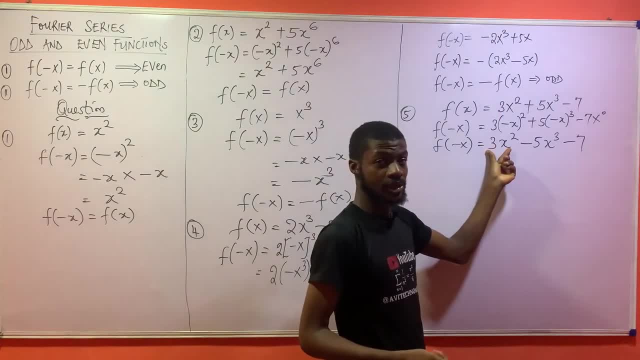 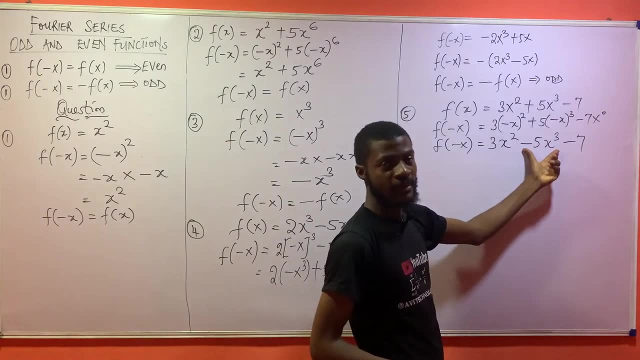 squared is still 3s squared. It did not change. It did not change. 5s cubed became minus 5s cubed. Obviously, this part is an odd part. Imagine if you want to decompose this: This part is the even part. You agree? right, This is the even part. This is the odd part. 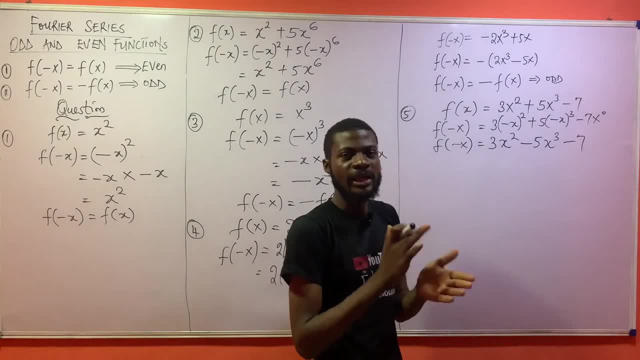 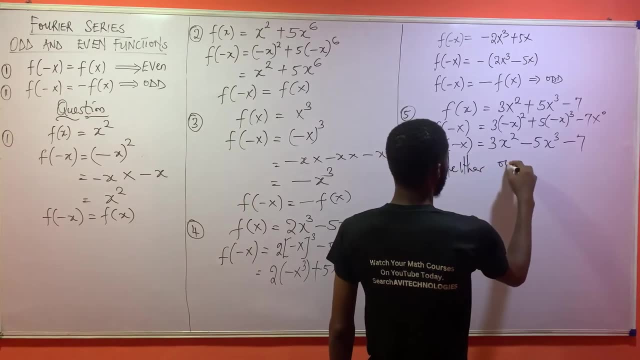 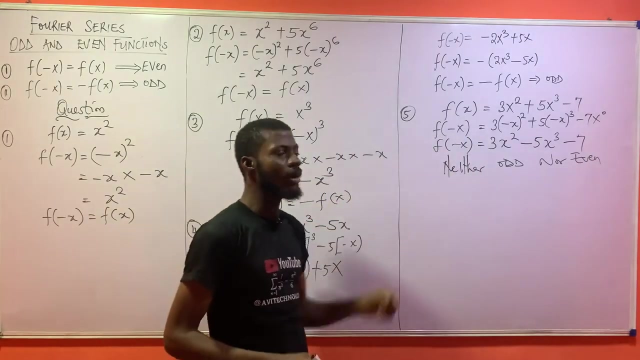 This is also what. Even Now, if you sum an odd and an even function, you're going to get a function that is neither odd nor even. Neither odd nor even So. this very guy is neither odd nor even So. this is what we have, And this happens. for what This happens? 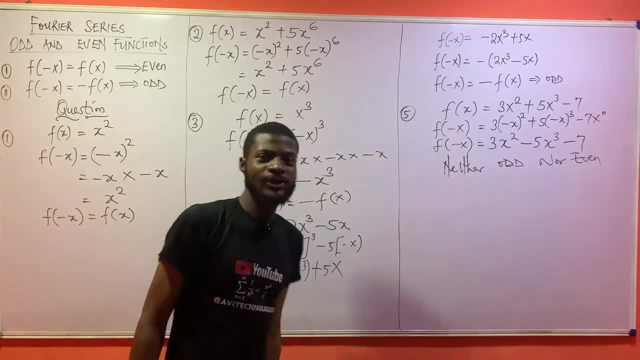 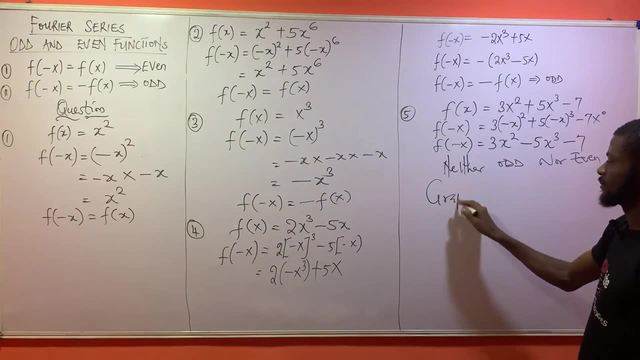 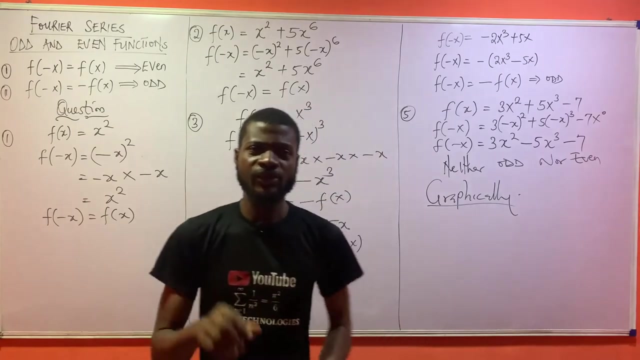 for what is it called When it's neither odd nor even When none of these conditions are satisfied? Next chapter of this: graphically, Graphically. Now in a graph: how do we know a function is even And how do we know a function is odd? How do we know all of this? Now look. 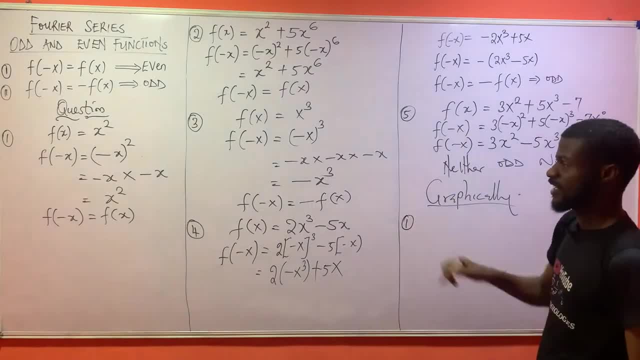 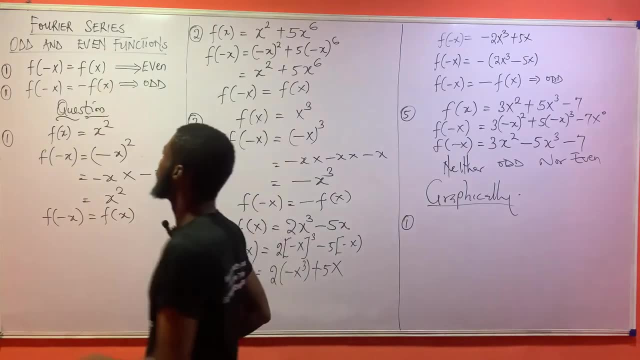 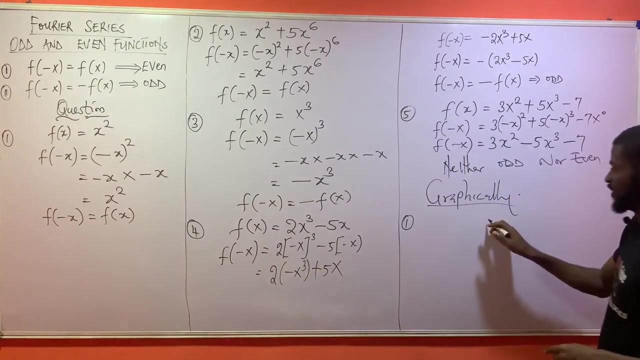 at this First part of this First part of this First part, Though, looking at this very condition, looking at this very top condition, this very guy, the negative part and the positive part are actually the same. See, Look at this, Look at this, This is your. 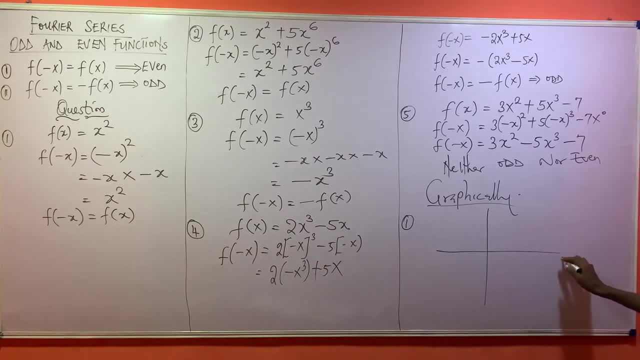 graph: right. This is positive x. This is negative x, right. Okay, Now they're trying to say that these two guys are going to be the same, So the function on this very part and on this very part is going to be the same. What that means is I'm going to be having 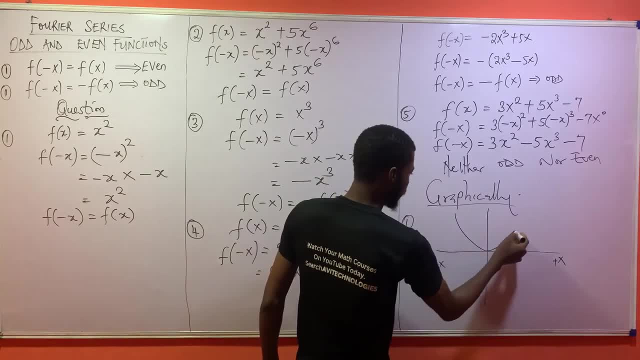 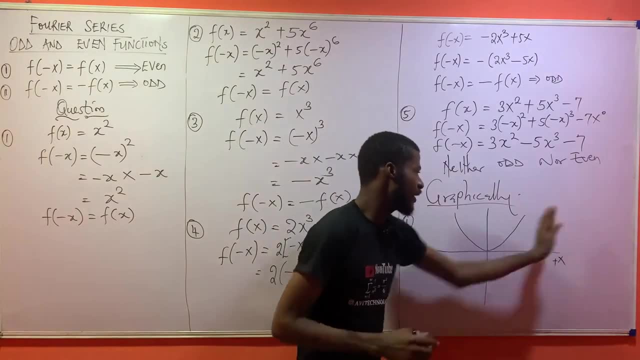 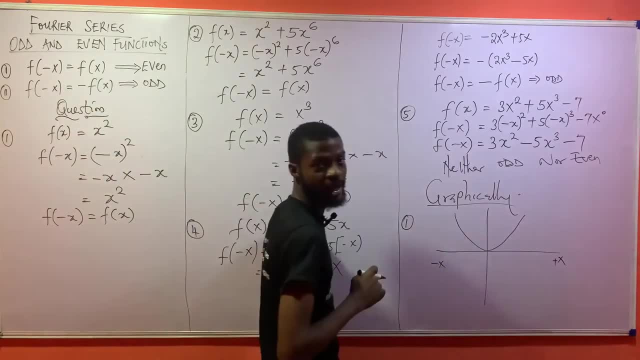 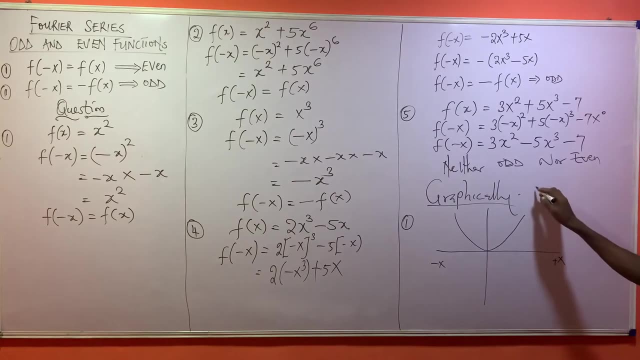 right, We agree from this very thing. This guy and this guy are the same, right. So how do we then mention this in mathematics? We're going to say that for every even function, the graph, the graph, is symmetrical, symmetric, symmetrical about the y-axis, The y-axis. 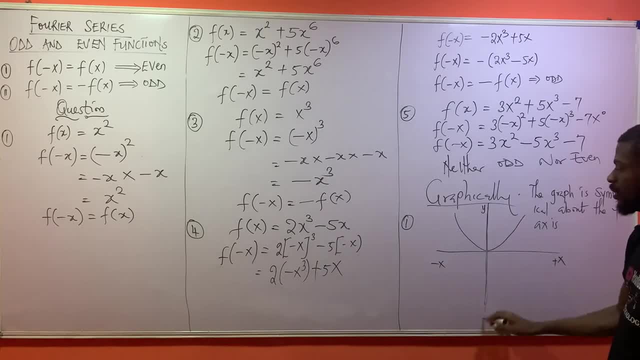 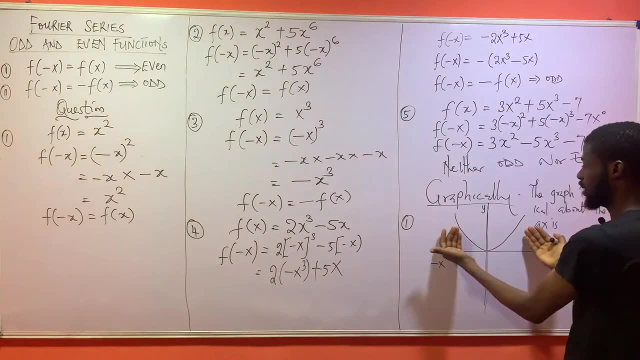 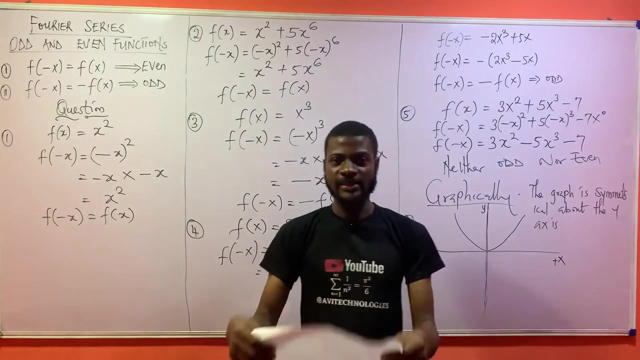 so this is the wires now. in other words, what is this saying this? saying that if you fold, it's an example, if you fold this very graph, if you close it up, this side and this side are the same, just like saying, i have a paper like this and then i fold it. if i fold this very paper, that 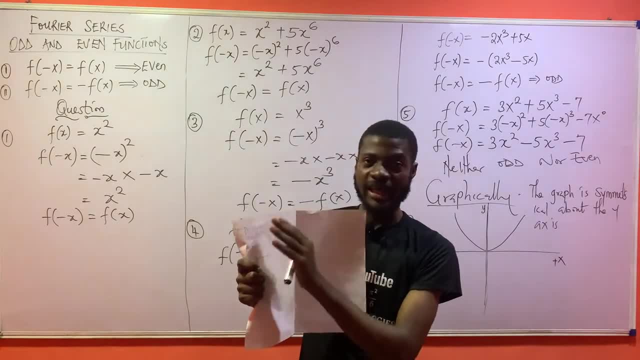 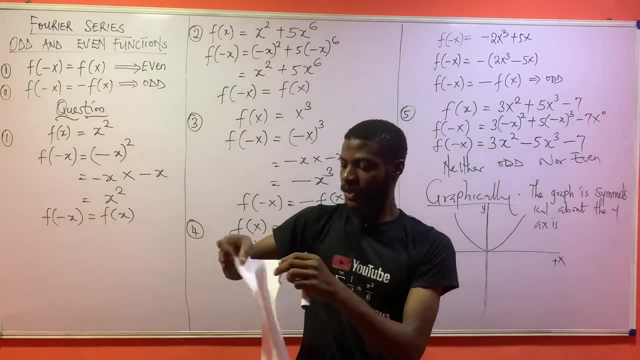 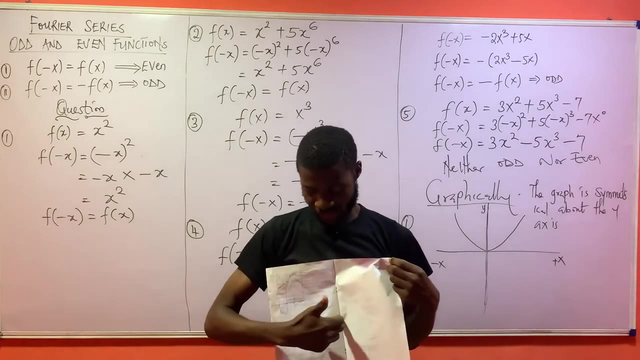 i have here, if i fold it, this very side. anything on this side is the same side. what? as you can see, they're the same side, or should i say size? rather so, these two guys, if you should fold it up, it is what symmetric about this very axis? because whatever is here, from here to here. 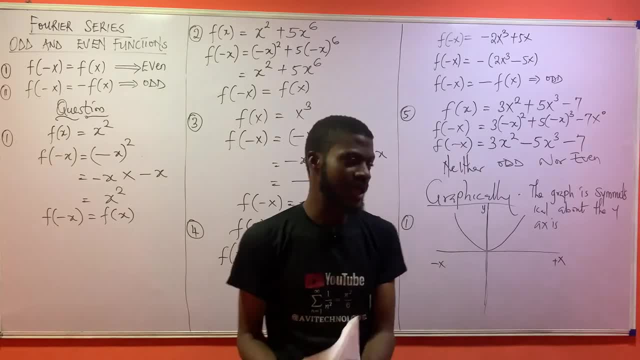 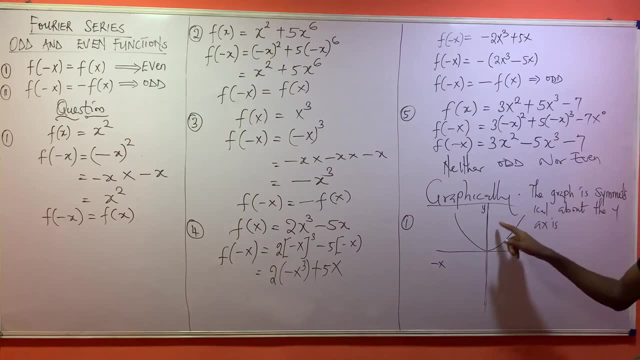 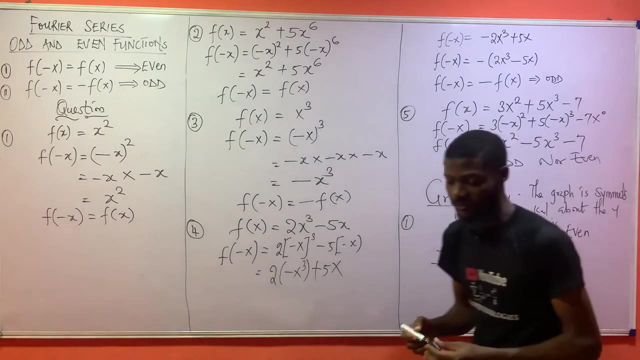 and here to here are having the same size. so it's going to cancel out. that's a counselor. it's going to be equal, rather, it's going to be equal. so this happens when a function is what is even this one, even function? symmetric about the y axis is what an even function. 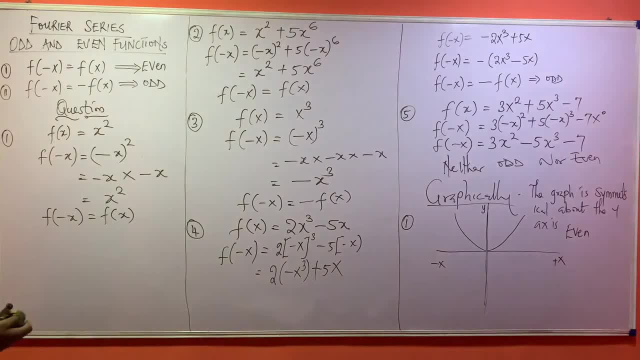 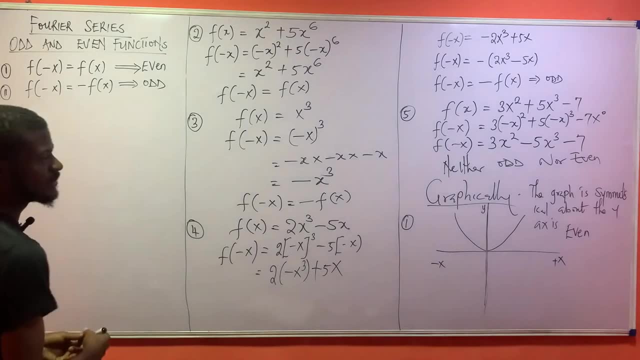 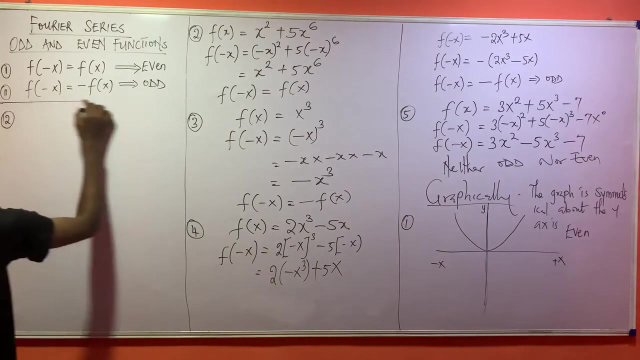 now, what about odd functions? what about odd functions? okay, let me wipe this part up. what about odd function now? odd functions are symmetrical. about the origin, about the origin. so that's one, two odd functions. odd functions, the graph. the graph is symmetrical or is symmetric? 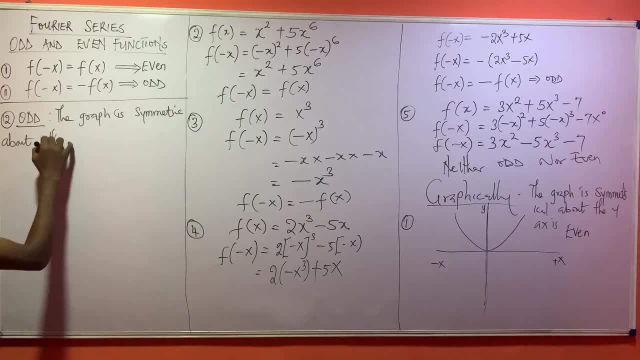 about the origin, symmetric about the origin. this is what we have and these are our conditions with graphs, and it's still the same. clearly it is the same. now let us take it. let us take some graphs. a let me assume i draw something like this. i'll draw something like this. now you are being asked: 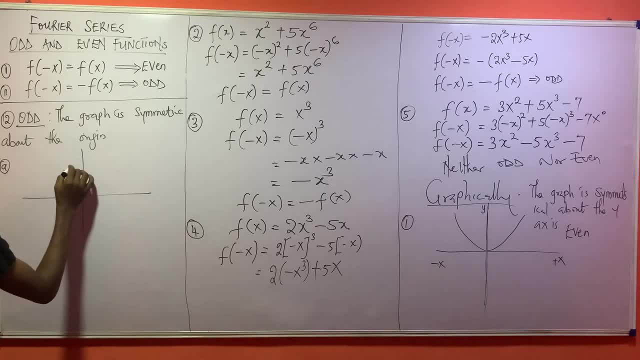 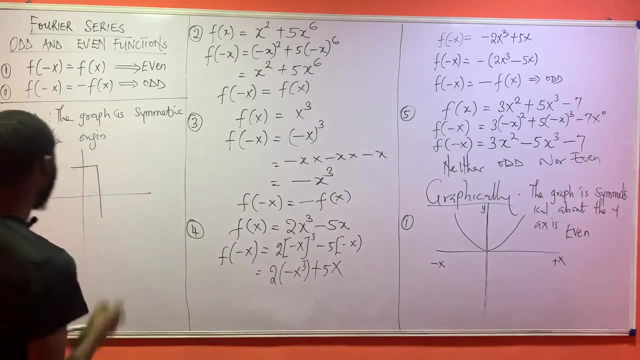 a question: if a function is symmetric about the origin, about the origin, symmetric about the origin, it is even or not. i just hope i draw this properly. you know i'm not drawing to scale, please. so, um, i think you're not going to judge me with how straight my lines are or how curved my curves are. okay, let us say i have 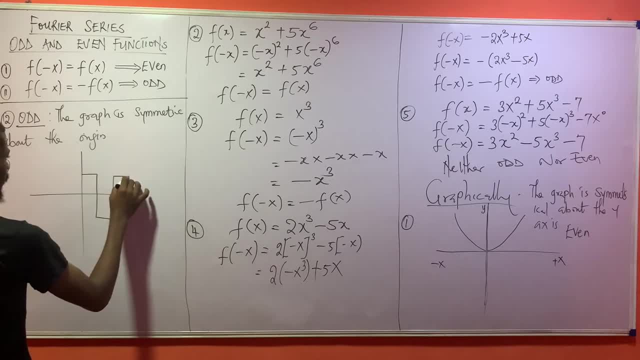 this, okay. and on this very side, okay, something like this: this is y, this, yes, sk Запas. now ask yourself, is this thing even or odd? will this function be even or an odd function? this is clearly an even function. why is it this way? look, look carefully. go to the y-axis. go to the y-axis. notice something here. everything that is. 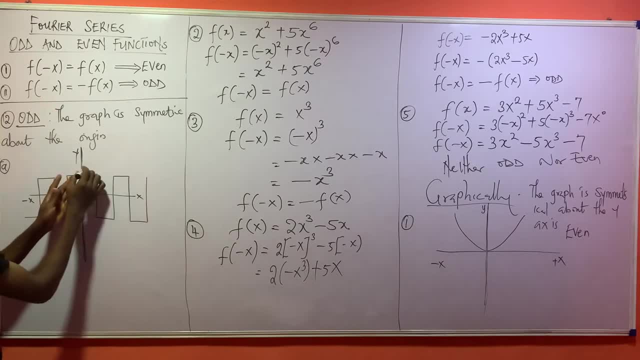 on this part is clearly looking as if whatever is starting on this very side, whatever it starts from here, is also what is starting at this very side. look at it, if we should fold this thing up, this edge and this edge will come together. look at it, they're going to come together. same thing with 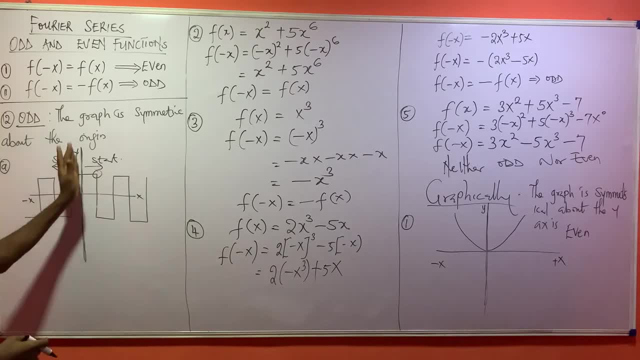 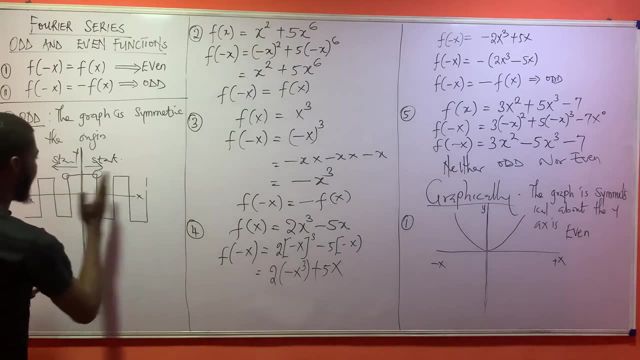 every other point here. so this guy is actually what it is symmetric with the what y, because it's just looking as if they went to y divided it into three equal parts where this side and this side are equal, because if you look at it carefully, you will see that, oh, they're actually the same. 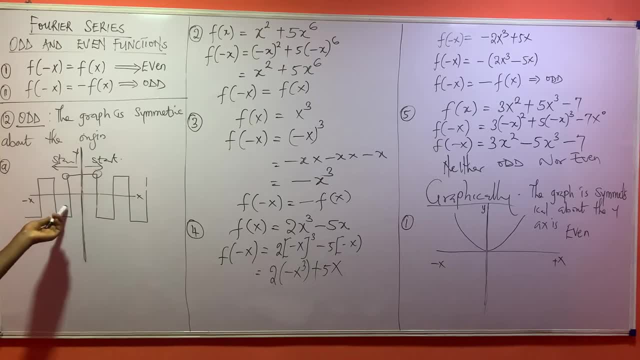 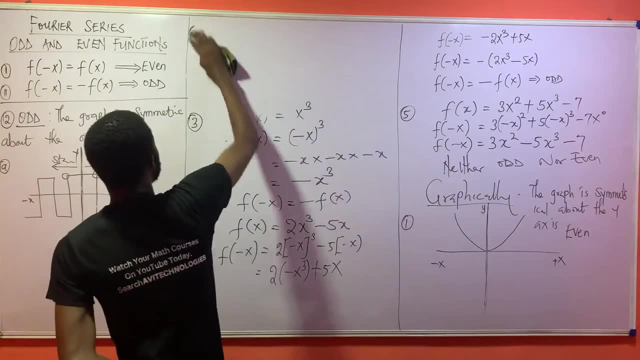 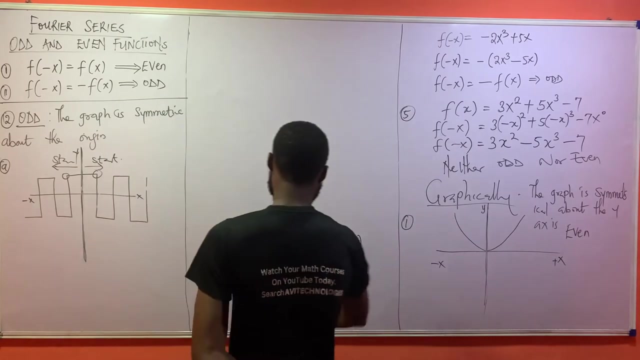 because everything on this very side is the same thing. what is at this very side, so this guy is- is an even function. you can call that guy an even function. clearly, it is even. remember to hit the subscribe button, like this video and share it to your friends. okay, let us proceed. 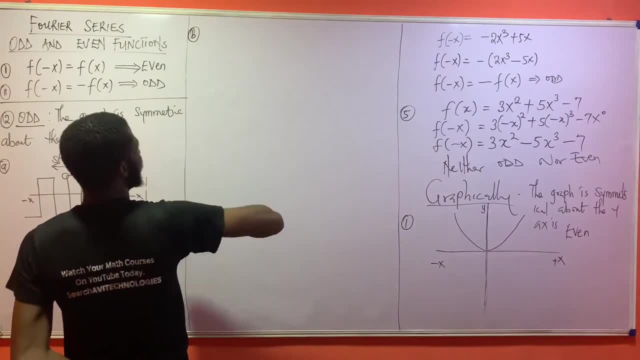 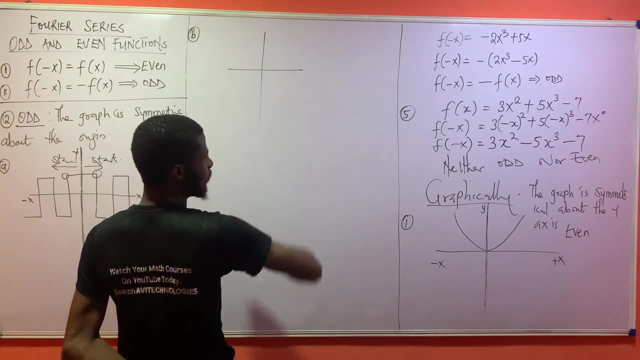 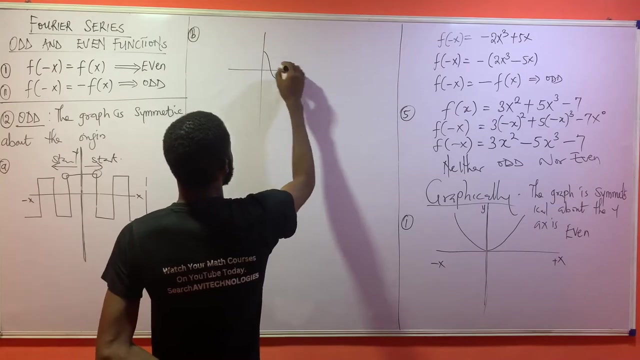 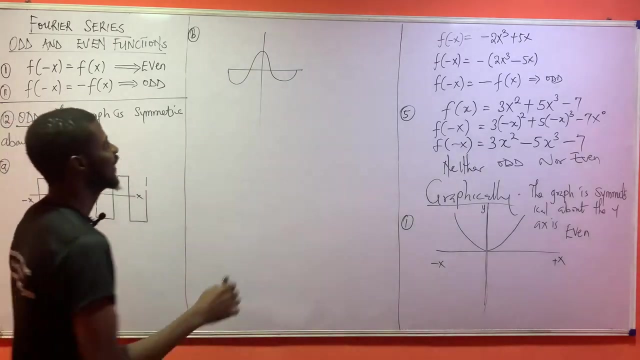 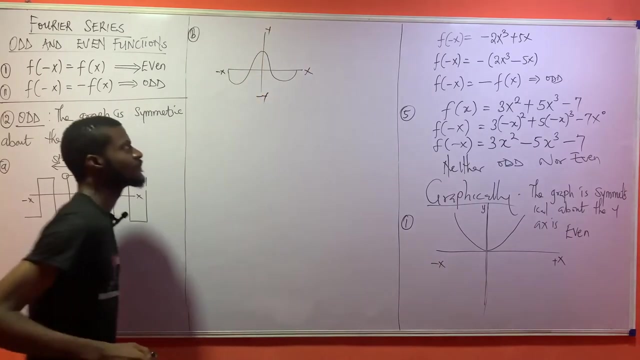 okay, b, i'm a very beautiful one, very beautiful one. yeah, let us say, we have something like um this, something like this. okay, i remember, i'm not drawing perfectly, though- so this is um x, this minus x, this y. this guy is going to be called minus y. okay, now look at this carefully. what function is this? 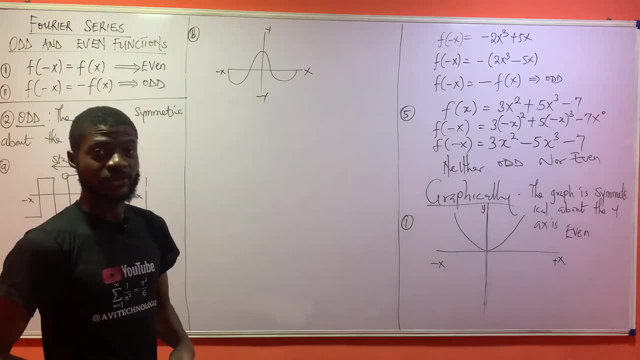 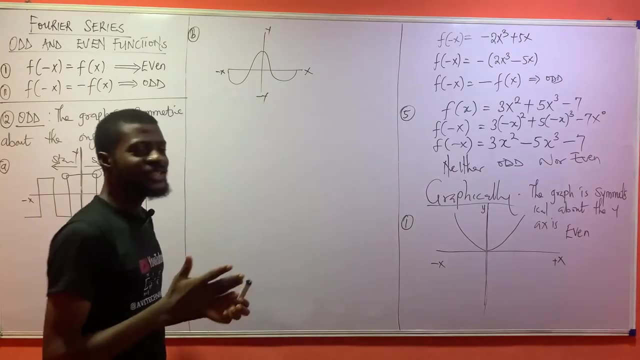 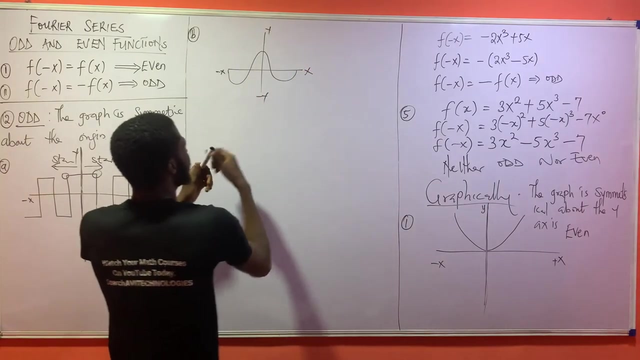 what function is this? this guy is an even function. it's an even function because if you will notice, if you will notice, if you the thing is, you just have to use your eyes. if this is your wires, if you close these two parts up, you will notice something. this segment, let me call this a let. 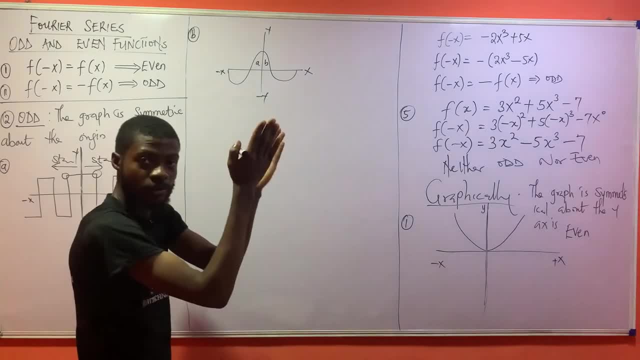 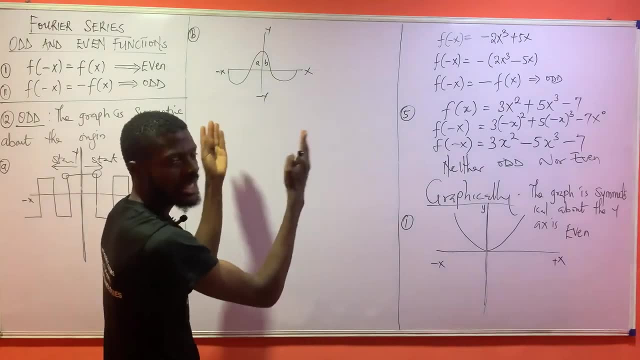 me call this that the same. they're going to cover up, kind of, they're going to cover up then, these two guys. if we notice that they are at the bottom, they're occupying the same position on both sides, so they're going to come together, because whatever is on this very side is still 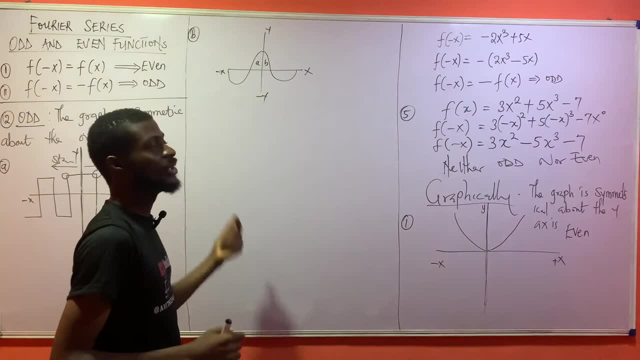 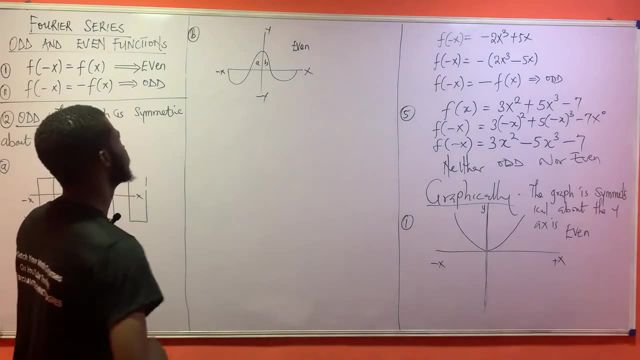 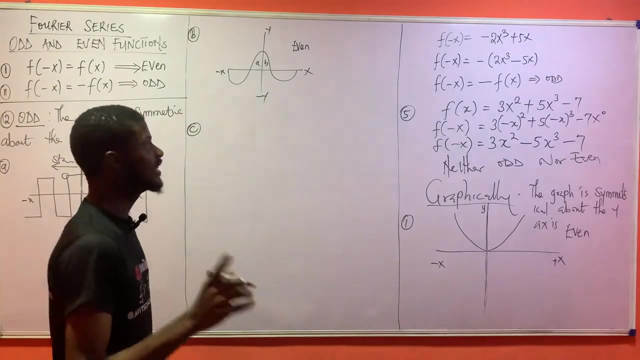 on this very side. so these guys were symmetric about the world wires. so this is an even function. this guy is also what an even function. it's even c for c. let us look at c. the easiest one for c, the easiest function for c. let me see the easiest one for an odd function. let me call this very guy. 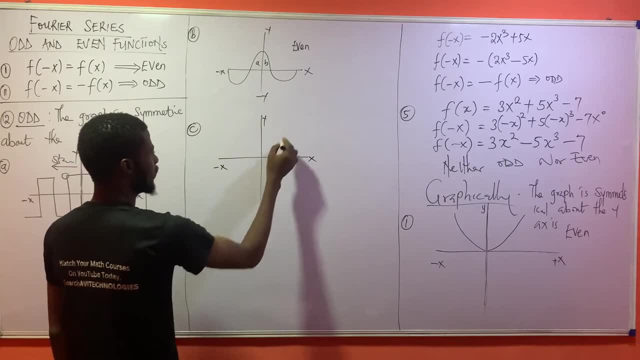 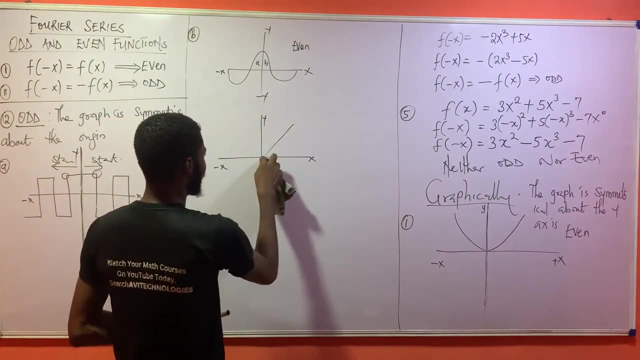 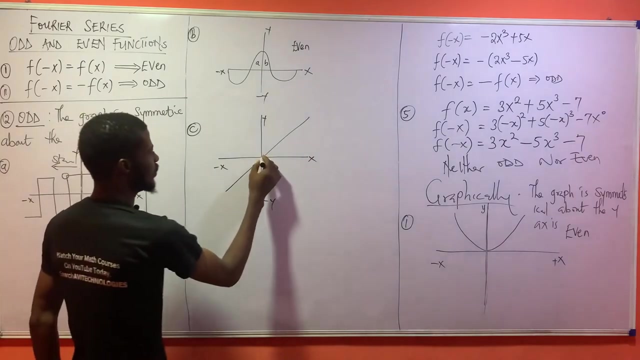 y. this is x minus x minus y. then something passes like this: okay, sorry, i think that was too sharp, too quick for me to do. okay, i think. something then passes like this: okay, let me just assume that this is the origin. okay, now this function is going to be what? this? 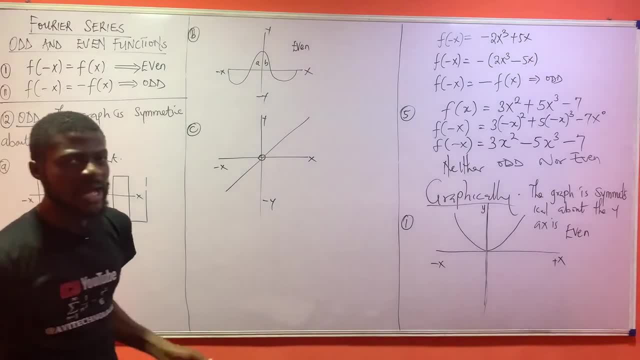 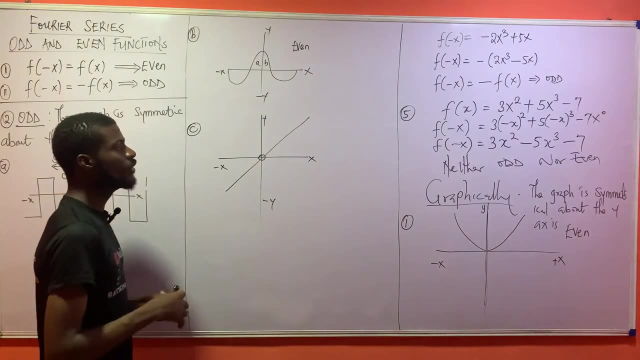 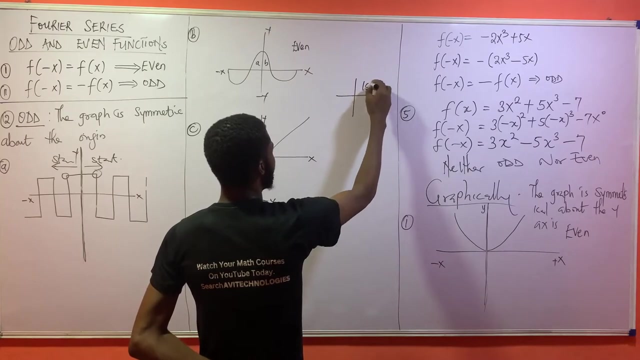 is going to be an odd function. yes, now another way. i know an odd function because i'm not talking now. how do we know odd function? see, i use this very trick in any graph. we have four sides. we have the first quadrant, we have the second quadrant, we have the third quadrant, then we 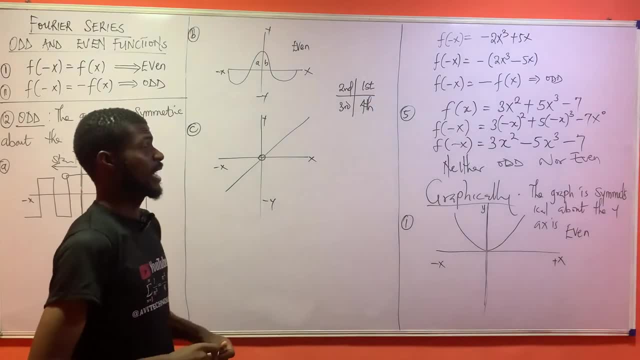 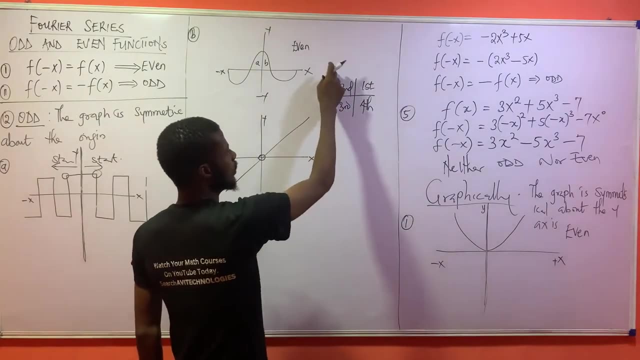 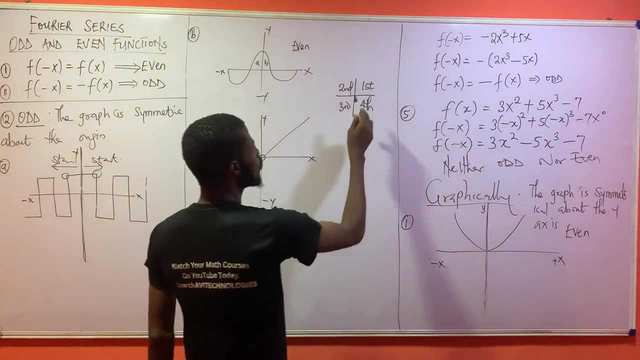 have the fourth quadrant. if i am looking at my quadrant and i notice that, oh, anything on the first is at the third, or anything at the second is at the fourth, that means that function is what is an odd function. let me go over that again. so let me not say opposite. i don't even know, at a way, on positive, if i should have the first. 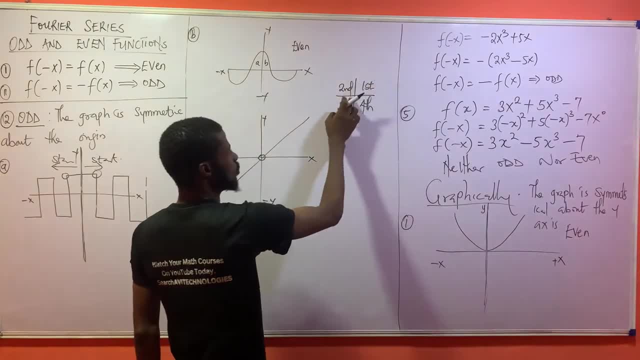 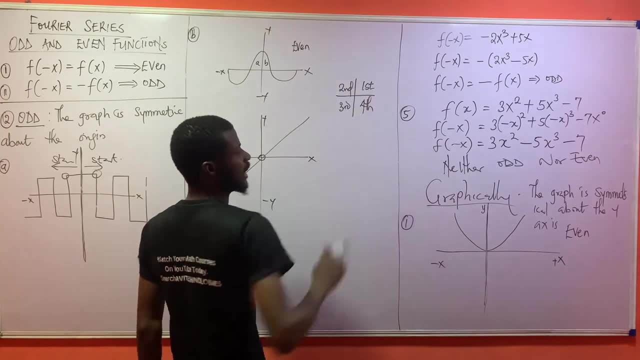 anything that occurs at the first is also occurring at the third quadrant. this function is an odd function. if what is appearing at the second and the fourth are the same, it's an odd function. but please, first and second the same thing at this very side. that's an even function. 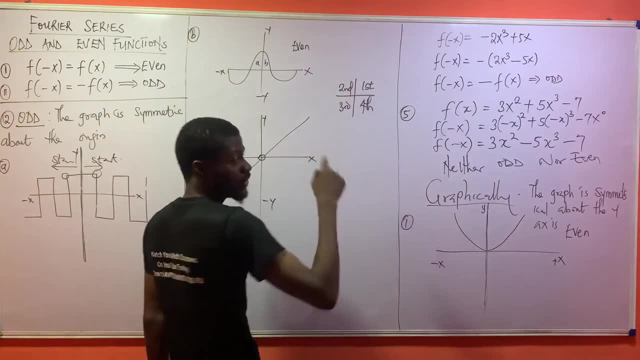 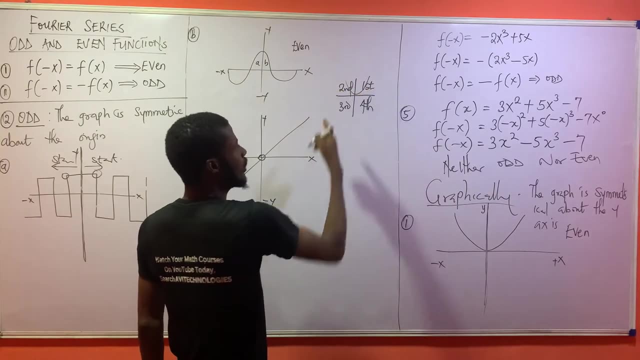 if i have the same thing on two respective, two successive quadrants, this guy is going to become what an even. because If I should have anything here and I have it here first and second, this guy is what Even. But if I have it on two opposites, let me say first and third, or second and fourth- 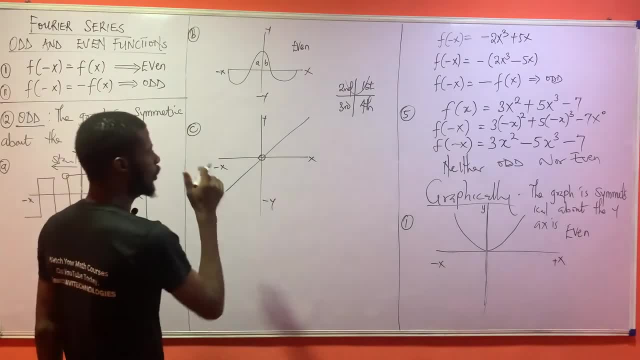 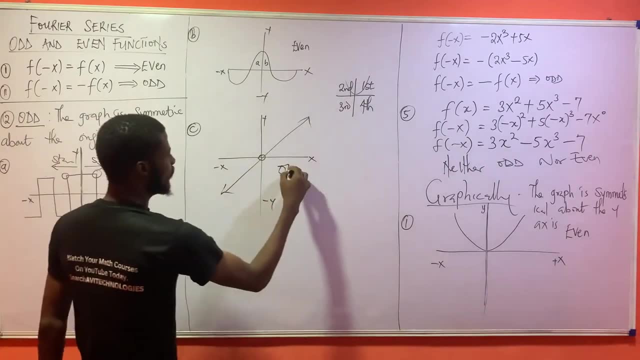 that's an odd function. Now let me go back to this Now. if you will notice, everything on this very side is the same thing as what is at this very side. Everything here is the same thing as what is here. It is an odd function. 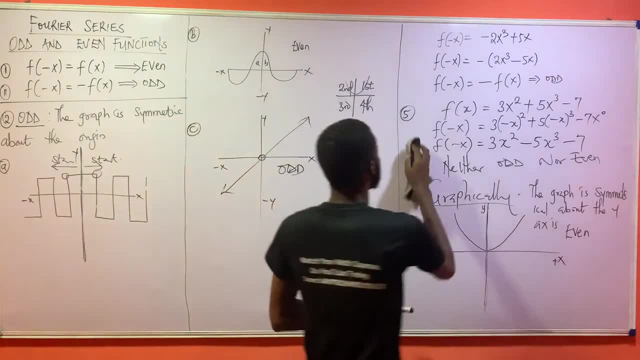 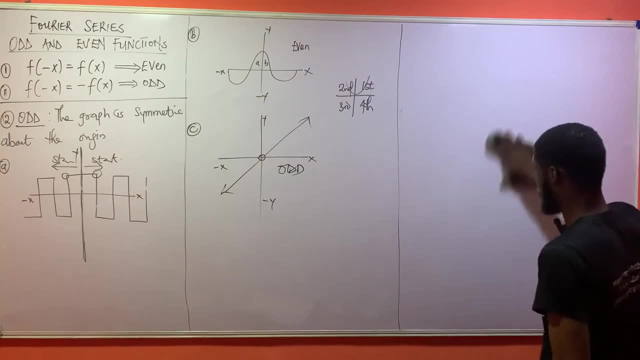 No need to actually take much time there. That's an odd function. Now another function that I want us to look at, another one that I want us to take a very good look at: d. let us say, we have something like this: 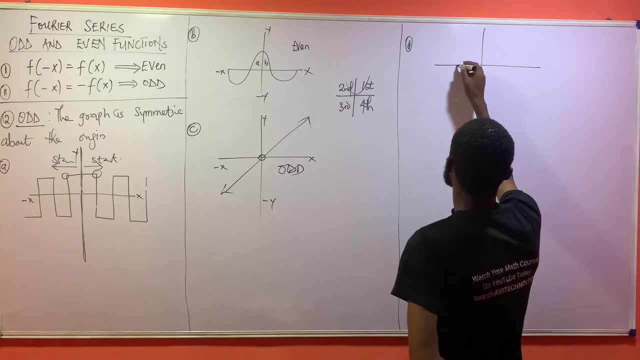 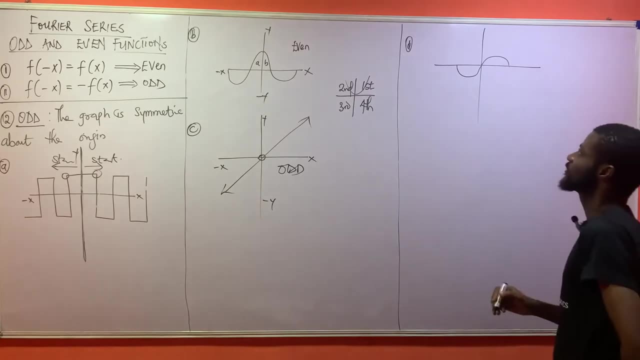 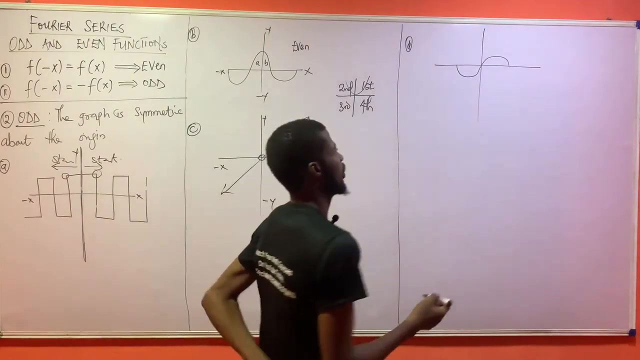 Hold on, hold, on, hold on. Okay, Something like this: Yes, Even though this is looking not really fine. Now, what function is this? This? This is also an odd function. Clearly, it is an odd function because this is first. this is third. 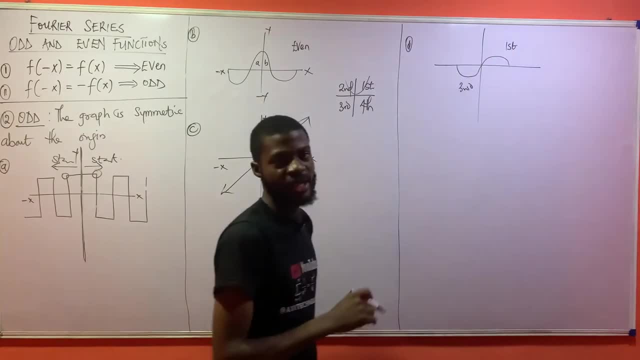 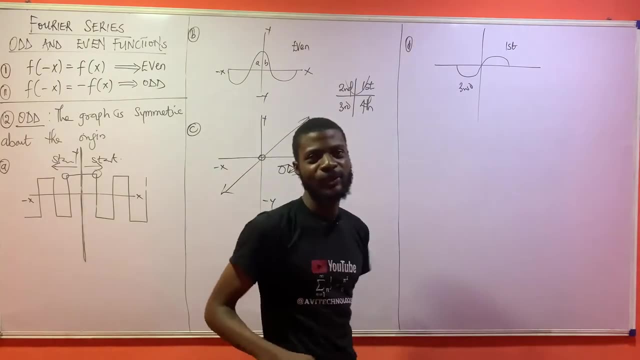 I have what is here at this very side. It's repeating itself at the other side. The same size, please. I know I did not really draw it up to up to this, but please, this guy is actually what, Correct. 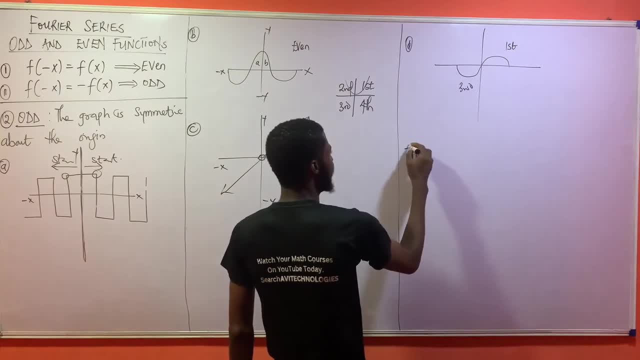 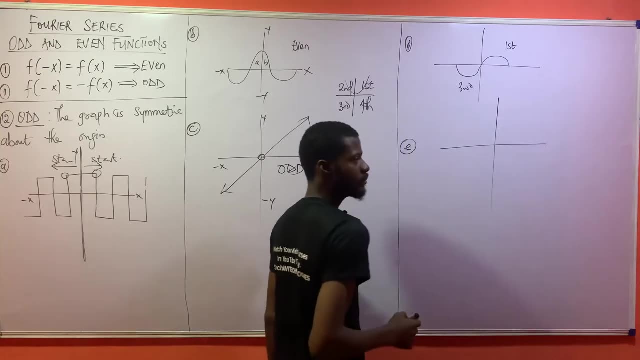 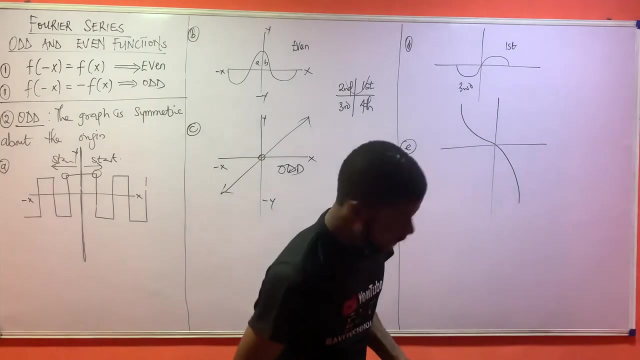 Very, very correct, Very, very correct. So this is e another example, which might even be the last. So let us say: we have something like this And then we have this guy like this. Okay, Hold on. 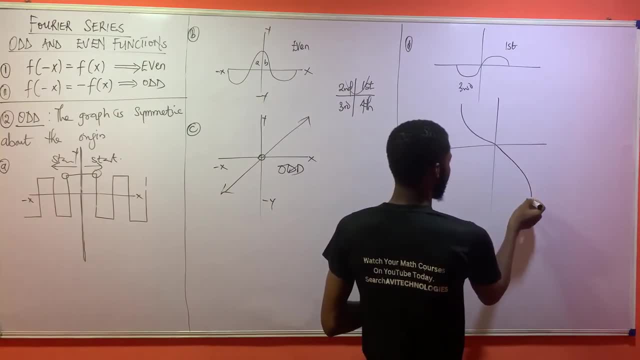 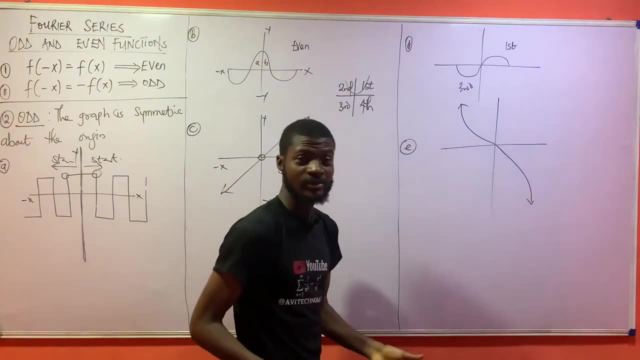 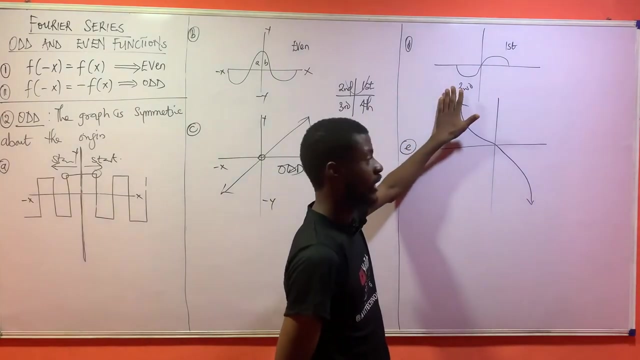 I then have this very guy. Now, is this even or odd? This guy is also going to be an odd function. Clearly it is an odd function, because what I have on this very quadrant- this is second quadrant- I have it at the opposite quadrant, which is fourth quadrant. 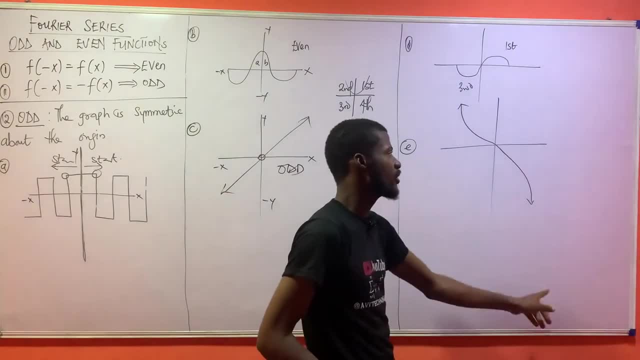 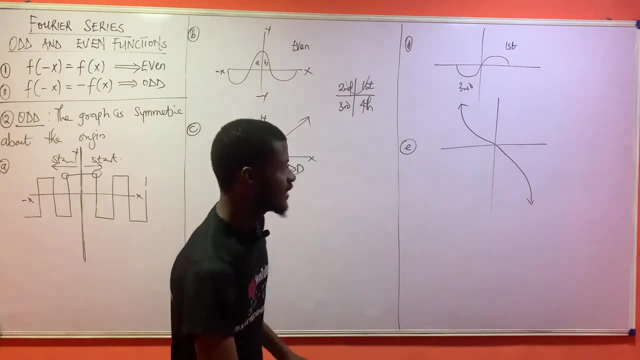 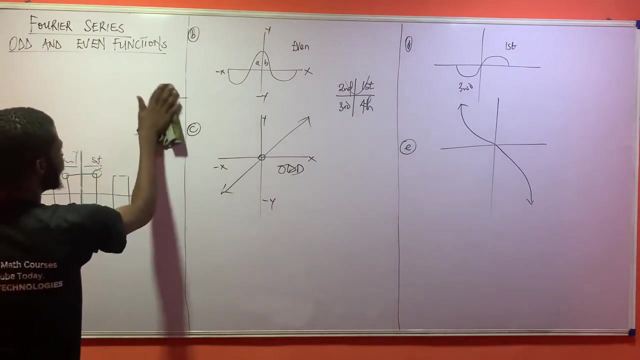 So, as you can see, this guy continues, this guy will still continue. They are passing the origin. So this very guy is what This very guy is: an odd function. The last example for us to recognize functions. the last example for us to recognize functions. 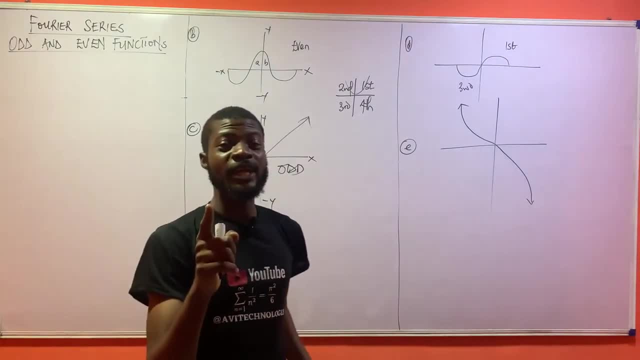 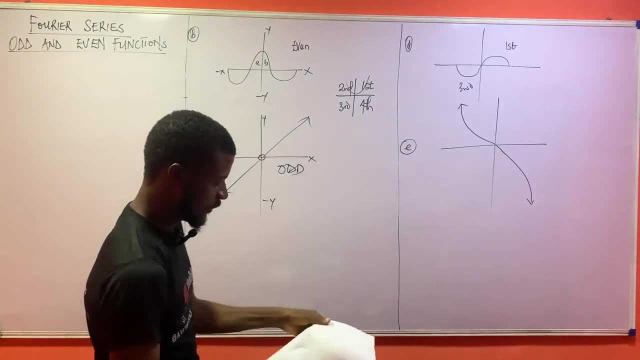 The last example. Now, remember to watch this video to the end, because I will be talking about the Fourier series: coefficients. Okay, Okay, I think I took one question. I think I took one question from the first question. Let us see. 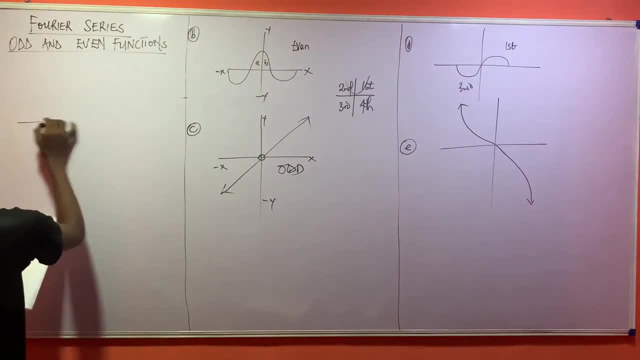 Let us see. I have my x, I have my y. I have this very guy going this way. I have this very guy here. I have this guy this way. I have this guy here, I have this guy this way. Okay, 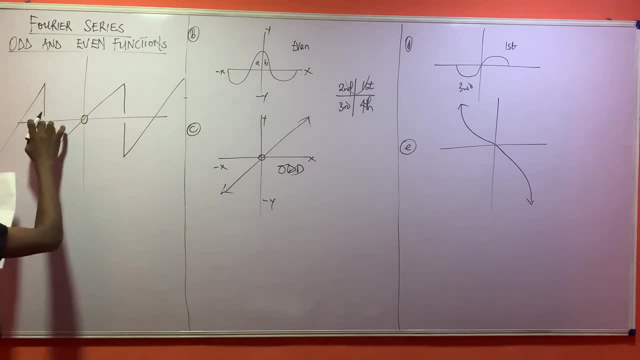 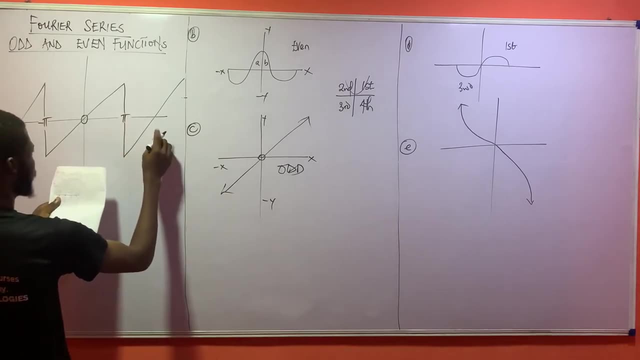 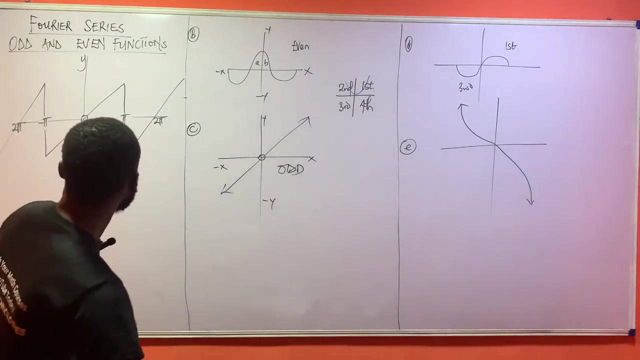 Something like this: This is zero. This is zero. This is minus pi. This is pi. This is two pi. This is also two pi. This is my y-axis, Okay, And we then have dotted lines, or what have you? 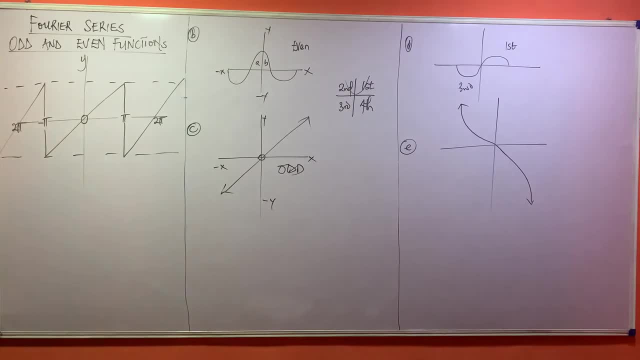 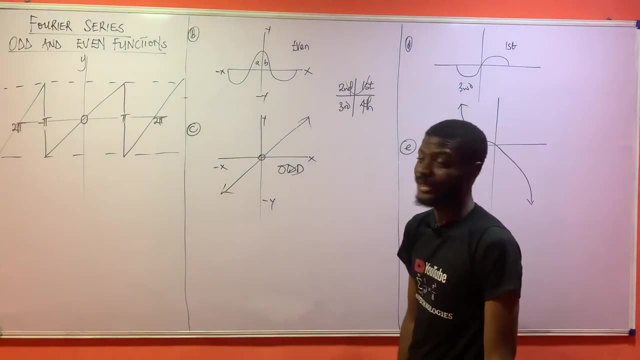 Something like that. And the question is: is this an odd or an even function? Is this guy odd or an even function? Clearly, Clearly. You can even compare it to this, if you want to. You can even compare it to this guy, if you want to. 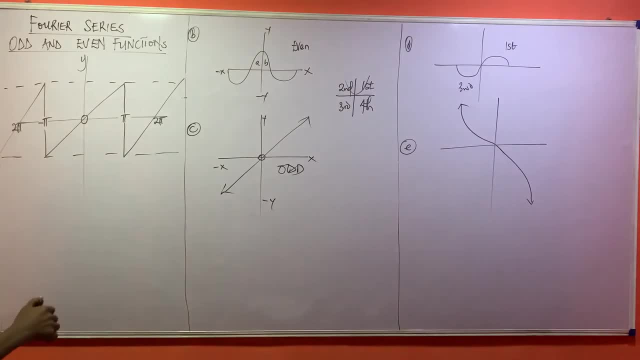 This guy is actually An odd function. Let me tell you why. First of all, I don't even like these dotted lines that they always put. I don't like the dotted lines, Okay, Okay. So this guy, We have this very guy. 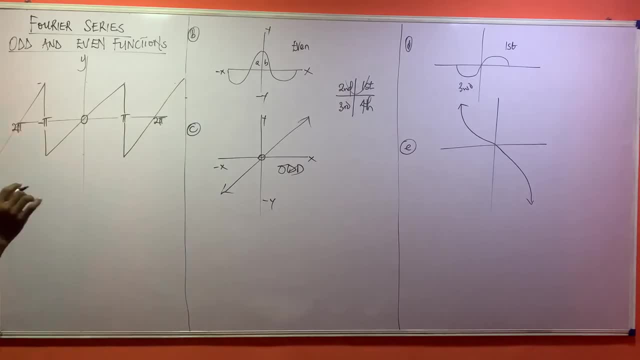 Okay, Now, this is what I like most. Let me call. Look at, Let me assume that it is from minus pi to pi. Now the portion, The portion from zero to pi. Let me call it. Let me call this very area. 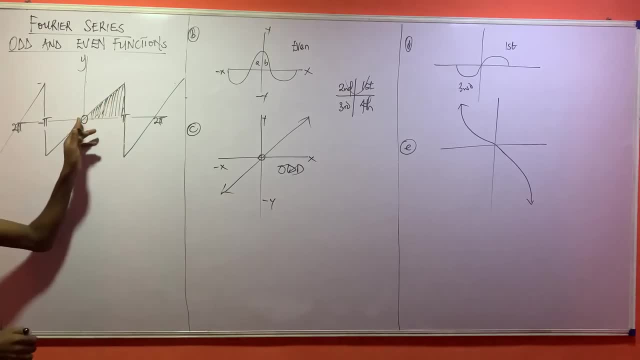 Let me shade it with a black, For example. that's from zero to what Pi. And let me see, I think I have this very color here. And let me call this very other side. Let me call this other side with red. 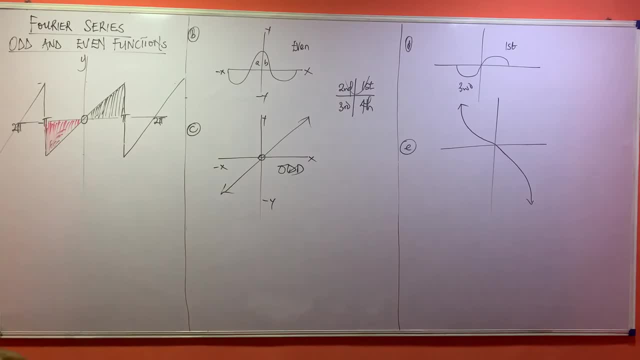 Now, what do you notice here? Very simple: What is at this very side. This is what. What quadrant is this? This is the first quadrant. What quadrant is this? This is the third quadrant. They are having what? The same thing. 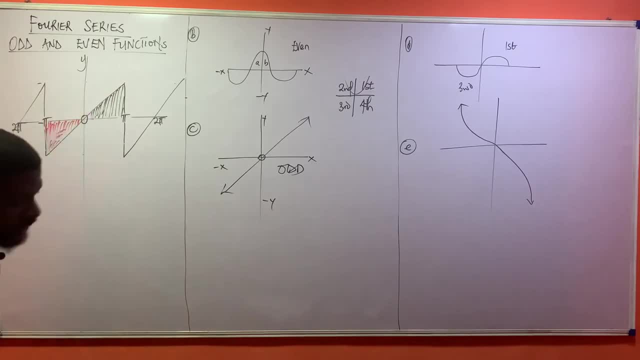 I don't know Opposite sides And it's even passing the origin. Okay, Now what about this very guy here? This very guy is at the what. This is at the second what. Sorry, This is the fourth quadrant. 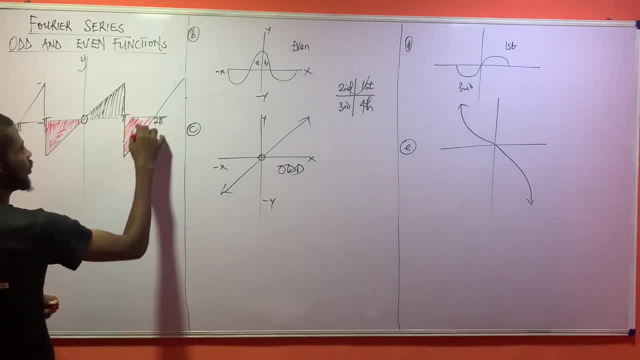 So I have this very guy passing the fourth quadrant. This is the fourth quadrant. Something is passing this very fourth quadrant. Now, what about this very side? Look at this, This very side is here, right? So, as you can see, we are just dealing with what? 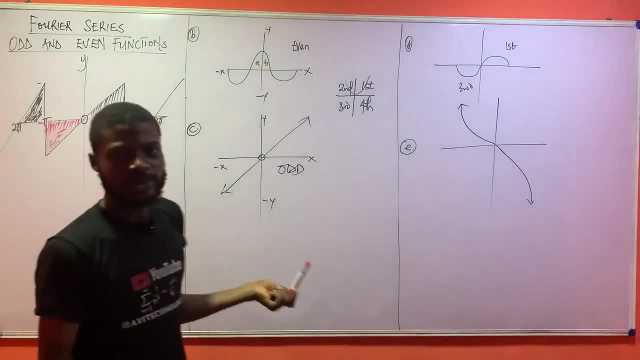 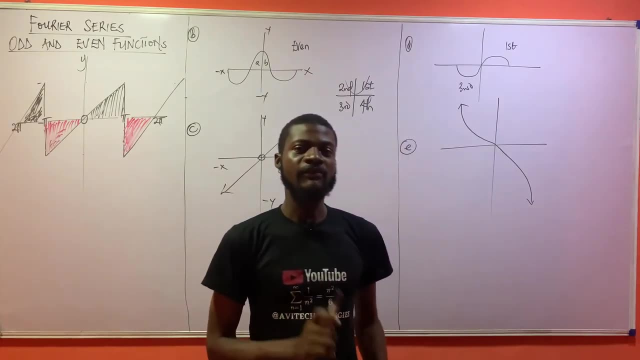 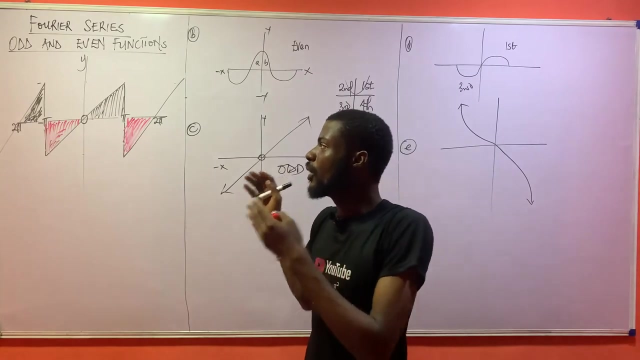 An odd function. This guy is also what Odd. Okay, Now, how do all of these relate and help us in Fourier series? That would be the biggest question You would then ask yourself. oh, what would I use all of this knowledge to do in Fourier series? 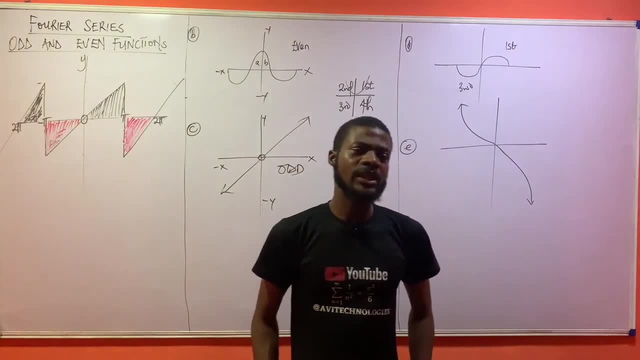 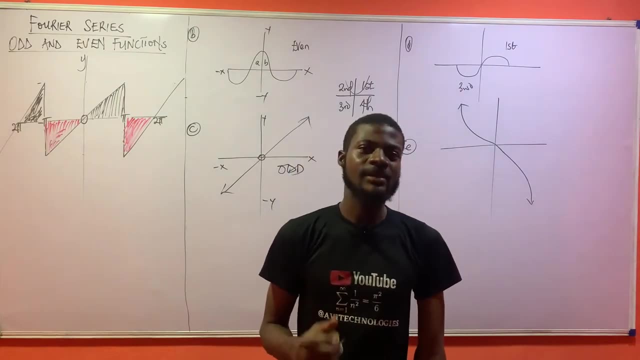 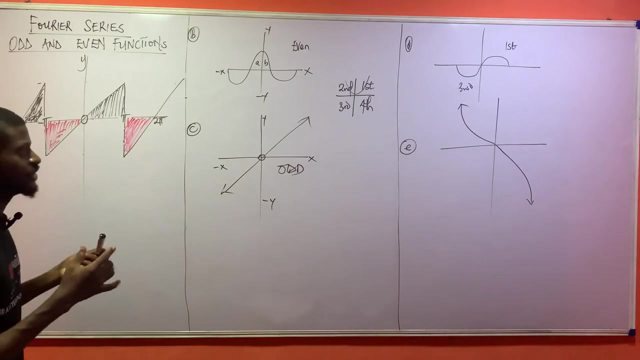 Now remember that Fourier series. actually, in one way or the other, the limits, the boundaries, the interval are symmetrical. Okay, Let me look at this same question again. See, the boundaries are symmetrical. If you notice, the distance from zero to pi and zero to minus pi are the same right? 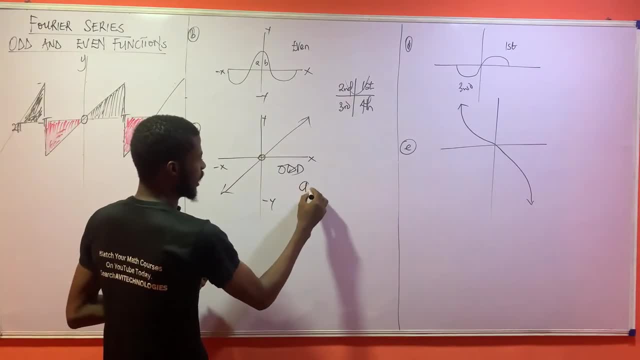 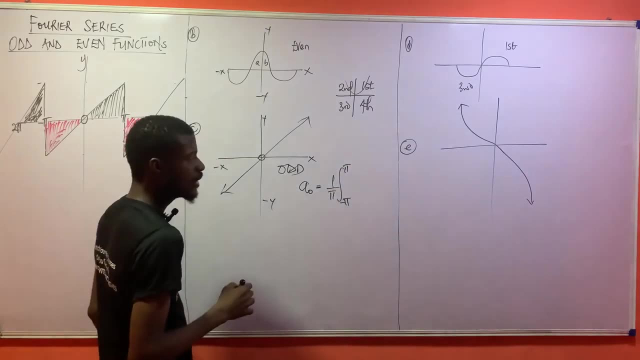 They are the same. And remember that. let me say for a naught a naught, for example, a naught is one over pi, integral from minus pi to pi. right Now, this very interval is called a symmetric interval. 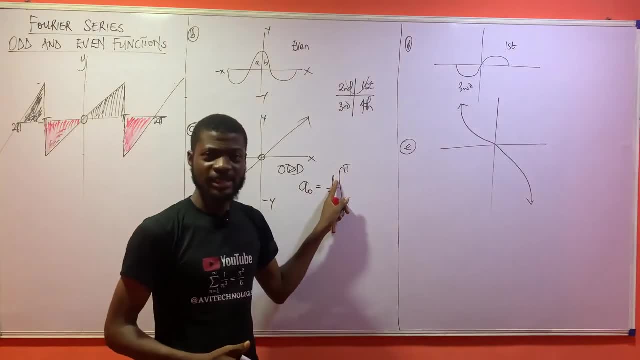 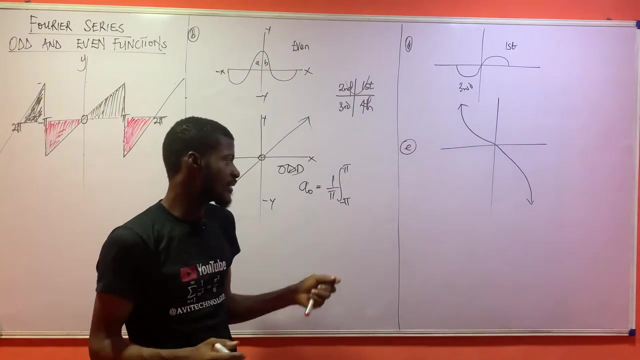 Now, since we are integrating- sometimes it is difficult to do this- We can actually reduce our integration. We can actually reduce how much, how far we integrate, how far we accumulate. Remember, integration is the accumulation of quantities, How far we accumulate these quantities. 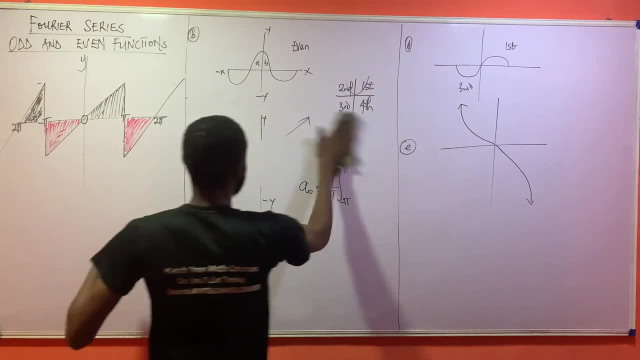 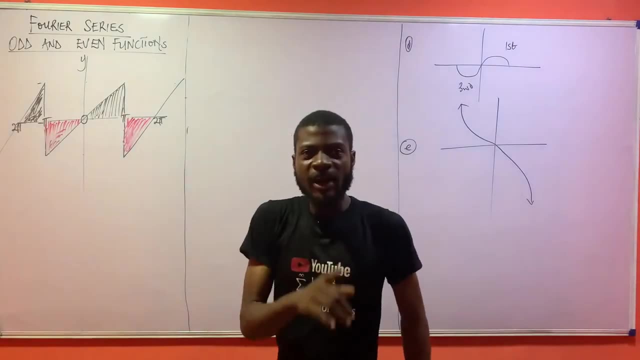 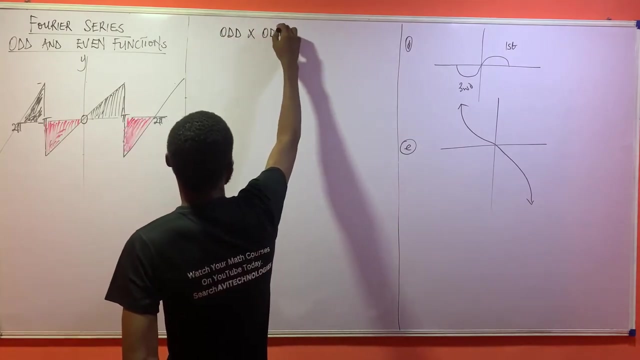 So look at this. Let me not wipe this part yet. Okay, We're going to do something very sweet right now, Before I go, before I proceed. an odd function times an odd function. What function do you think that will give to you? 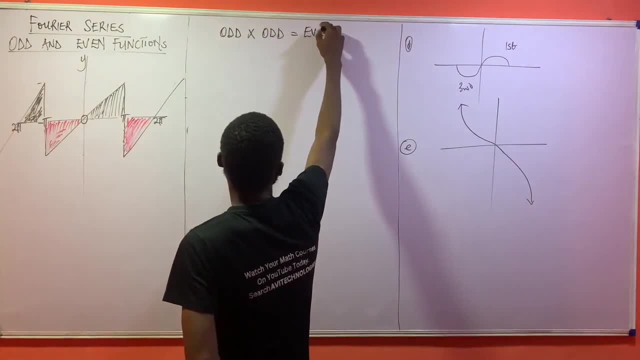 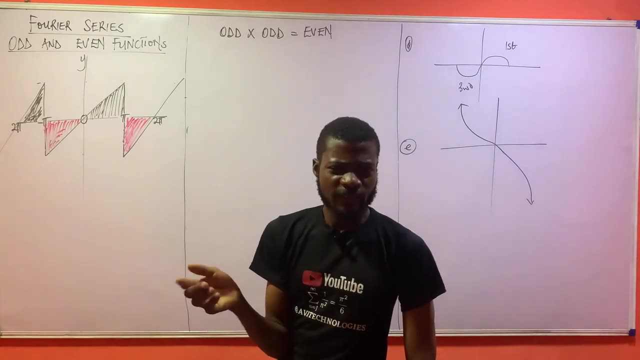 This will be giving you an even function. Now, please, I'm not talking about numbers. I know what your brain is doing. right, Your brain is doing three times five. fifteen, Fifteen is odd. now, Then why did I say even? 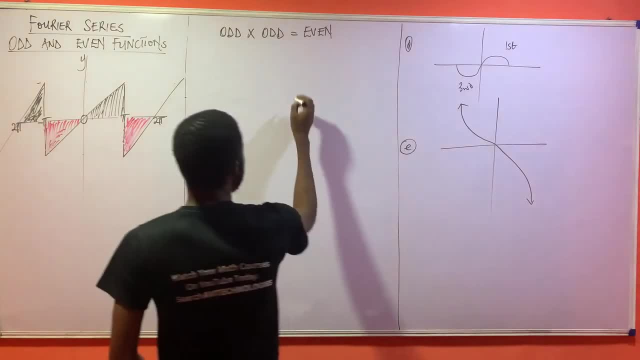 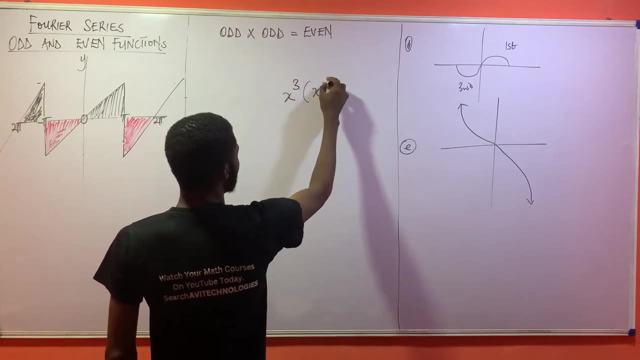 Please, I'm talking about functions here. Functions, Imagine if you have s squared bracket s. Sorry, We're talking about odd Right S to the power of three, bracket s to the power of five. What would you do here? This is s to the power of, since it's indices, I would say three plus five, eight. 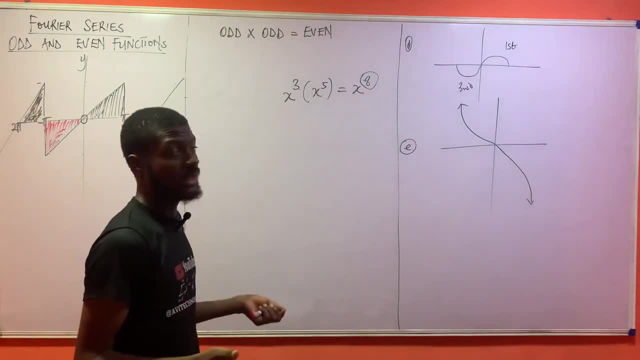 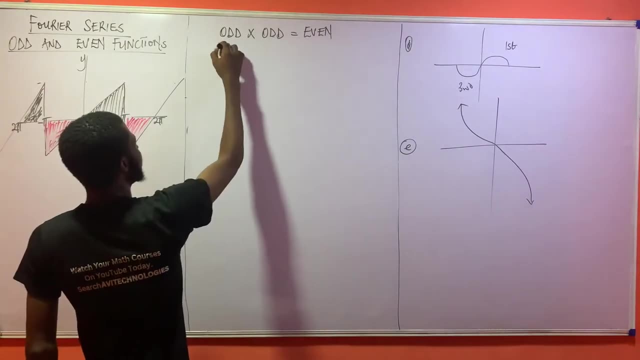 This guy is what? Even So, I hope that is now clear to you, that this guy is even Okay. So let us proceed Now. what about if somebody says we have odd function times, an even function? What are we going to be getting? 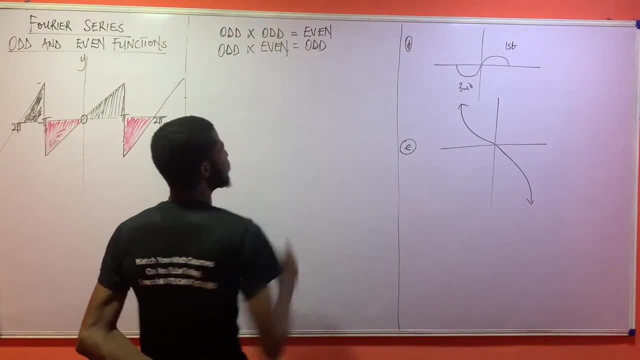 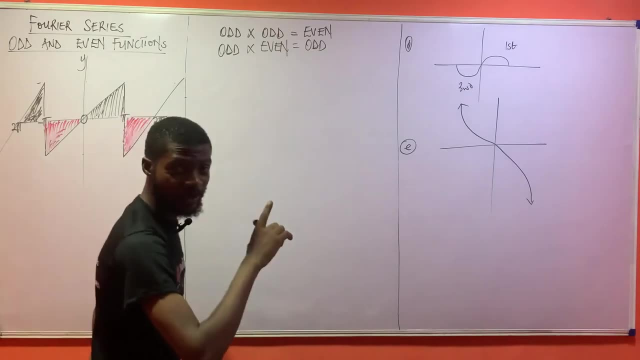 This is going to be giving me an odd function. That is very, very understandable. Now what about if I have? I hope you know why that's an odd function, Or do I have to explain that guy again? It's also an odd function. 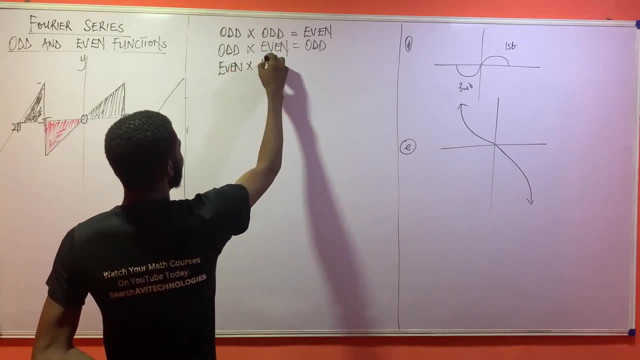 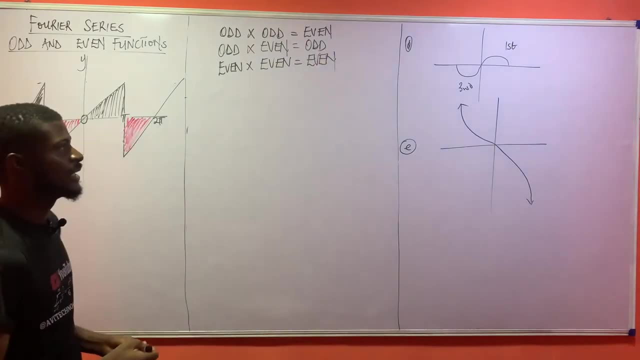 Now an even function times another even function is going to give me an even function. It's going to be giving me what An even function. Okay, Let us see. I think this guy should be much more okay. Okay, So let us see and let us get started. 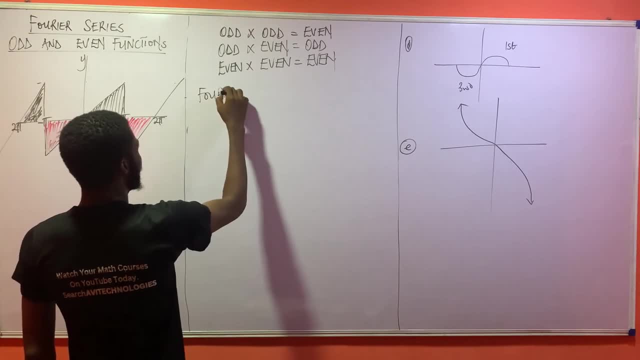 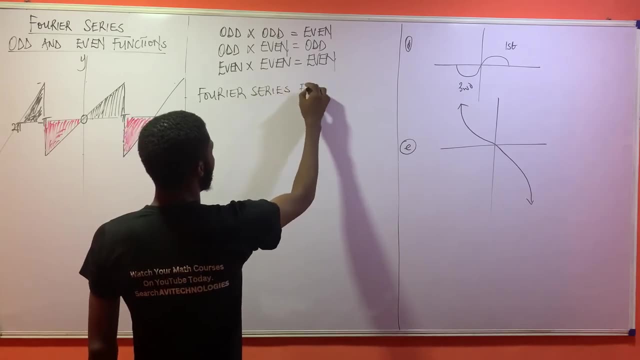 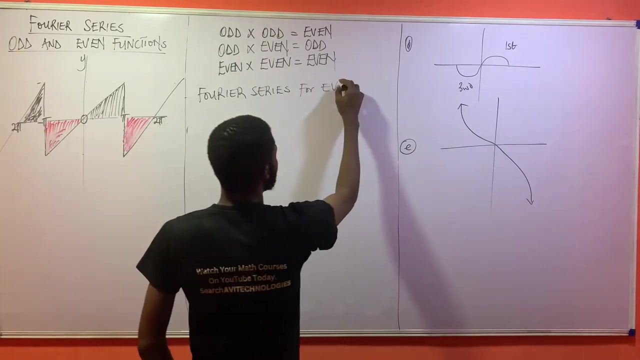 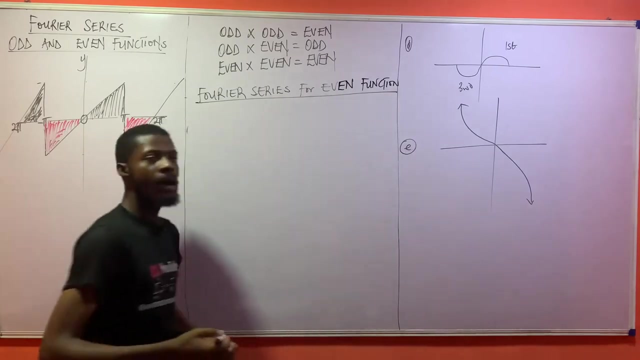 Okay, Fourier series, Fourier series. Fourier series For even functions. Fourier series for even functions. Let us discuss about the even functions first of all. Okay, Now, how would this be looking like And how are we going to have this? 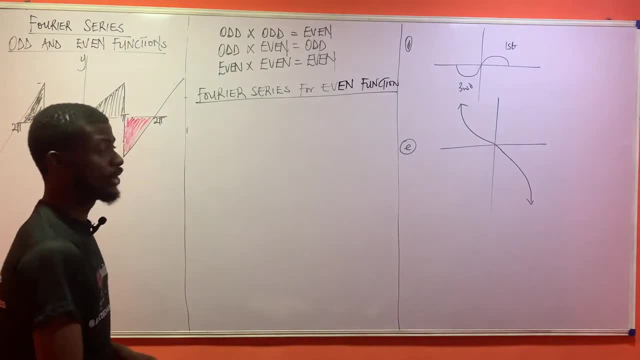 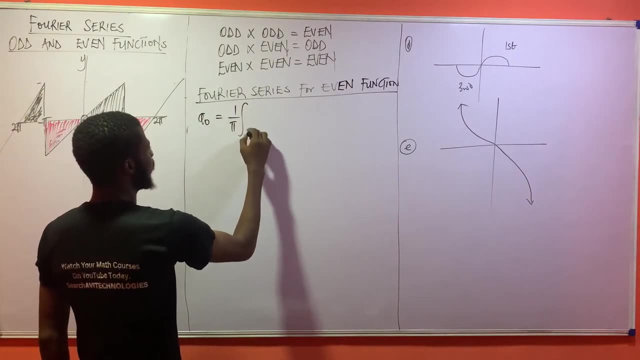 First of all, Let us talk about. Let us talk about A naught, Let us talk about what A naught Formula for A naught is: 1 over pi, Integral from minus pi to pi of f of s dx Right. 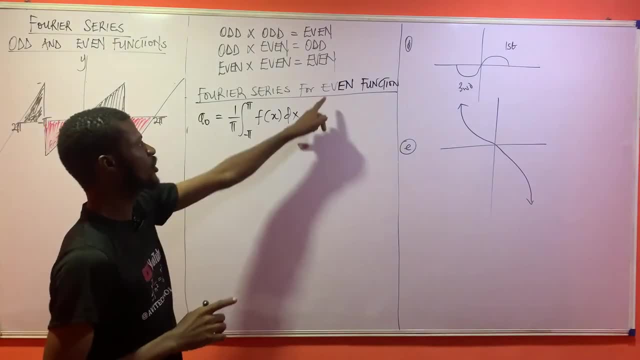 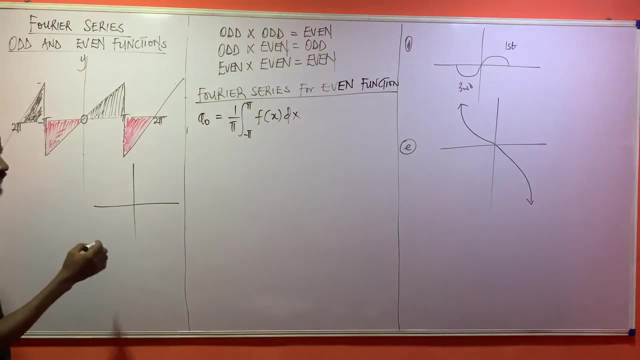 This is the formula. Now, if a function is even- Please take note, Let me draw it here. I'm going to be drawing something very small- If a function is even, Let me say I have something like this, For example, something like this: 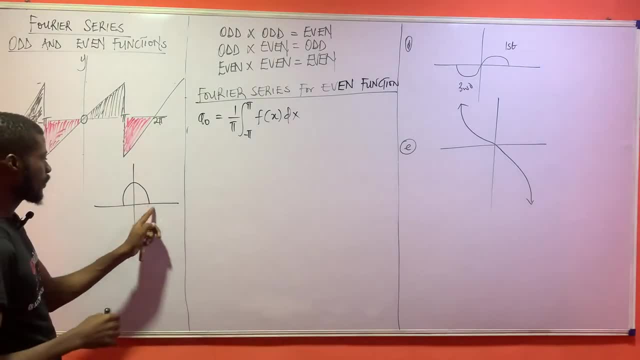 Now look at this, Look at this carefully. Look at this carefully. The value here, or the area under this very graph A, under this very curve A, is the same with the one under this very curve Right Is the same. 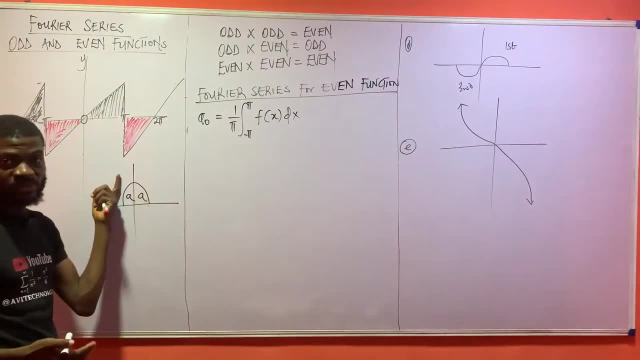 Because remember that I said it's symmetrical. So whatever you have here is what is here also. So A plus A will give me 2A Right Now. see, This is your pi. This is zero. I think this is too small. 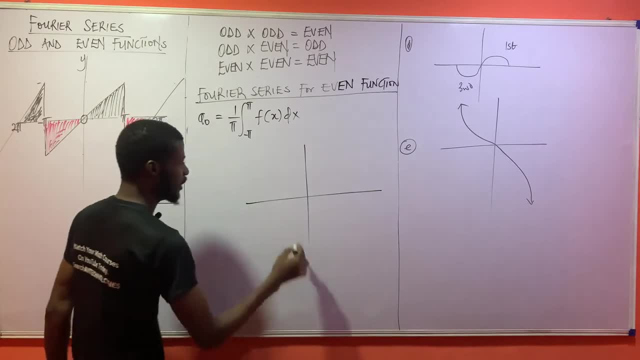 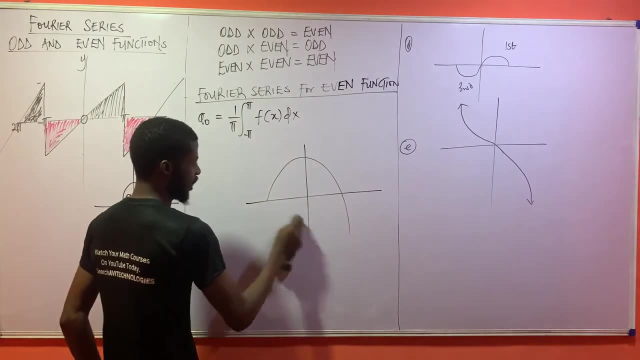 Let me explain this, Because I love doing things very big. Let me say I have something like this: Okay, Even though this is looking very unprofessional. Okay, Now imagine if it's an imagination. I did not really draw to scale. 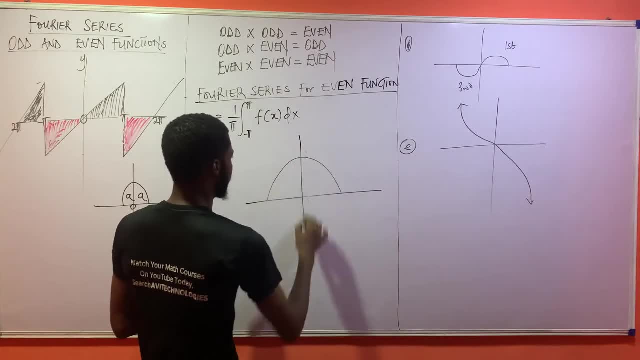 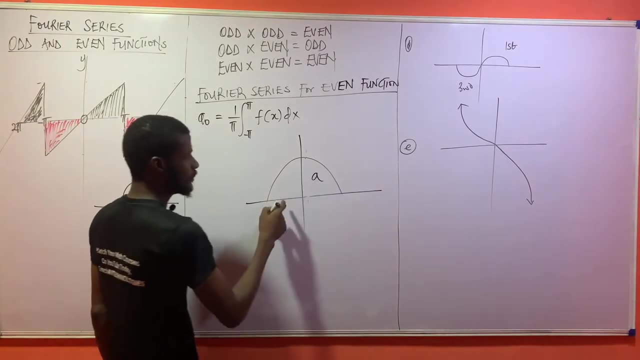 So imagine if this very guy is an even function. Whatever area you have here. Let me say, the area here is E. It's the same area with this other side E, Because they are actually the same size. So if this is zero, this is your pi and this is your minus pi. 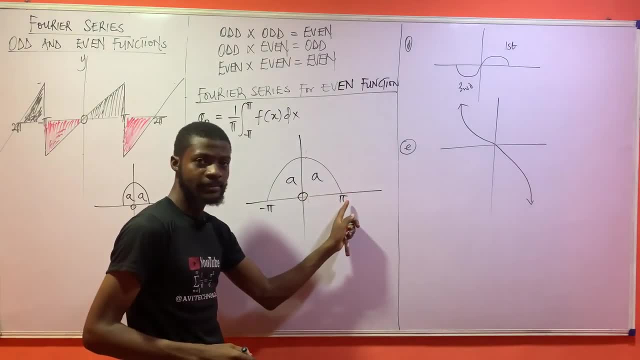 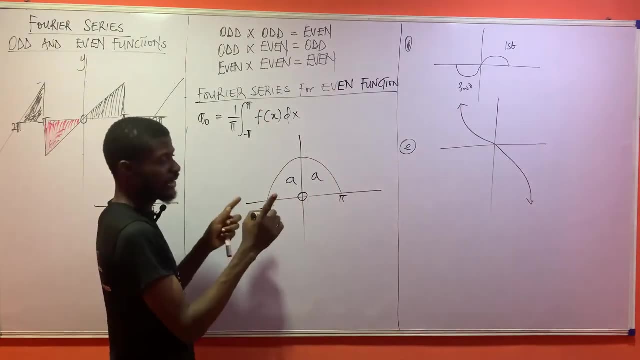 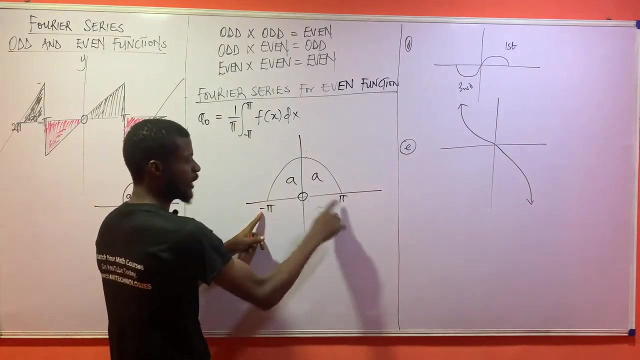 From zero to pi. the area from zero to pi is the same with the area from zero to minus pi, So instead of me to start integrating from minus pi to pi, I'll be spending time integrating from minus pi to pi. It's stressing me: from minus pi to pi. 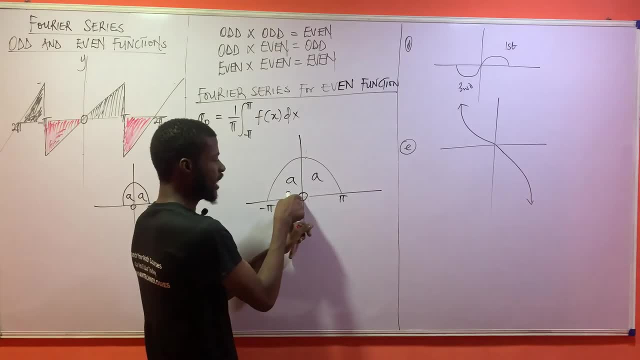 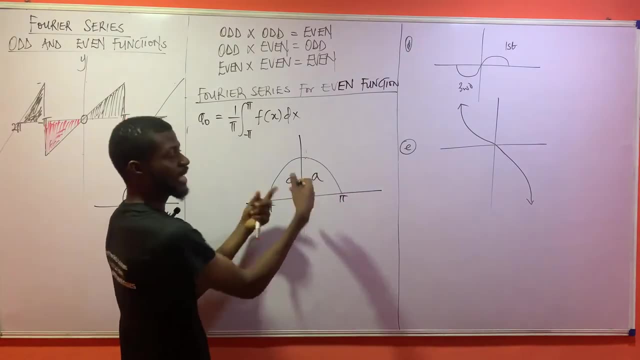 Why would I not just say, oh, let me integrate from zero to pi instead, Then double the answer, Because these two things are the same. If you can get the value of this one, I will just times by two, And obviously I've gotten everything. 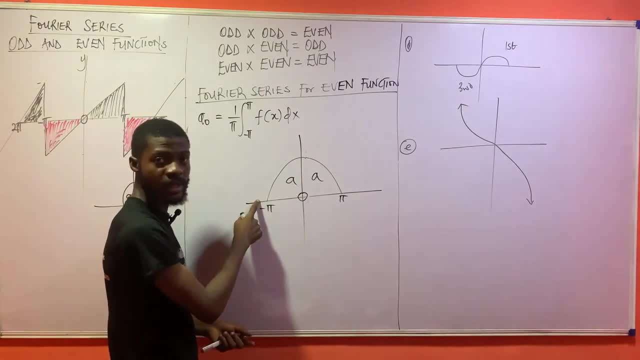 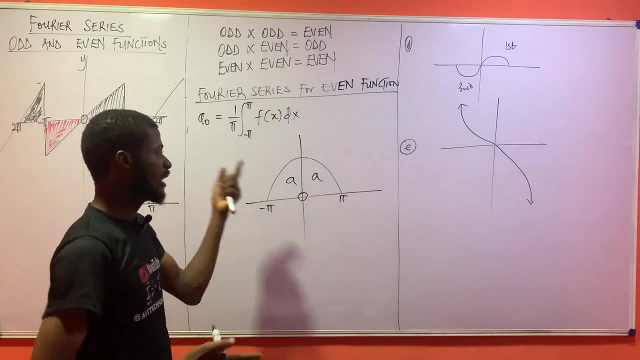 Because if here is E from here to here will then become 2E. So if you can get the value of this first part, this very part, all you have to do is to double your answer, Because in an even function, these two sides are the same. 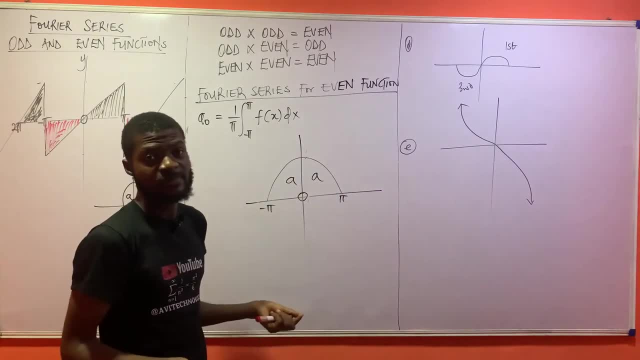 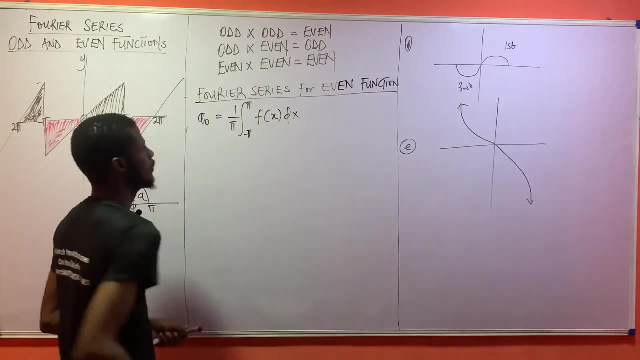 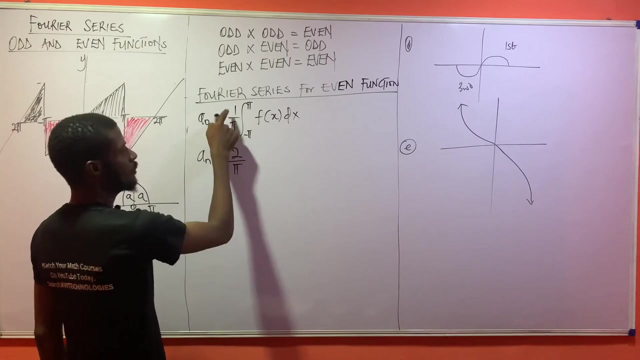 So you can calculate for one side of it And to get the total of it you just times by two, Because I have two portions. So that means That your A naught can be reduced 2 over pi. You know why it's 2?. 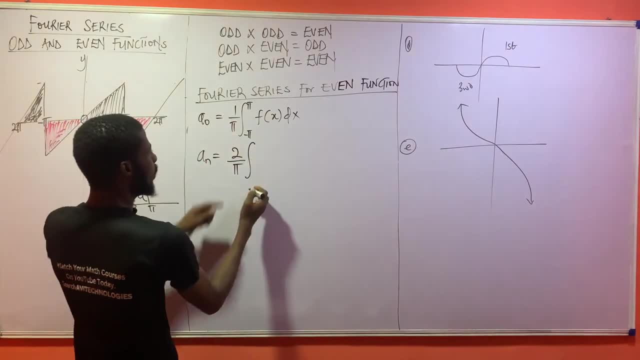 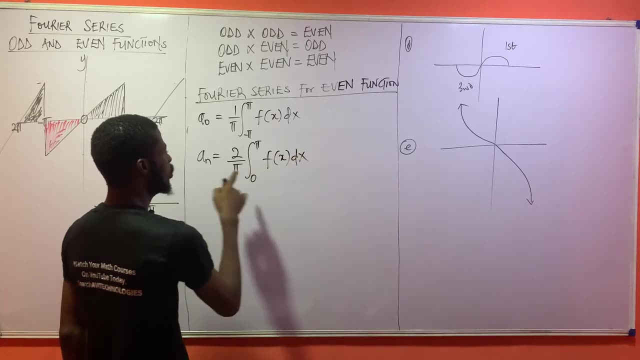 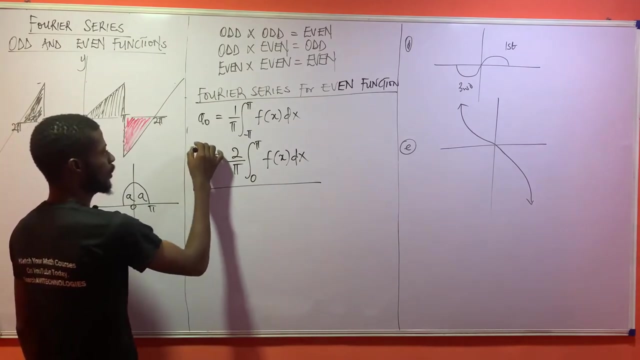 Because you are timesing by 2. Integrate from. I will no longer integrate from minus pi. I will integrate from zero to pi f of s dx. So this will then become your new formula for A naught. This will then become your formula. 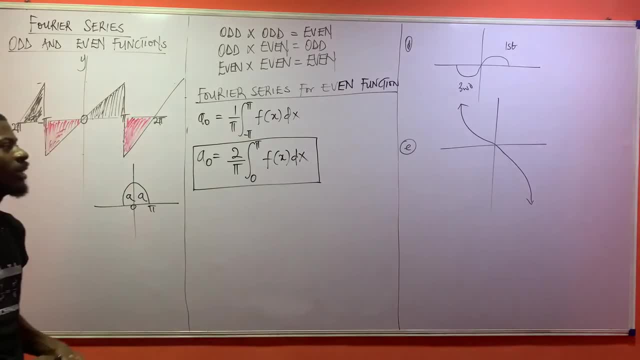 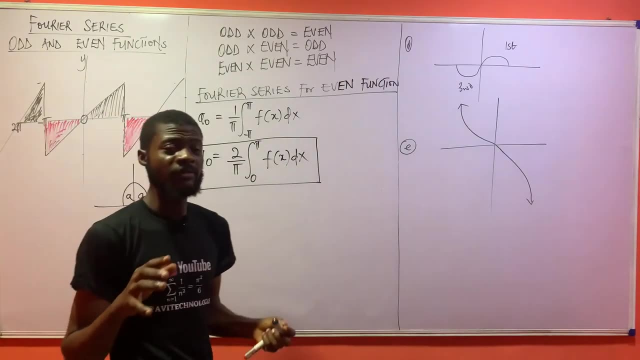 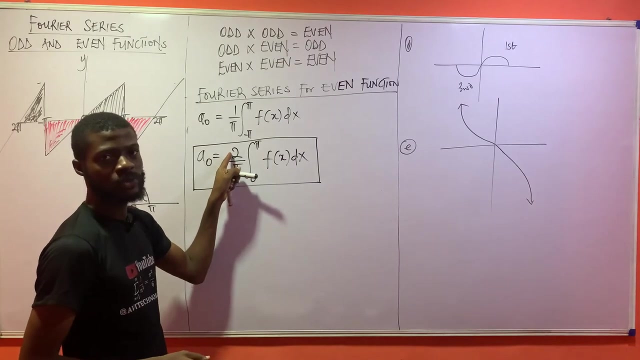 For what A naught. Very beautiful and very, very interesting. So this is what we have Now in the comment section. I believe a particular person was asking for this very guy. A person was asking: when does it become 2 over pi? 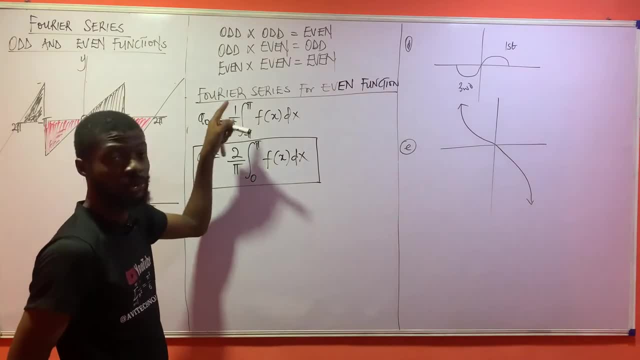 Okay, So I was thinking that he was asking when, if the limit are not going to change. actually, Right now, this is the perfect answer for him. So if this is 2 over pi, your limits are also going to change. 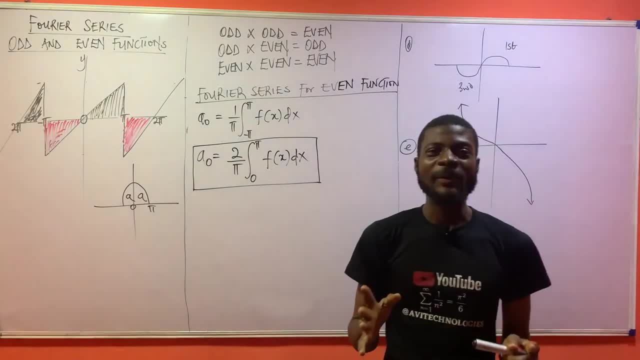 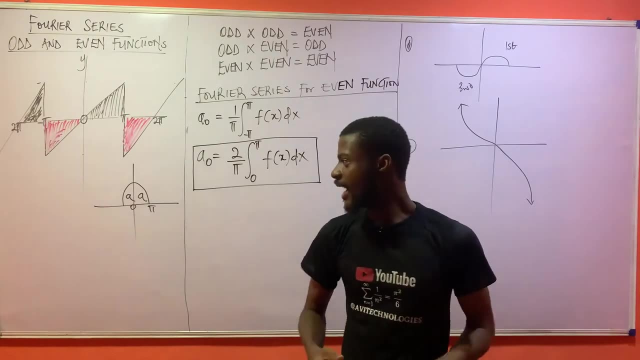 Now I noticed something. You guys are going to help me play with the girls All of my videos. they are all boys that are watching them. They are all men I have not had. Okay, maybe one day I will reveal it to you. 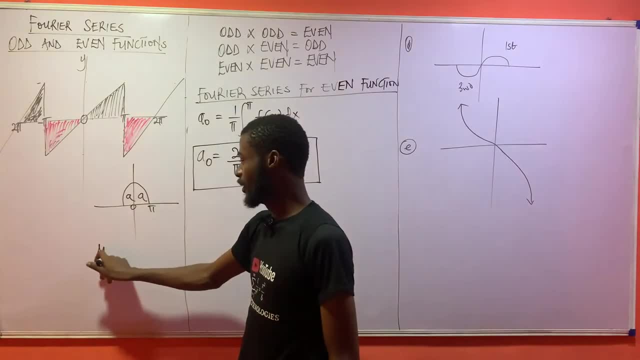 In my studio. if I go to YouTube, I will see male, I will see female, Then obviously I will see unspecified. Now, when I am talking to the male, 100% are going to be there Because you are going to be. 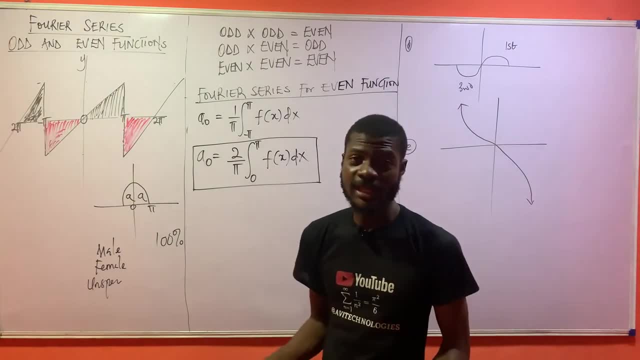 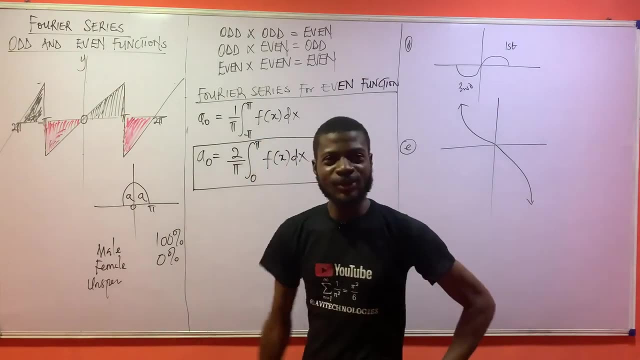 They are going to show you the percentage of viewers according to sex: Female: 0%. And I am like: are you serious? So you mean that girls don't watch my videos? So please help a girl out there, Share my video to girls please. 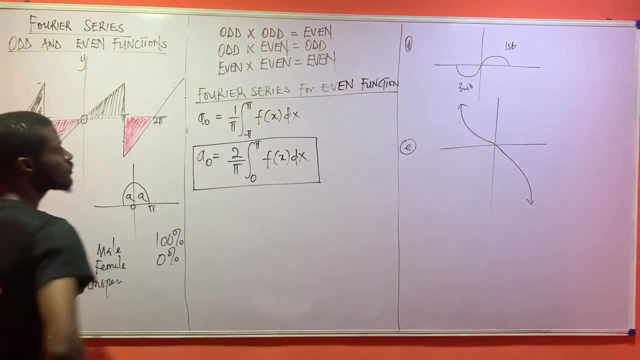 Okay, Meanwhile, let us continue. Let us continue Now. see, After a nut, what was the next one? A sub n. A sub n. A sub n. Now, what am I going to do here? I am going to say: 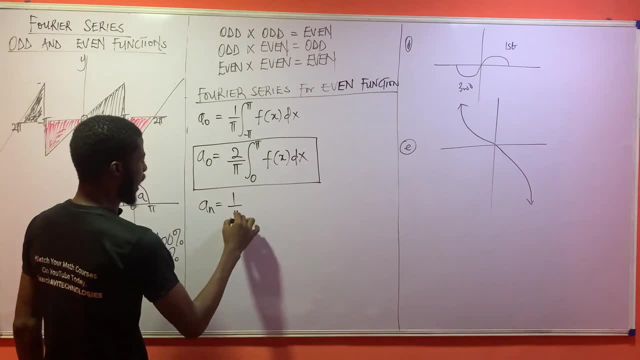 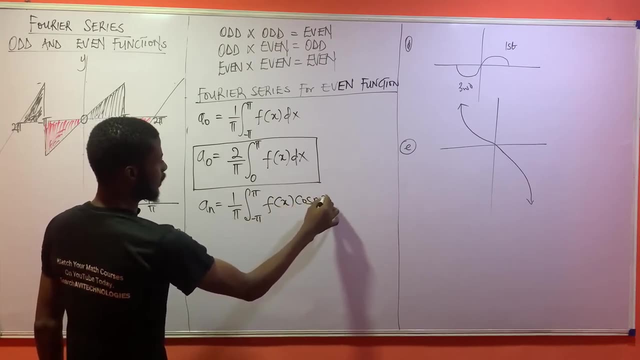 A sub n. A sub n on a normal day is 1 over pi Integral from minus pi to pi. F of s? cos nxdx. Okay, So this is your, what? This is your a sub n. Now look at this. 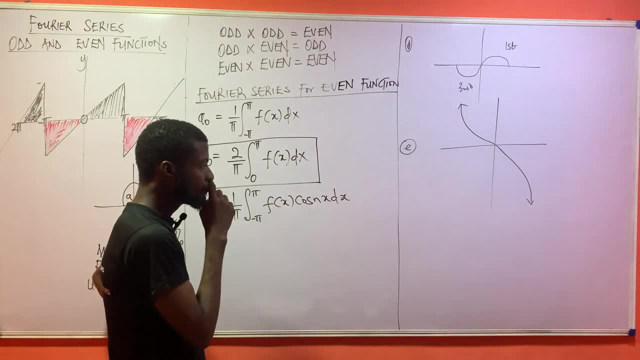 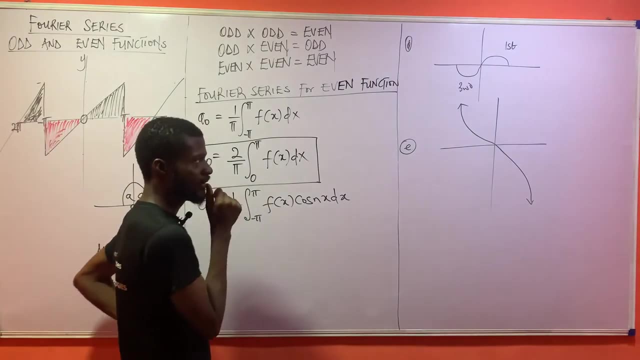 Careful, Be careful. Have I drawn a cosine graph before And did I tell you it is a cosine graph? Because you have to first of all know what a cosine graph is. Now, please take note. This is what a cosine graph looks like. 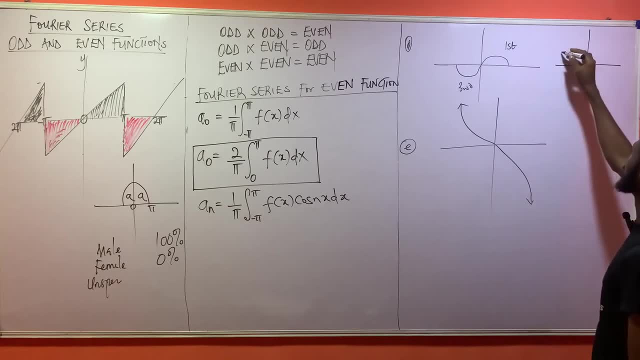 Cosine is an even function. So this is what a cosine graph looks like This very guy. So it looks like there is this cosine graph. Why this very guy is a sine graph. This is a sine graph. Why there is a cosine graph. 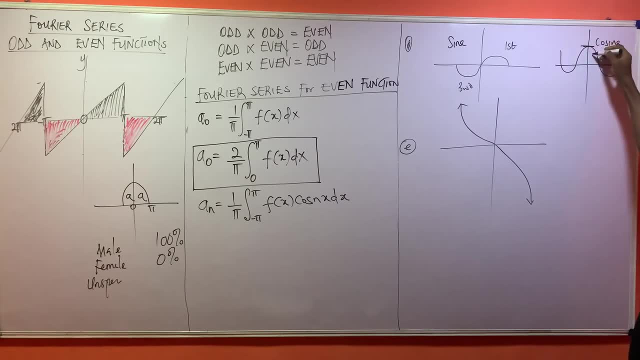 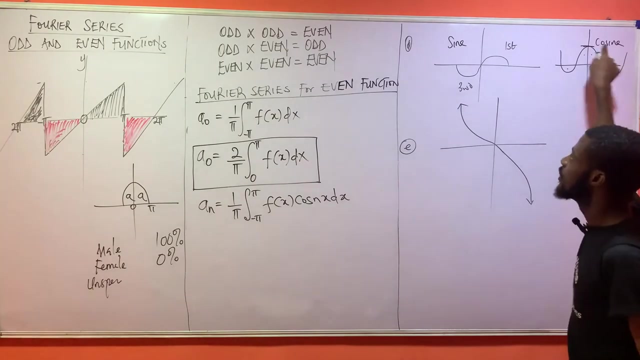 Simply because you can see that this guy, Oh, this guy- is actually. This part and this part are actually the same. This part and this part are actually the same. So this cosine is an even function, sine is an odd function. repeat after me: cosine is even, sine is odd. now see, 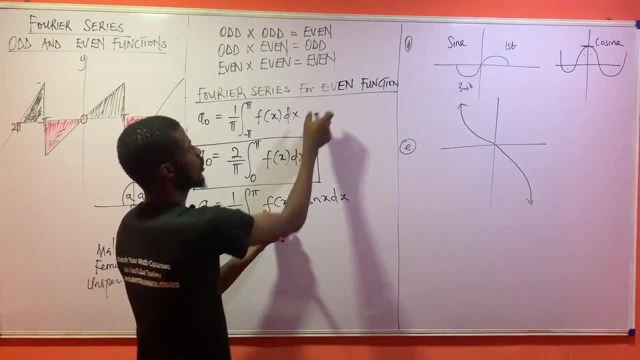 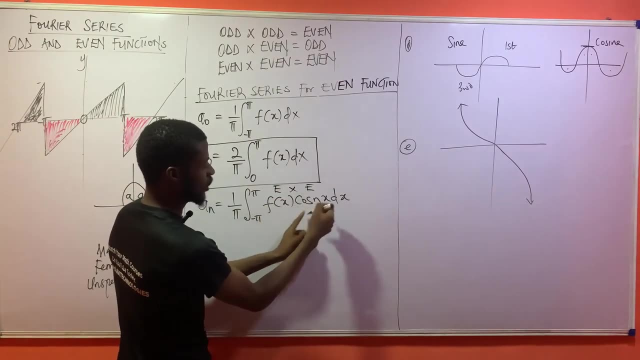 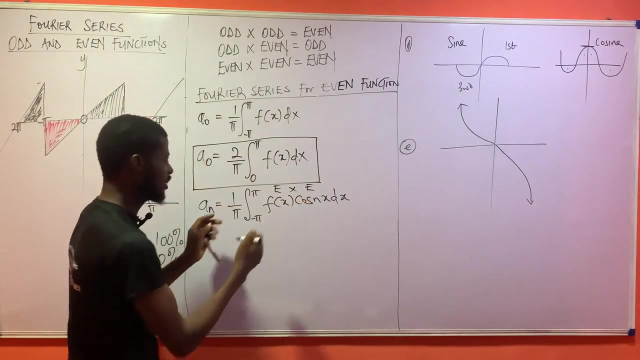 we already said that we're discussing only even functions here. so if f of s is an even function, even times another even because cos is even even times even we give what an even function. so what does that mean? i can reduce this very integration. i can say a sub n is equal one over pi. 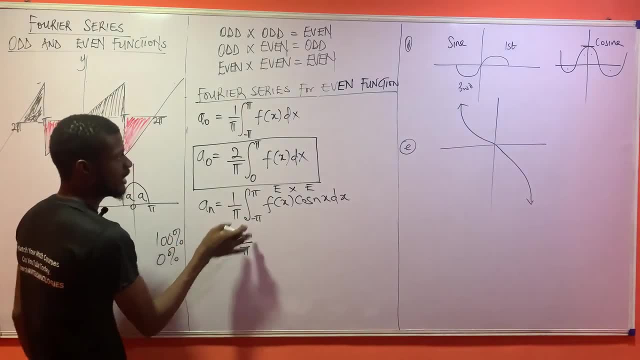 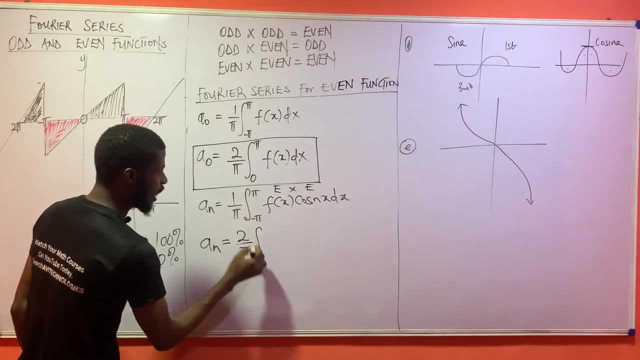 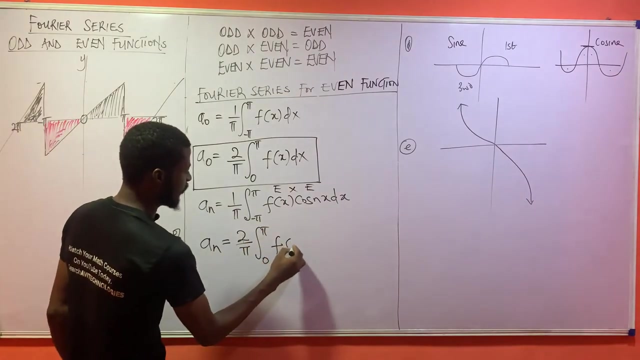 times two, because you know i've already explained it before here, so no need for me to do that again. clock time: now. we say two over pi, integral from what zero to what pi. i've changed the limit, the lower limit, to zero to pi, then f of s, cos, nx, dx. please take note. 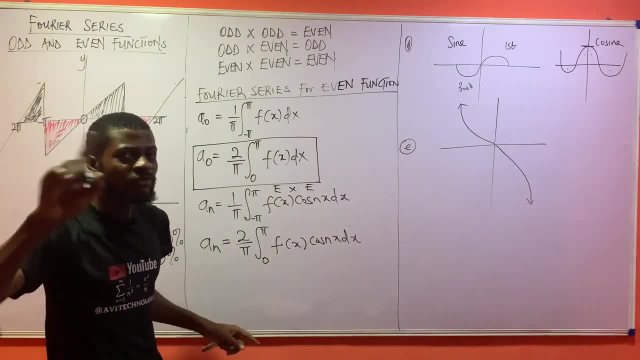 you can't change the limit, you can't change the number of times, because this is an even function. You always say two times when it's an even function. I will tell you what happens when it's an odd function. You will see that briefly. 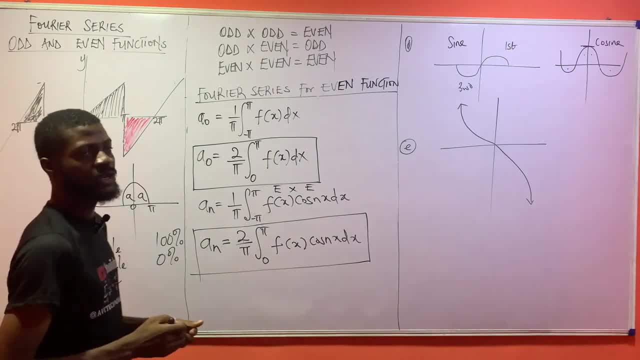 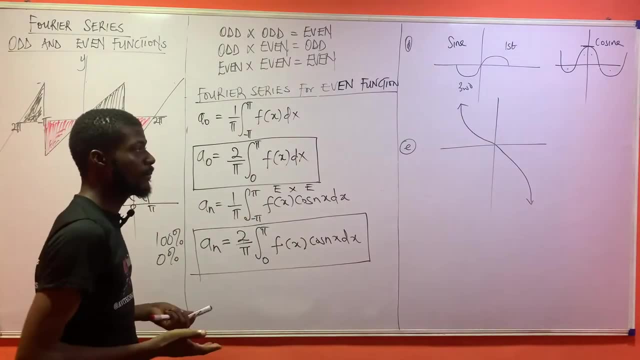 So this formula is going to hold. So instead of us integrating from minus pi to pi, we can just integrate from zero to pi and double our answer. It's much more easier for us to solve. It's much more better for us to solve. 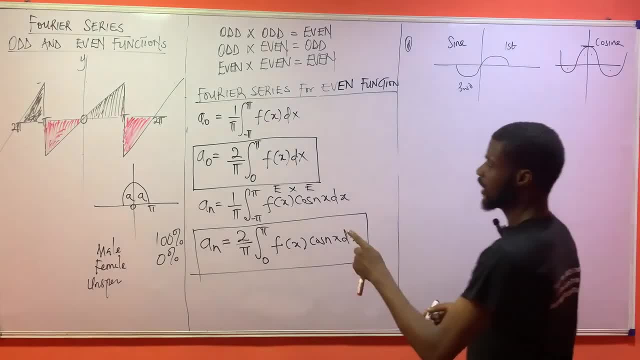 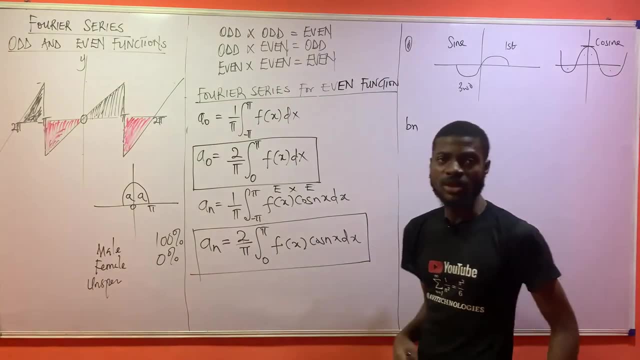 Okay, And let us proceed. The next one is b sub n, Because obviously Fourier series coefficients, we're going to have three things: a naught, a sub n and b sub n. Now this is 1 over pi. 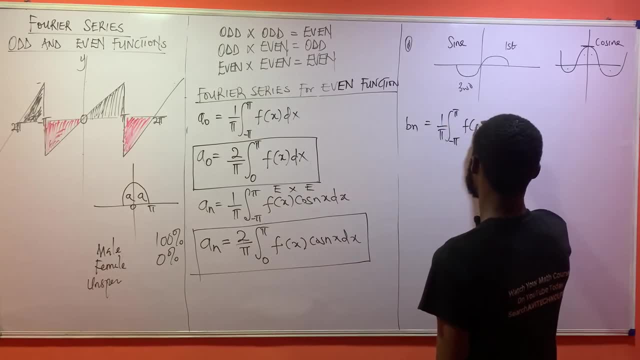 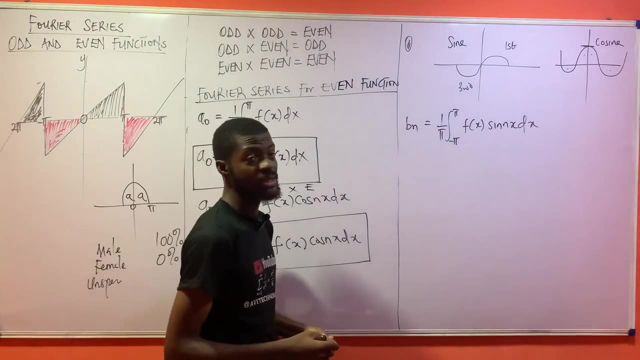 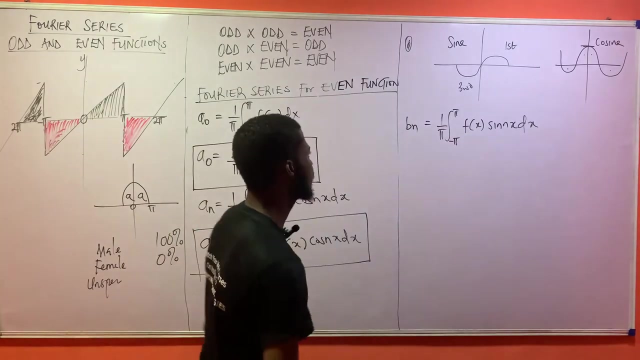 integrate from minus pi to pi f of s sine nx, dx. So if this is what I have, if this is what I have, for example, how do I know This product? what will this product give to me? Look at this. 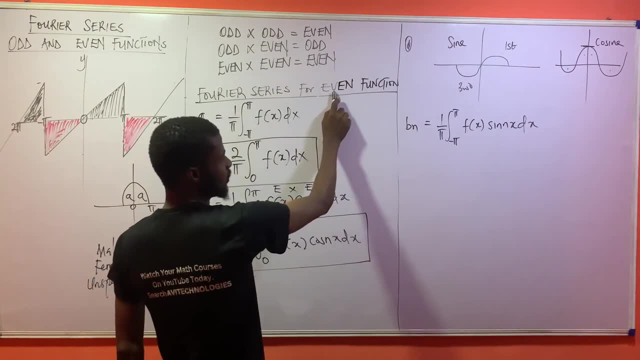 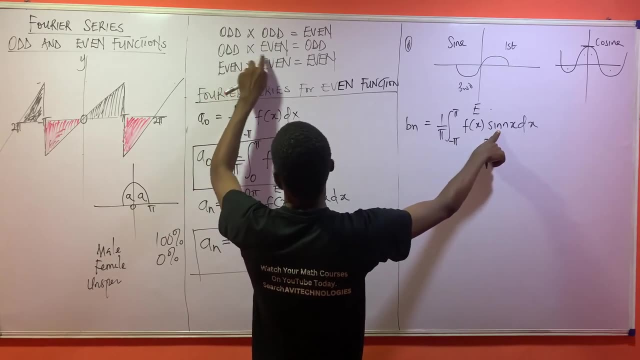 We already said, f of s is even Because we're discussing even functions. An even function, times sine is odd, Even times odd. Even times odd will give me what Odd. So that means this thing here is an odd function. And how would the graph look like? 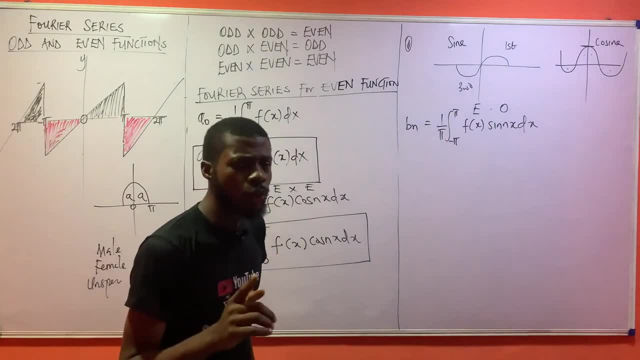 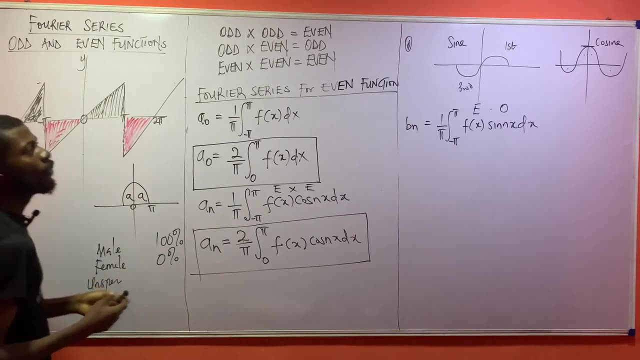 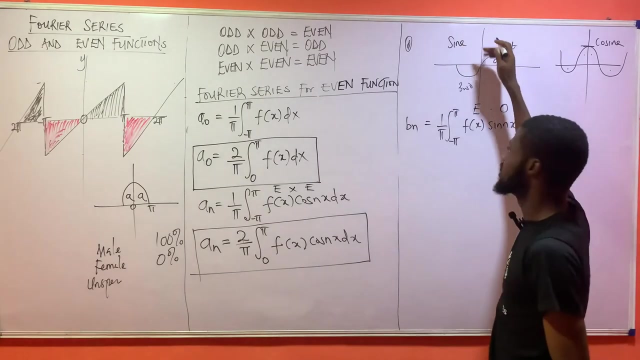 This is how the graph would look like Now. are the areas the same? No, When I was solving here, I said: the area on this part and the area on this part are the same, But in an odd function, please. the area on this side is a. it's positive, it's positive. 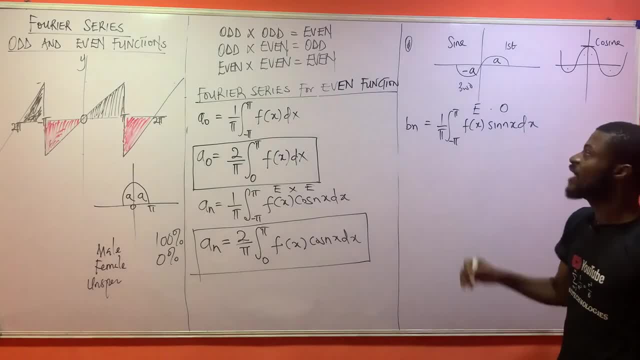 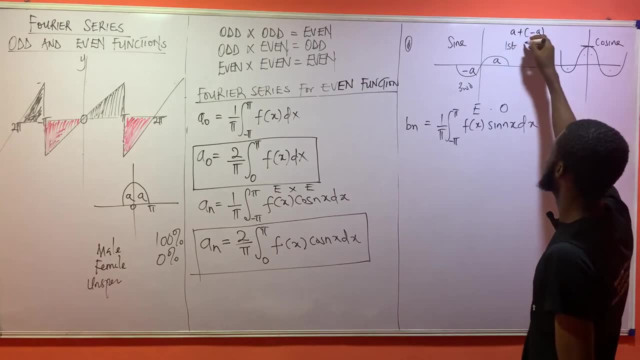 The area under here is: what Minus a? Now, if you should sum up these two things and say you want to plus them, if you say a plus minus a, this is a plus, minus is minus a. so all this a gives to you zero. 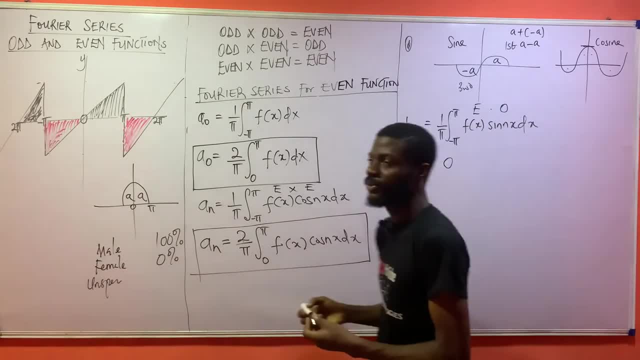 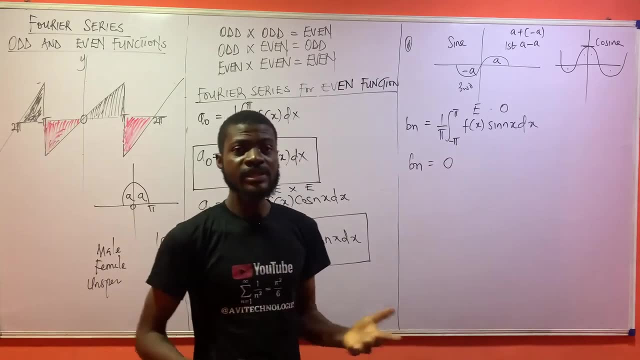 So it means that your b sub n is equal to what Zero, And that is why, many a times, when you are solving some questions, you find out that your b sub n is equal to zero. Simple, Simply because your function is an odd function. 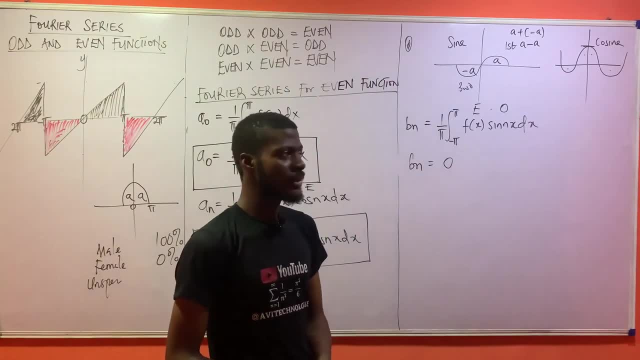 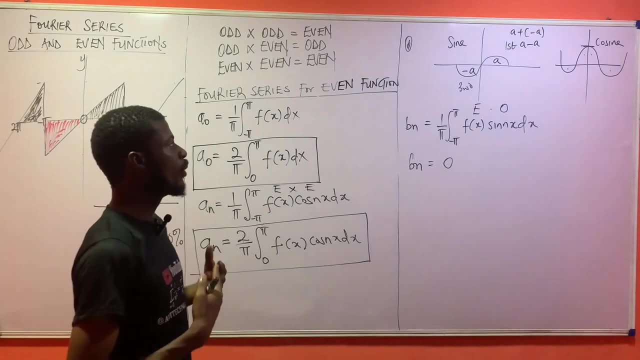 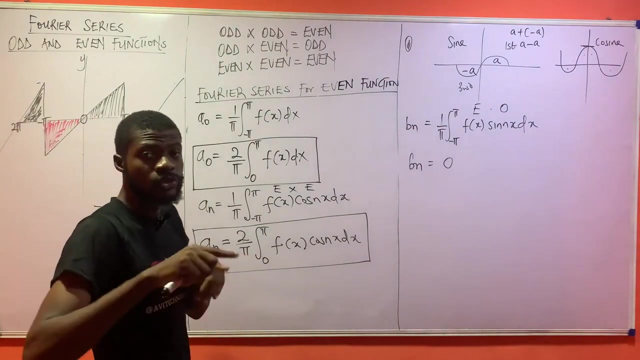 No need for you to really stress yourself. in some cases, If you are integrating this guy over an odd product, your b sub n is zero. Now what does this result tell me? They are trying to show me that you cannot and won't. sorry, let me get the right sentence. 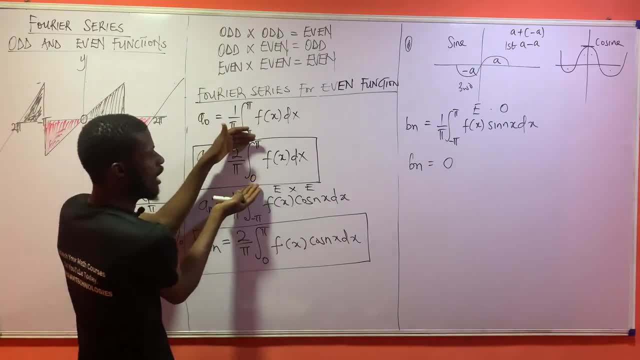 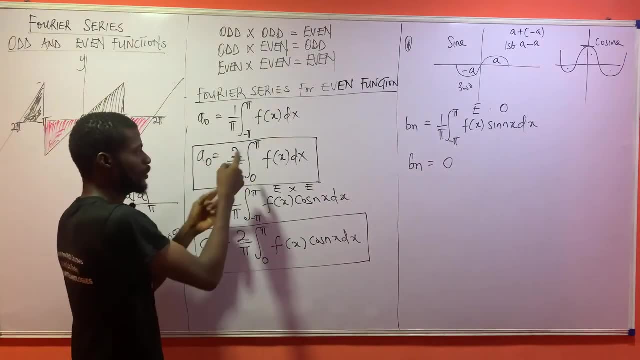 You will not only be able to reduce by how much you integrate or the boundaries, because we have reduced the boundaries, yet We have reduced the limits. You cannot only reduce it, You will not only reduce it, but it is going to tell you that. 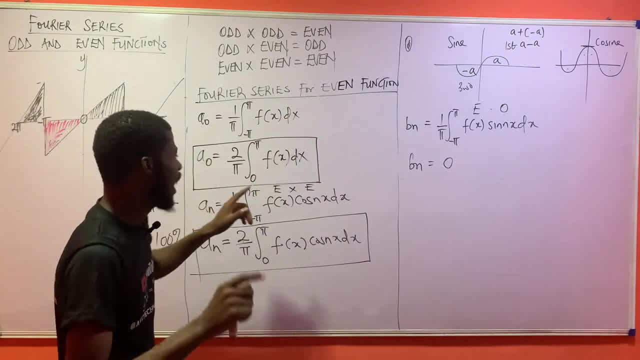 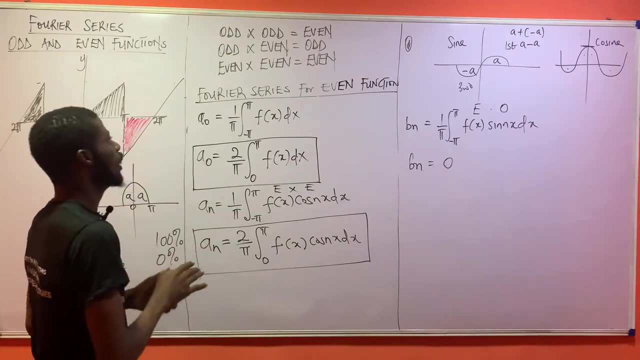 oh, since it's even, I only need to find a naught and a sub n. That is what these very formulas are telling you, That, oh, not be saying. oh sorry, I don't know. I want to speak, Pidgin. 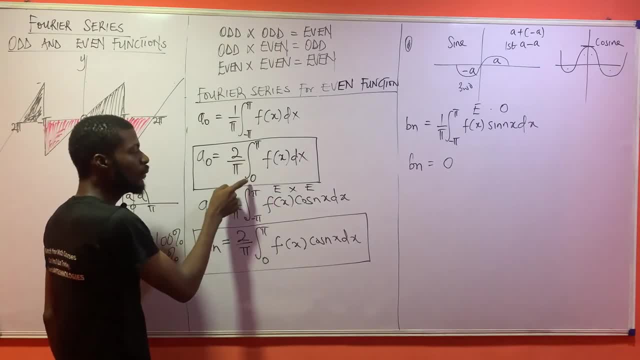 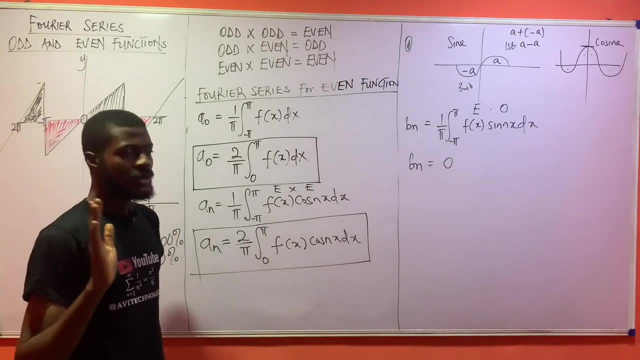 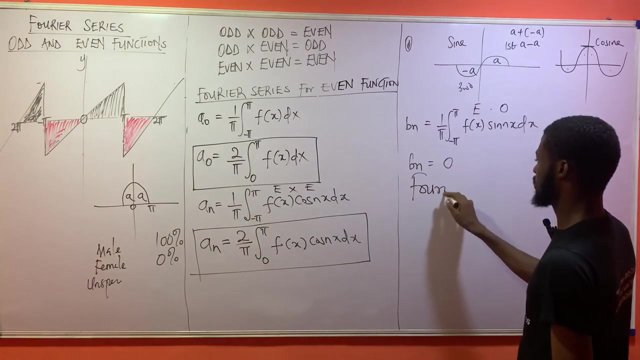 but not be saying: only this one will fit well. We have different benefits. We have reduced the integral and also reduced the things we are supposed to solve for. So this is where this guy is very, very important. Now, what about? we're talking about Fourier series. 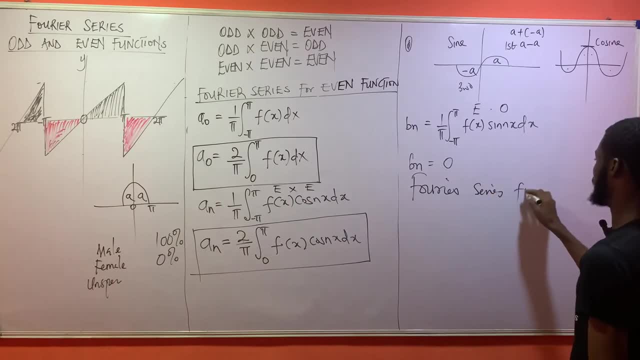 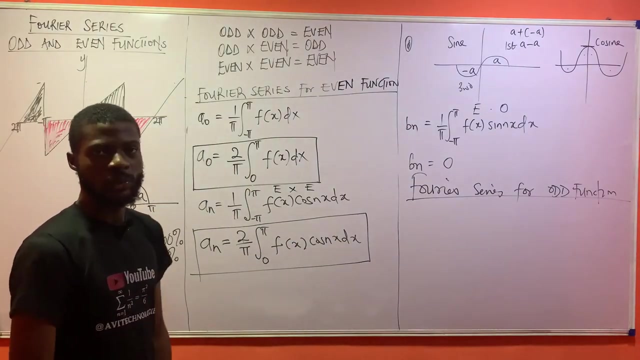 the Fourier series for an odd function for an odd function. Now, how do we do this guy The Fourier series for an odd function? How do we go about this? Well, I do not really want to waste time because we're close to the end. 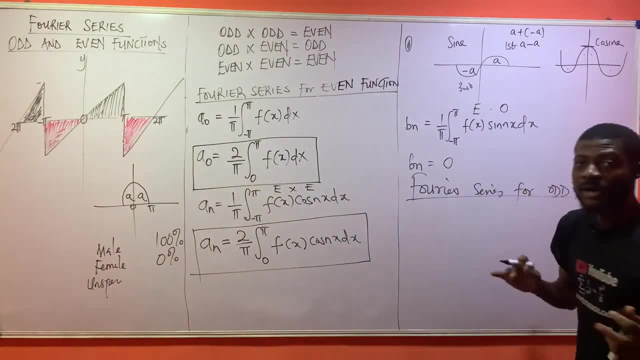 We're close to the end of this video. Now see, the first thing I'll do is this: As always, we need to find a naught, and what have you Now? a naught is equal one over pi, integral from minus pi to pi. 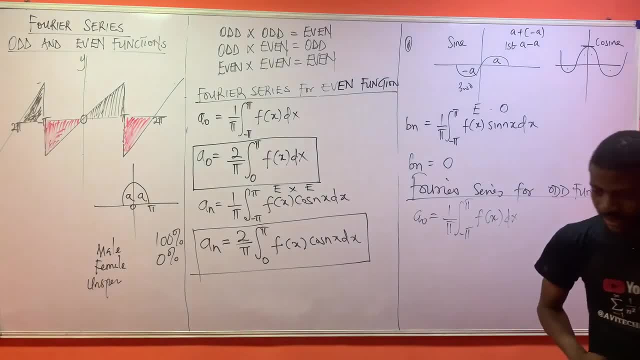 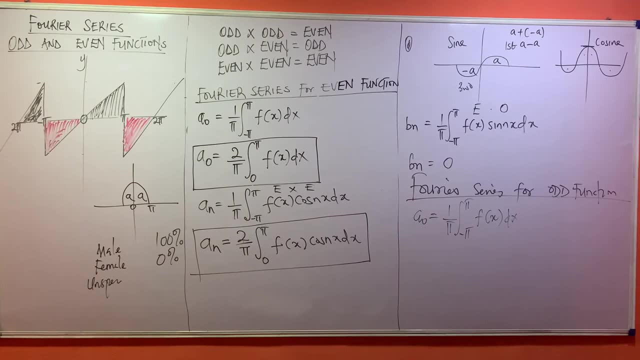 of f of s dx. Sorry, I think all of these guys, I would be getting a new marker. Let us see if this new one is going to perform much more better. Okay, Now see. so this is what we have for this very guy. 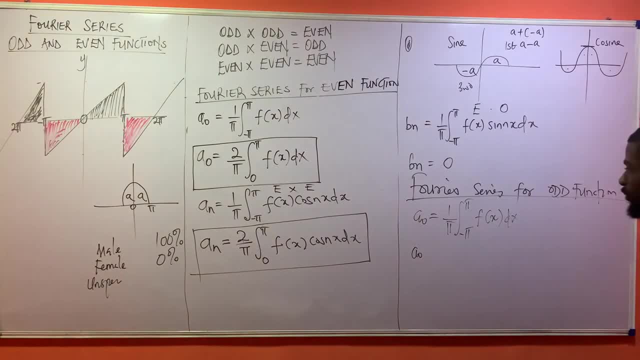 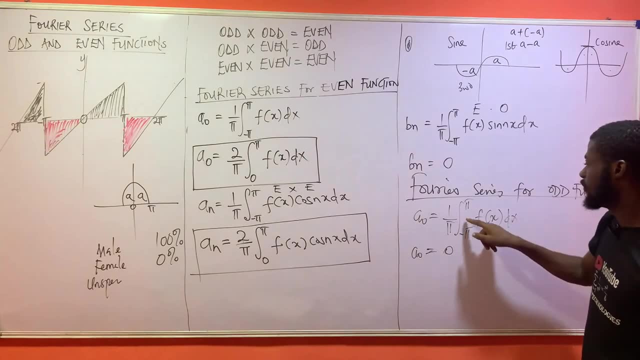 Now a naught. okay, better marker. very good, It's going to be zero. Why is it zero? We already said that the function is odd, If you want to integrate this very guy odd. This side is positive. this side is negative. 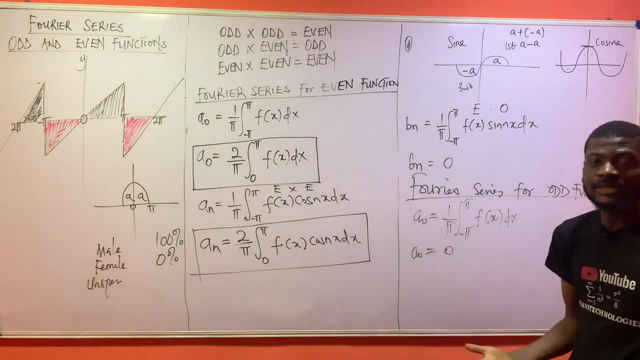 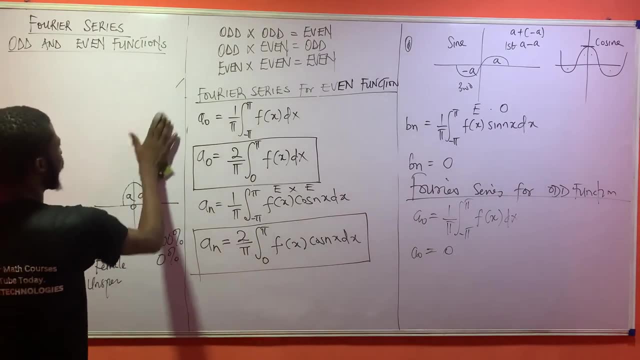 The areas we cancel will give you zero. So a naught is zero, Thank you. Now you will not work out, And you will not work out. and come to this side. Now, on this very side, we're going to be finding something. 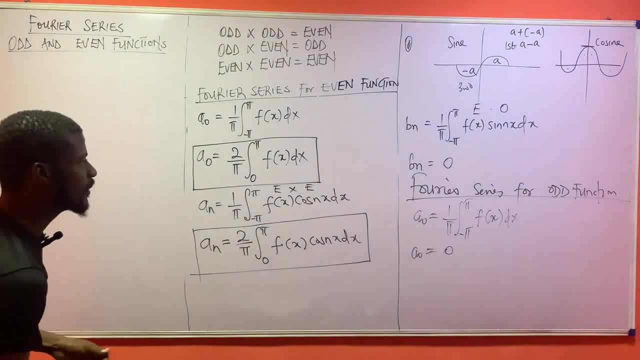 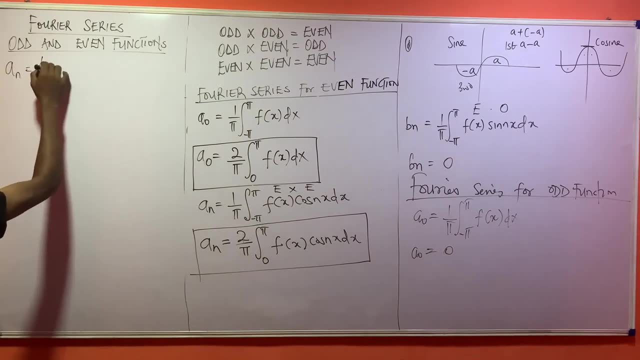 On this very side we're going to be finding something. Now see a sub n Formula: is what One over pi integral from minus pi to pi, f of s, cos, nx, dx. Now look at this carefully. We already said that the function 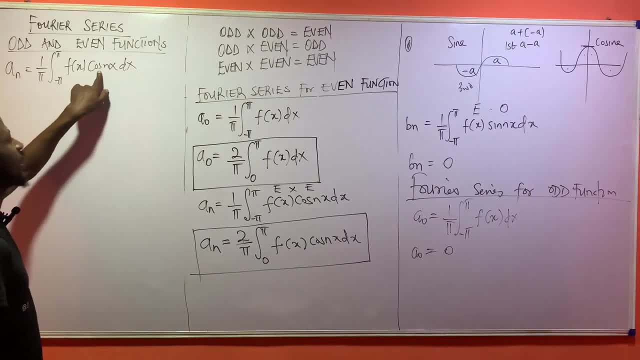 is odd, An odd function times an even function. what would that give to you? Odd times even will give you what Odd. So it means this guy is going to be an odd function. And if you should integrate an odd function over a symmetric, symmetric interval, 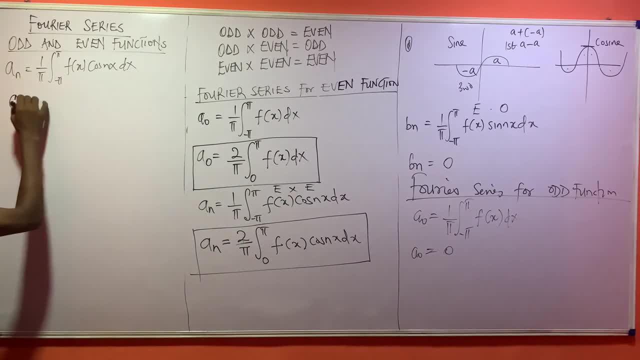 my result is what Zero, So a sub n is equal to what Zero. I've already explained it with this, The last guy. So let me be putting this guy in the bracket. Putting this guy in the bracket, OK. The last guy is b sub n. 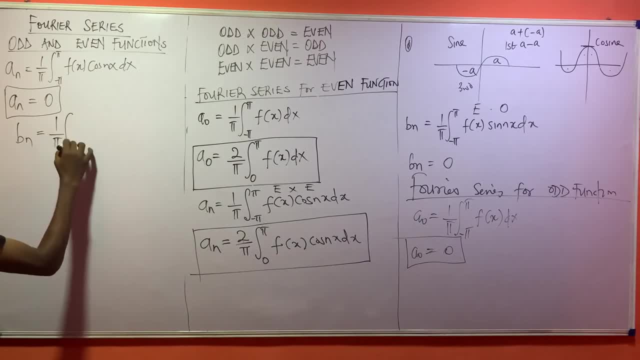 b sub n is one over pi, integral from minus pi to pi f of s, sin, nx, dx. Now what happens here? The function is odd. We already said it: The function is an odd function. Now this very function is odd. 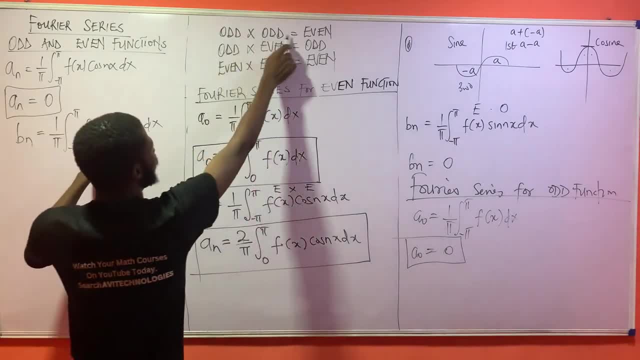 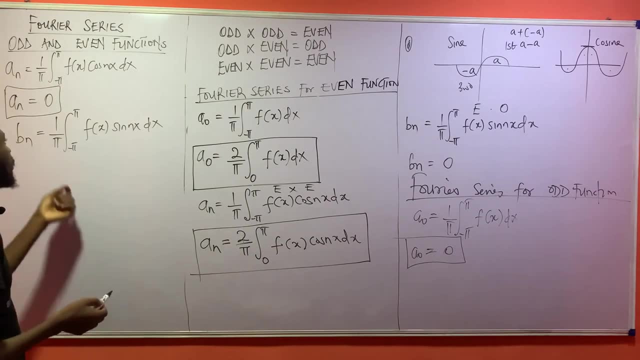 Sine is also odd, So odd times odd will give us an even function, And this way it gets very beautiful. If you want to integrate an even function, what you simply do is to reduce the interval and double your result. I've already explained it using that guy that I've claimed. 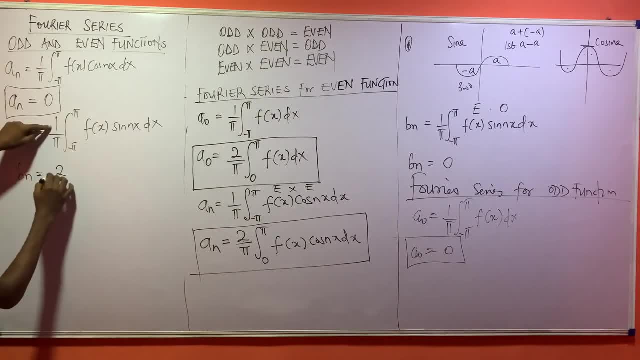 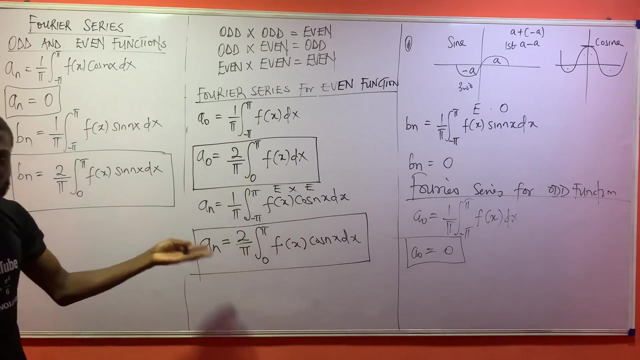 So right now, this will become b sub n equal 2 over pi integral from. I want to do this again. I will say: this is zero to pi, Then f of s, sin, nx, dx. Now, as you can see, this is not just telling us that. 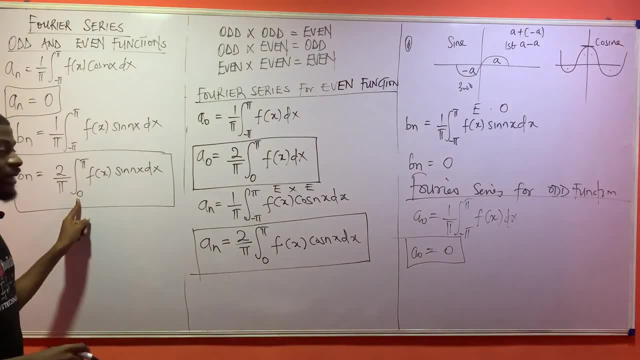 oh, you can reduce this integral. It is also telling you that, provided you know the function is odd, the only thing you need to come and find is b sub n. It is not beautiful. So if you just know, oh, the function is odd. 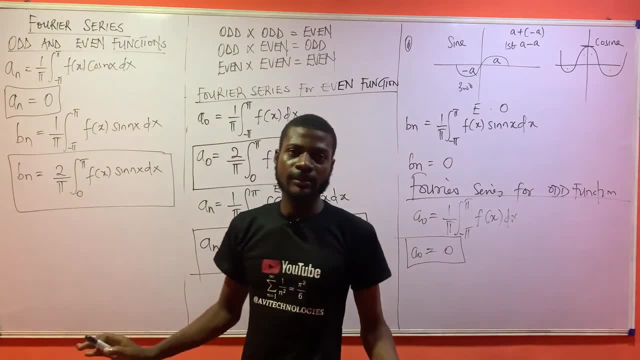 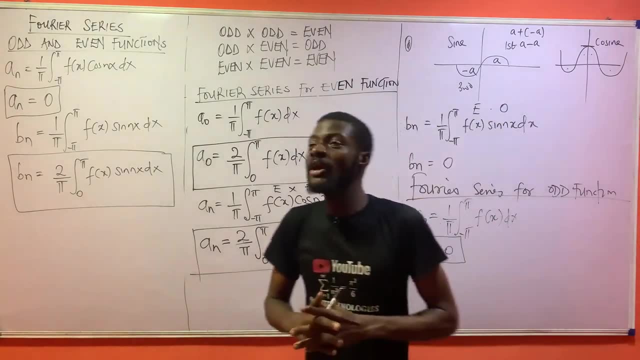 what would I do? Just come and find b sub n, Because you already know the function is what Odd? So this is why we need the odd function. OK, Odd and even function. Now what if the function is neither even nor odd? 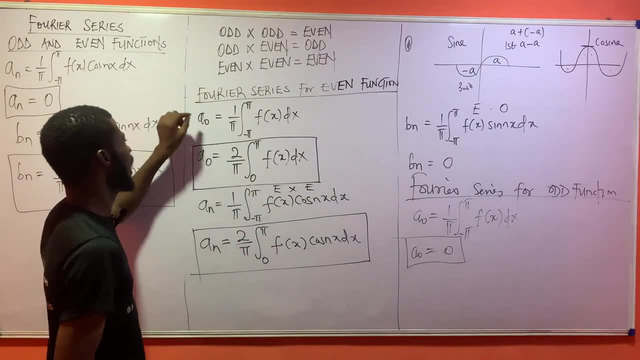 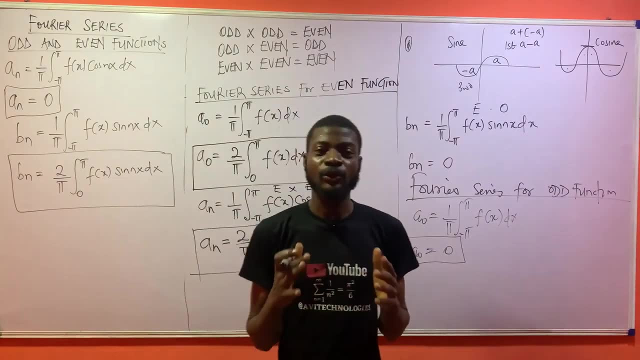 My dear, you will find everything. Like with the way they are. you will find everything. It's neither odd nor even Now. with these few points of mind, I hope I've been able to convince you to subscribe to this channel. 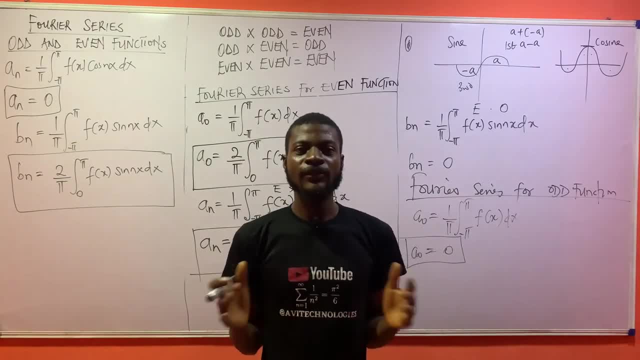 and share this very video to your classmates. Thank you very much for watching. See you next time.